That we have to count. And likewise, if we make it even smaller, we've created another surface to measure. So we are increasing surface area the smaller and smaller that we make these particles. So in the same volume, in other words, if we had a jar filled exactly. 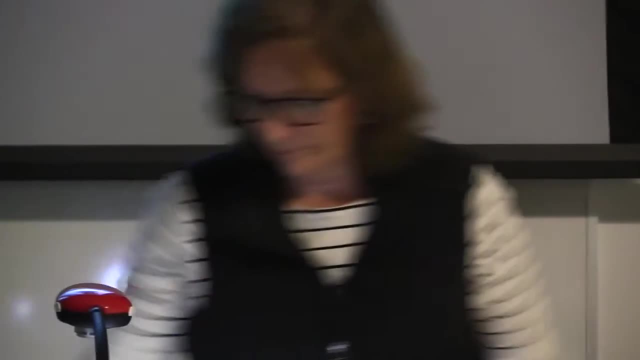 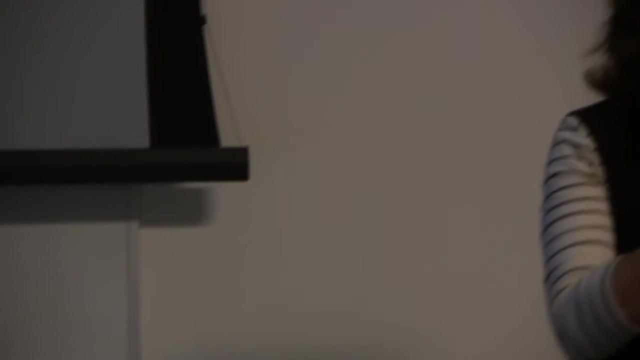 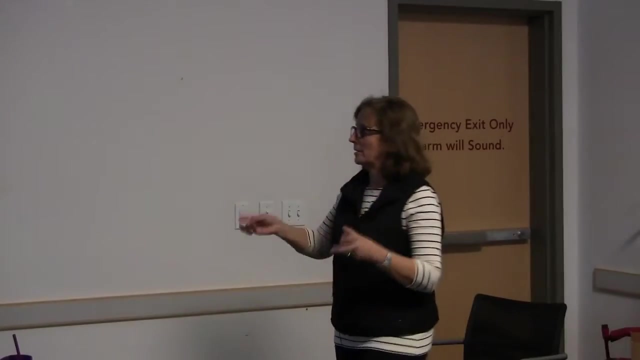 the same we would. Let's see, if I can, These guys will show up under there. Yeah, maybe You know we've got surface area in that, but if we were to cut those golf balls in half, we were adding surfaces Likewise a quarter, et cetera, et cetera. So the smaller. we get, the more surface area develops. Those surfaces is where water clings and minerals cling. So the more surface area you have, the more added surface area you're going to have, The more active typically the soil is chemically, but also you've got more potential for water. 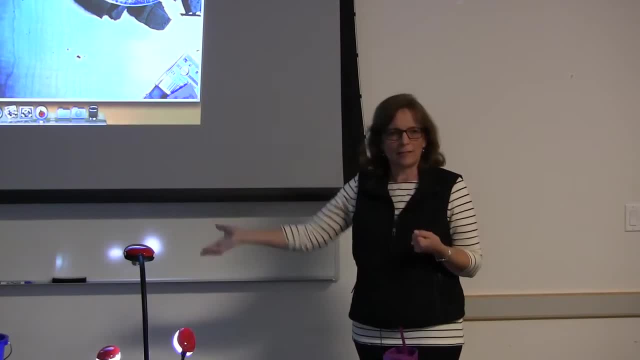 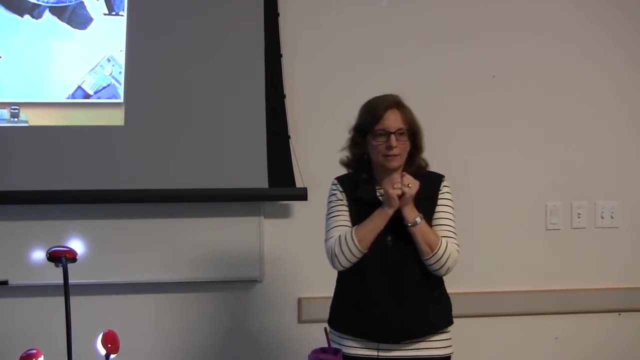 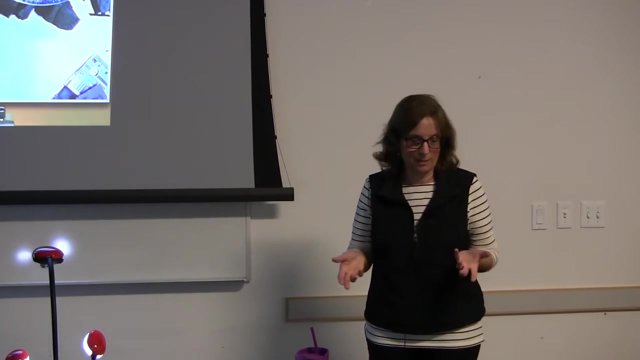 holding capacity. So when we say the clay soils are wet, slowly draining, et cetera, it's because of those surfaces They're holding on to that water. Sandy soils, the golf balls you could imagine, are much more well-drained because of those big pore spaces. Yes, they're. 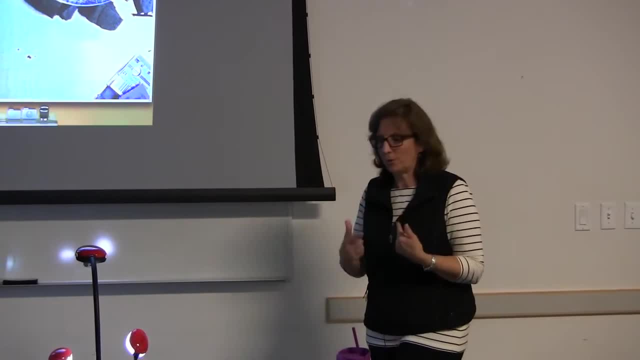 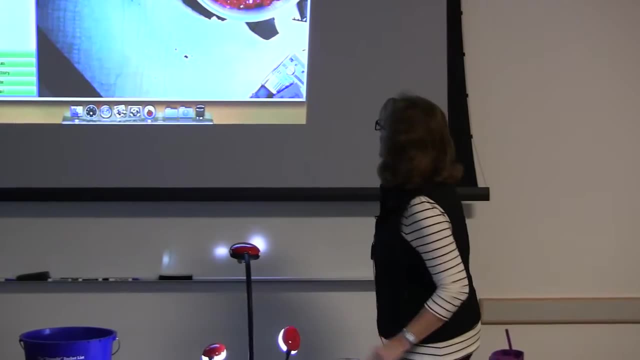 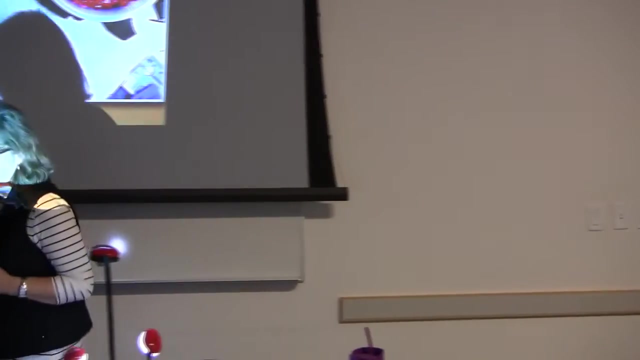 larger particles, but when you add up all the surfaces in that area, they're not that big, And so we've got the sort of medium-sized particles. Those are the little red beads you may not have been able to see from the back, And then we have these little tiny sea. 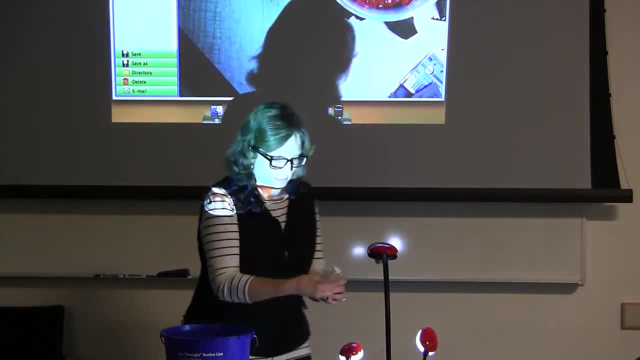 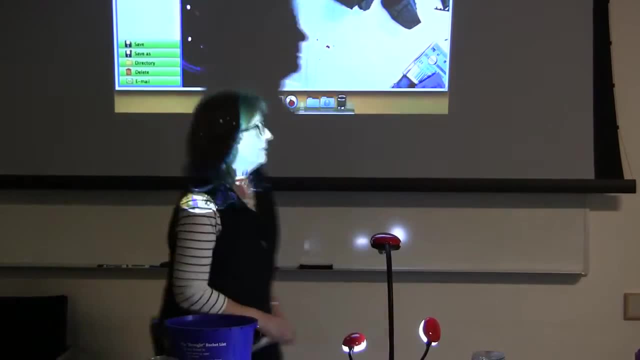 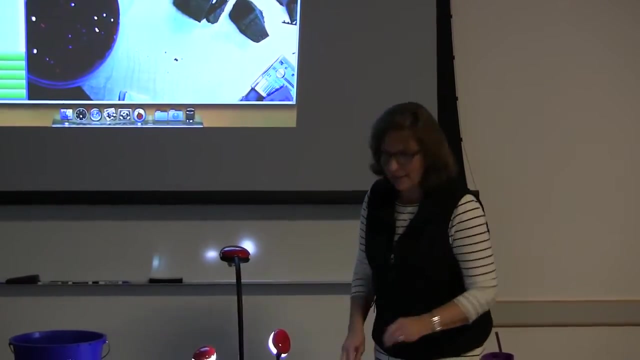 beads. You can put it on here one of these days And hopefully you can get an idea what those are like in comparison. Now, one of the other things that's kind of fun is that I doubt anybody here brought 100% sand for their soil. Pretty close. Anybody think they have 100% clay. That's possible, But typically your soil is going to be a mixture of the three particle categories, And so oftentimes what I'll do is I'll say OK if we have sand with very large pore spaces. that's one thing. 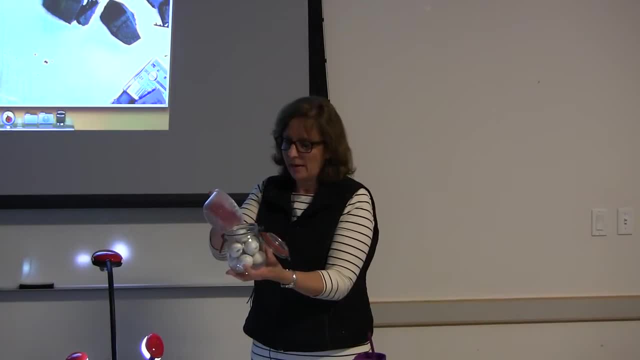 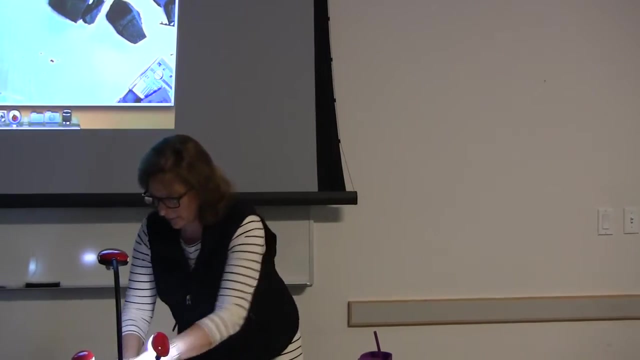 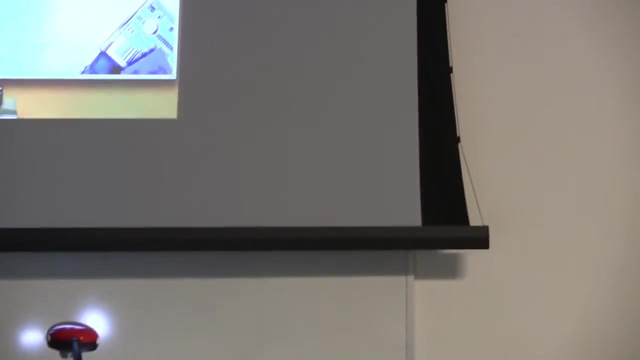 the beach or a playground or whatever. But we can actually add these silt-sized particles and begin to fill up the spaces here in this soil, And now we have created a soil that has both macro pores And sort of medium-sized pores in it. 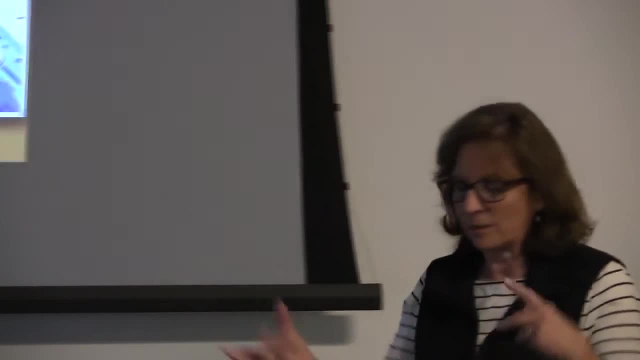 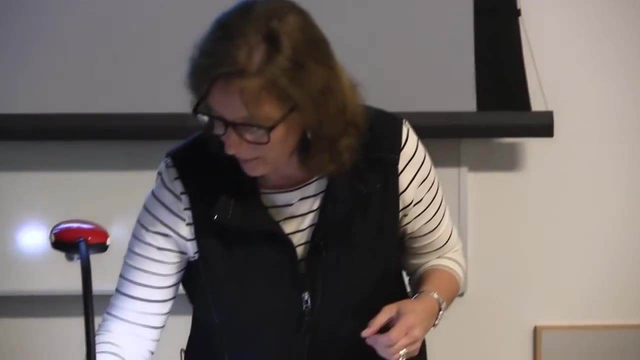 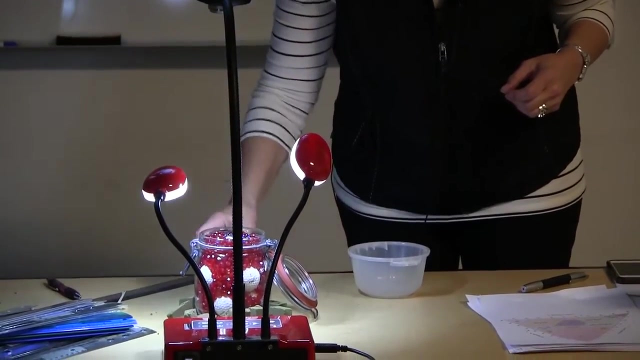 So we've got some macro and some micro pores going on there, And that's probably what's happening in your soils is that it's a mixture of all three, And we can even add in these sea beads and fill in all the little spots in between. 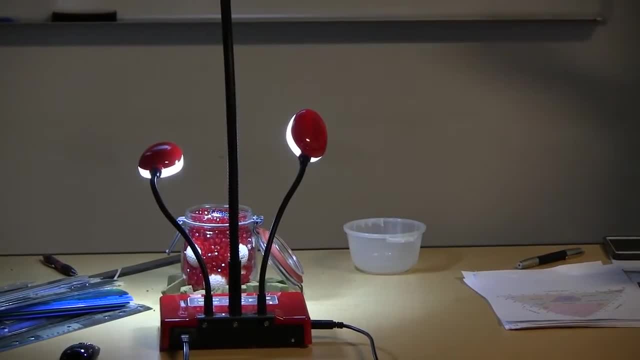 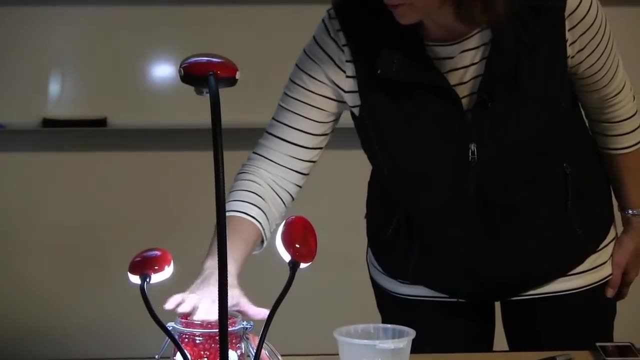 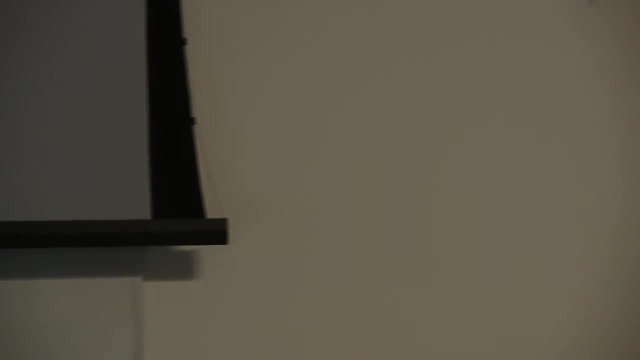 And then, you know, sift down eventually in there and fill up all the little spaces in between these red beads, And so we even have much smaller micro pores. OK, So typically we have a little bit of sand, silt and clay in our samples. 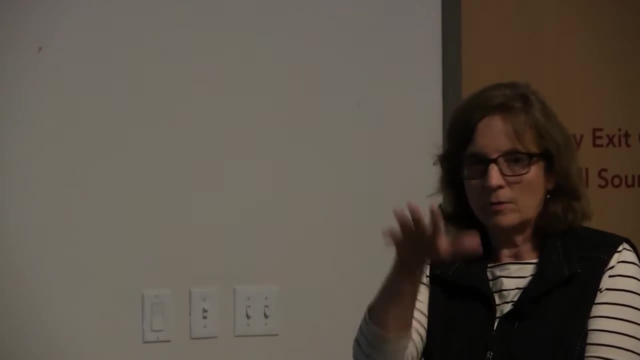 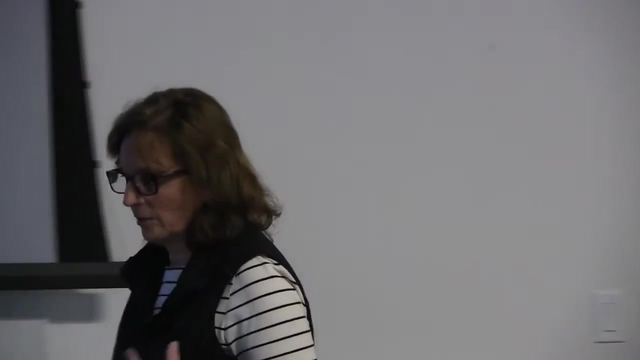 Though I will say, sometimes I've seen just sand and clay, very little silt. So if you don't have all three layers, don't despair, It's just. you know, silt is more something that's wind-driven or carried by water or something like that. 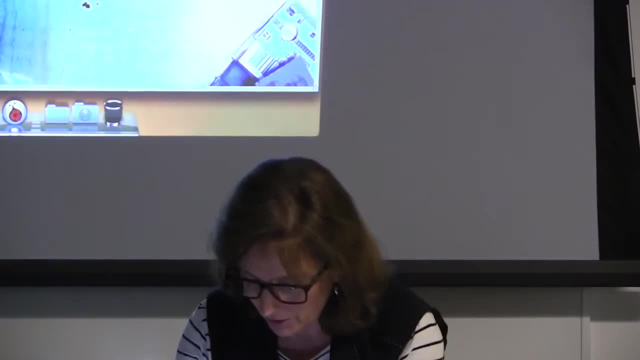 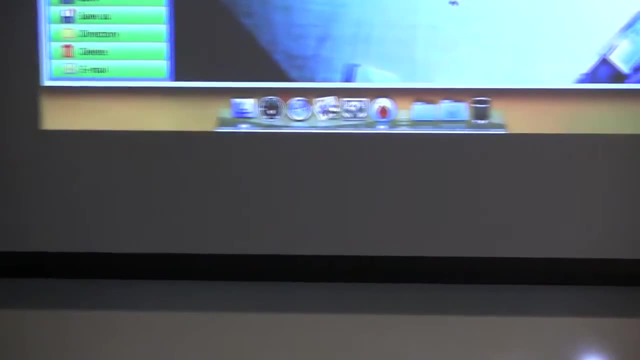 So you may not have natural silt-sized particles in your area. The idea, though, is to figure out what you have and then what influence it's going to have on your practices, And then what can you do about it. All right, 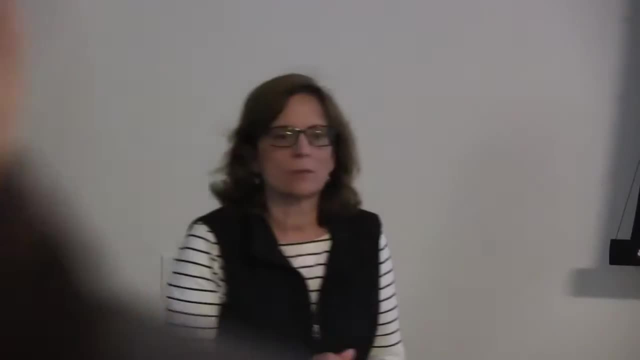 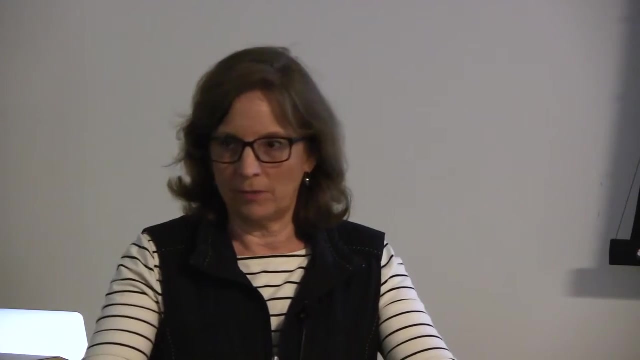 So we talk about these as soil separates, Because what you did in your jar analysis is you separated your soil particles right. So you put your soil in the jar with water and maybe some Calgon. I'm not sure if you guys got a chance to use that or not. 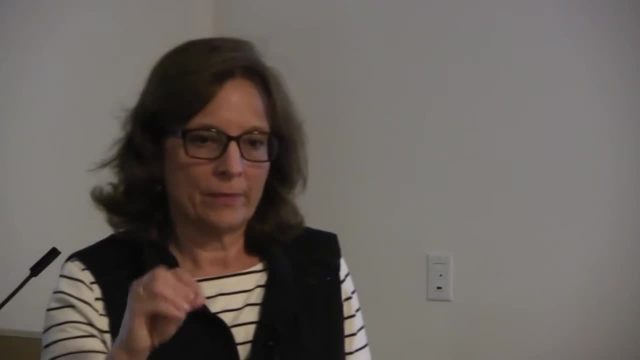 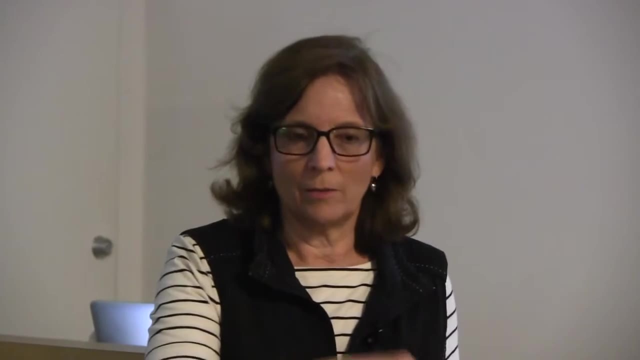 Sometimes you can use either dishwashing liquid or what we call Calgon, the water softener, to that, And that's a deflocculating agent You don't want to use like Dawn, You want to use more like Cascade that doesn't soak up or foam. 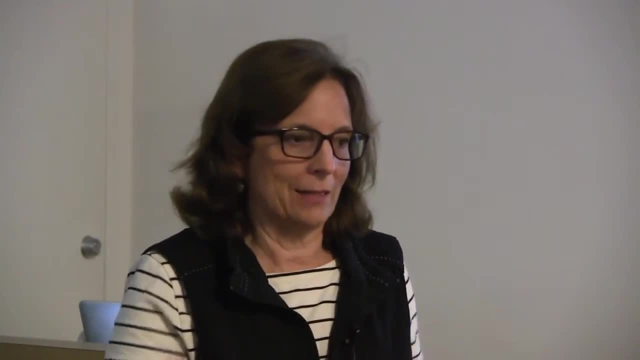 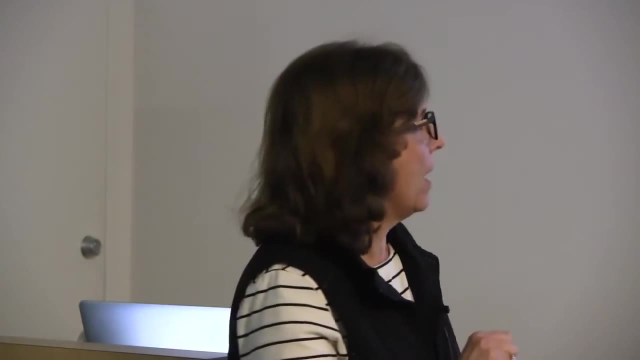 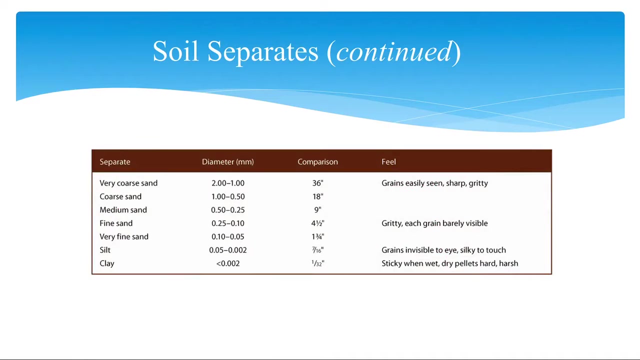 But you can put it in there, And that would just help break things apart more. But water is perfectly fine. Shake it up for a few minutes, five minutes hopefully, whatever- And then let it settle, And these separates then will begin to settle out. 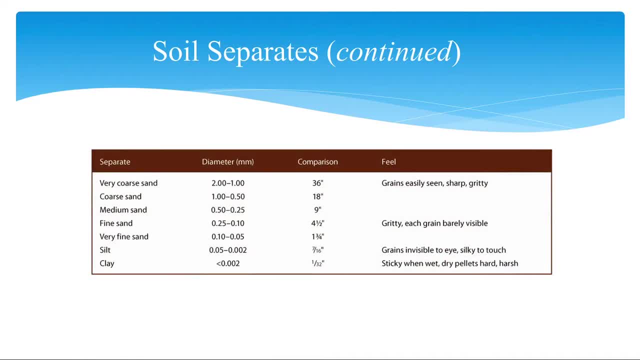 And some scientists actually categorized all the divisions of sand- the silt-sized particles and the clay-sized particles, And they determined that within, I think, 40 seconds, all of the sand-sized particles fall down. So there's a mathematical equation that you can do that. 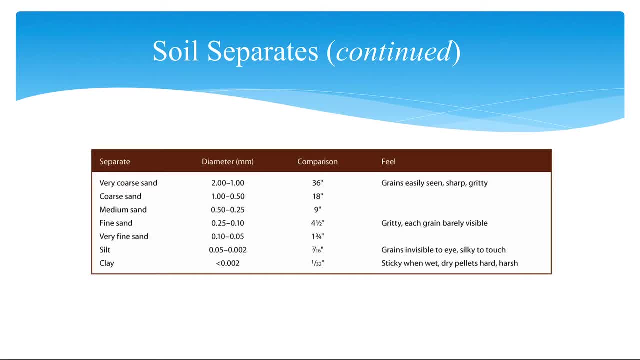 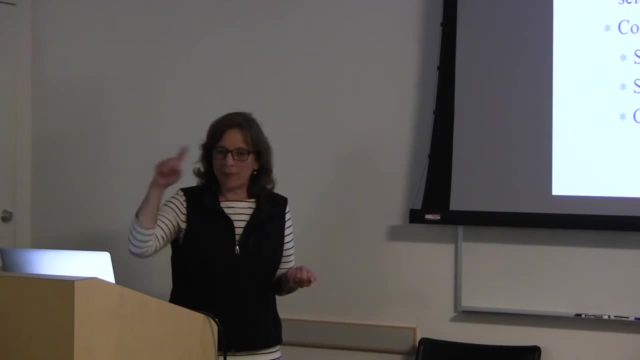 Within 30 minutes, all of the silt-sized particles come down, And then anywhere from 24 hours to two weeks or more a year, the clay-sized particles will settle down Now. most of the time your organic matter will remain floating. 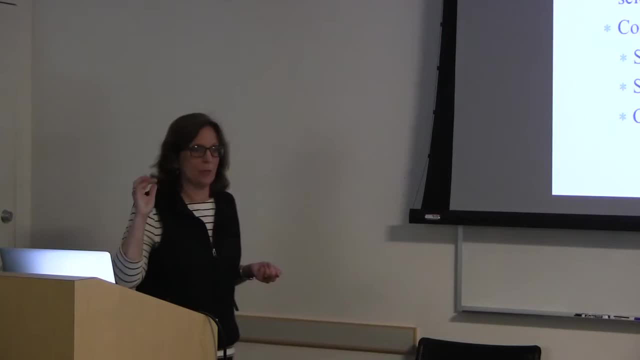 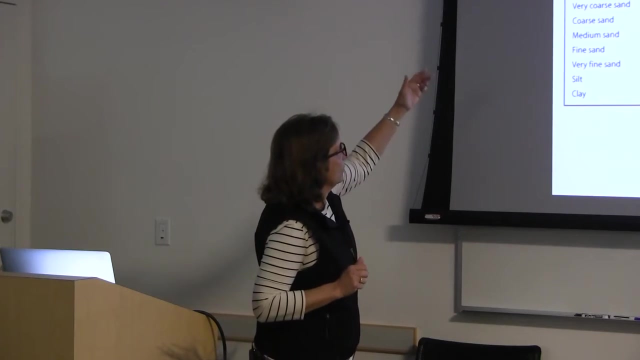 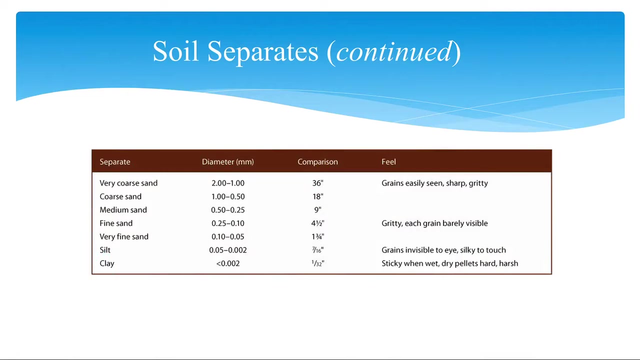 And also your clay sometimes remains floating in the water because of the negative charges that they have. It's just a kind of electrochemical reaction that they do. But just to give you an idea What these look like. again, when we talk about sand soil, scientists go anywhere from very fine sand to very coarse sand. 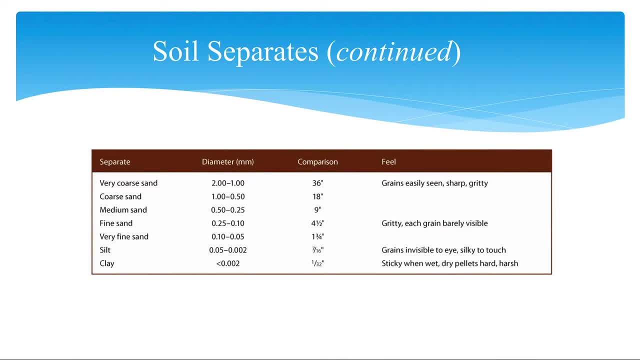 It can be anywhere. In other words, rock or gravel is anything over 2 millimeters in diameter, But if it's anywhere between .05 and 2 millimeters, that is considered sand. So if you were to compare it to objects, 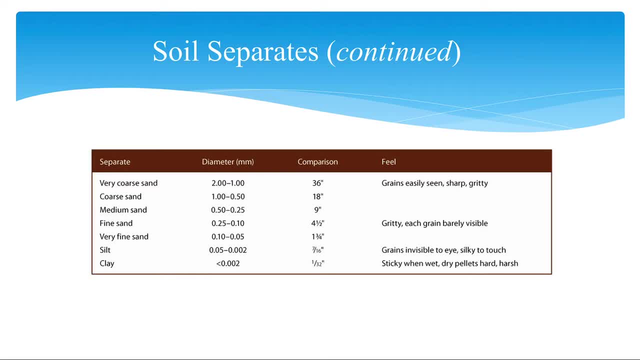 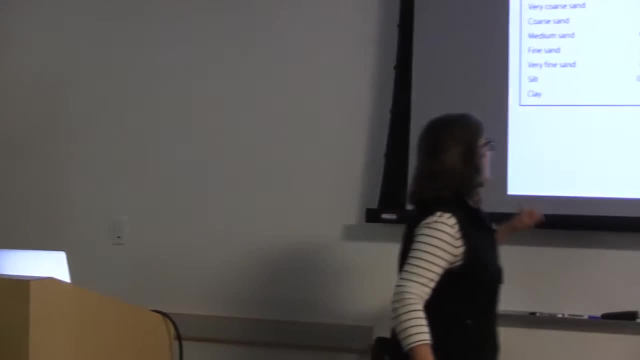 The very coarse sand would be 36 inches in diameter, But it could also be as small as 1 and 3 quarter inches and still be considered a type of sand-sized particle. But they're still big. They're much bigger than these guys. the silt: .05 to .002 millimeters. 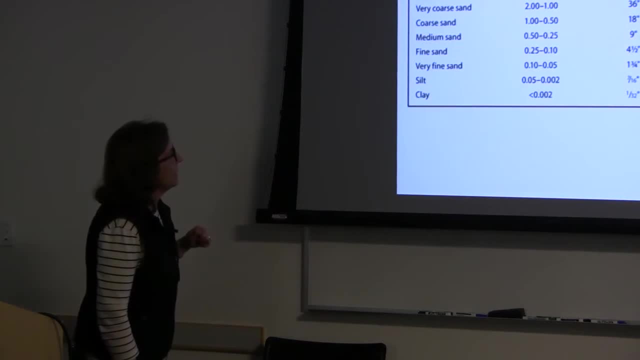 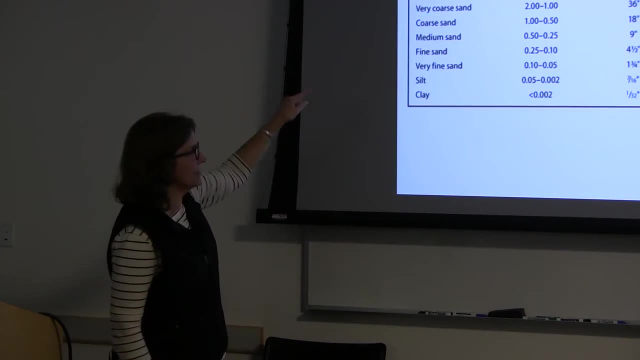 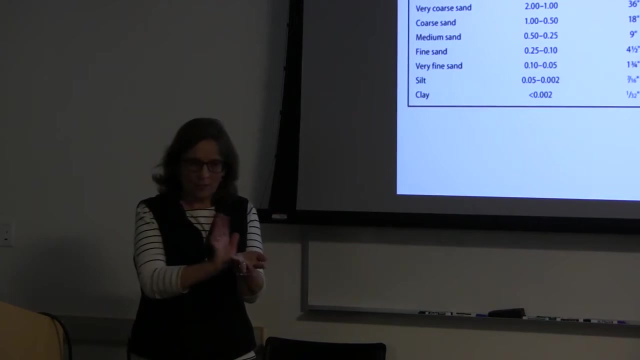 And then anything less than .002 millimeters is considered to be clay. Now you can easily see these very coarse sand grains And you may even be able to see that first layer that dropped And it's probably still settled there. How you know gritty looking it is and particulate. 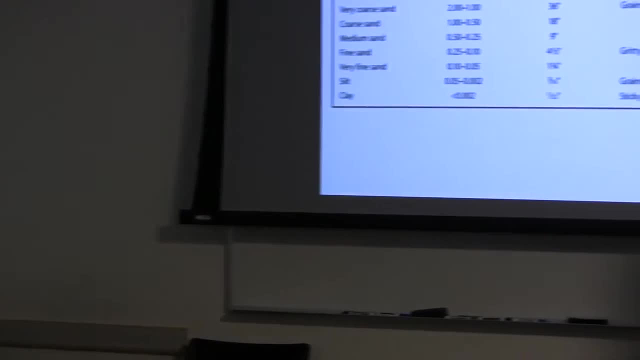 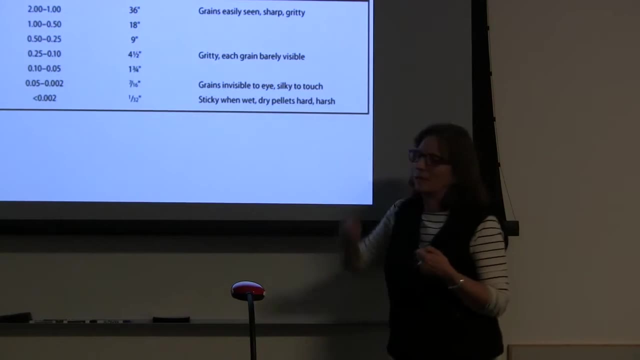 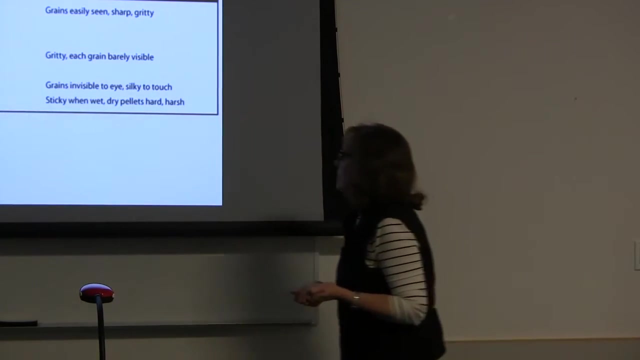 But when you get to the silt-sized particles, the grains are actually becoming invisible to the eye And they're very silky to the touch And it could almost be like flour. We know that there's individual flour particles in there, But you really can't see them very much. 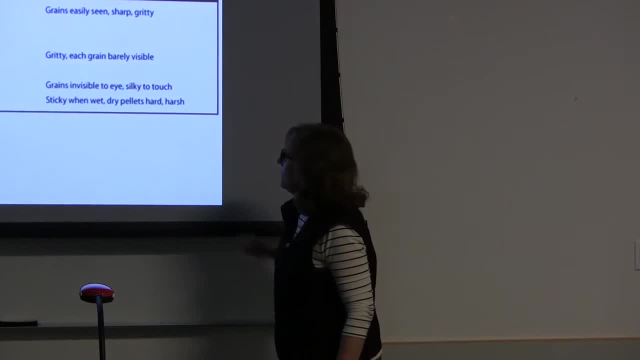 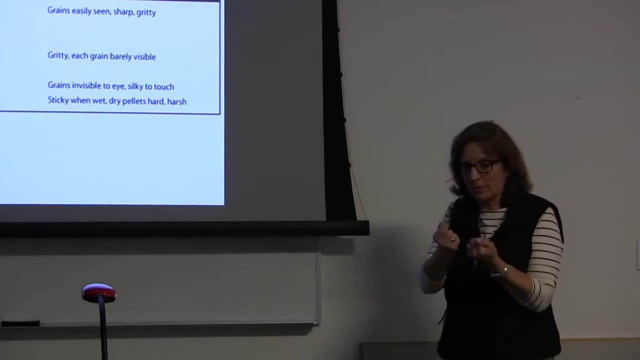 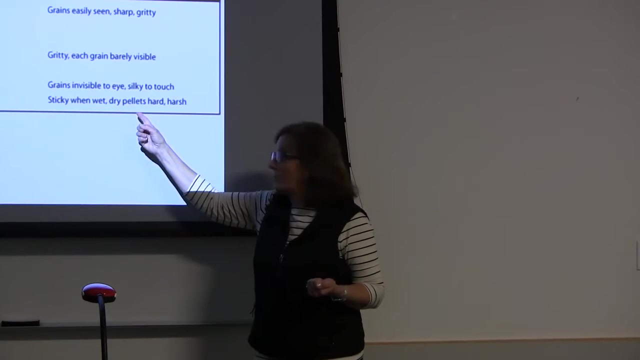 And so it feels silky like that as well. Clay is very sticky when wet. Again, these very small particles, Because they have those surface areas that hold on to water. when we wet them, typically they're going to be sticky, But boy, when they're dry they're hard as a rock, almost. 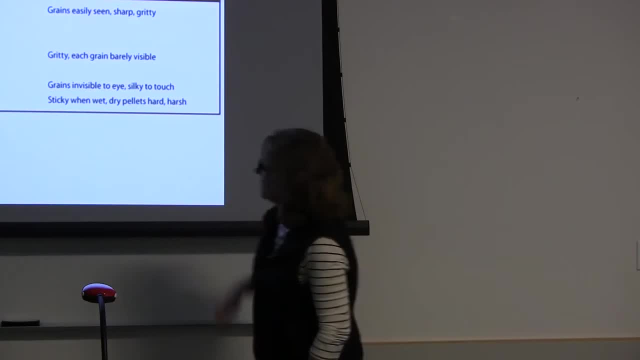 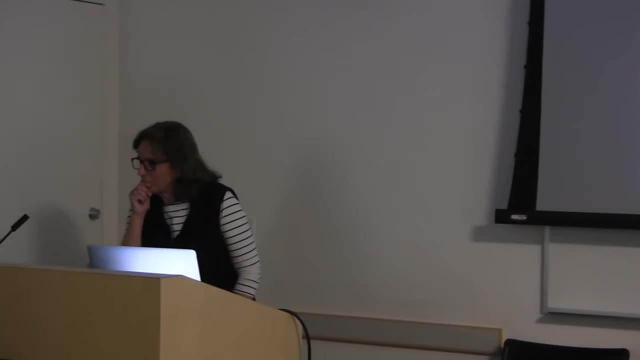 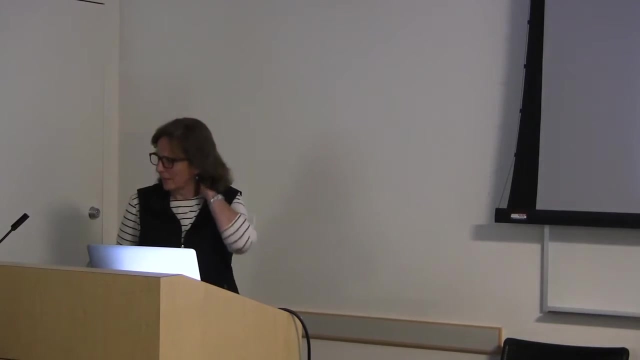 And I'm not sure what harsh meant. But anyway, I think in the book clay soil is described as harsh soil. Okay, Because of its chemical, I don't know. That's how it says there. Even though it's called fine texture, it's called a harsh soil. 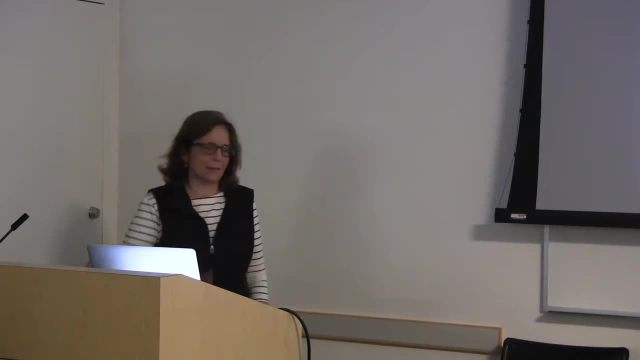 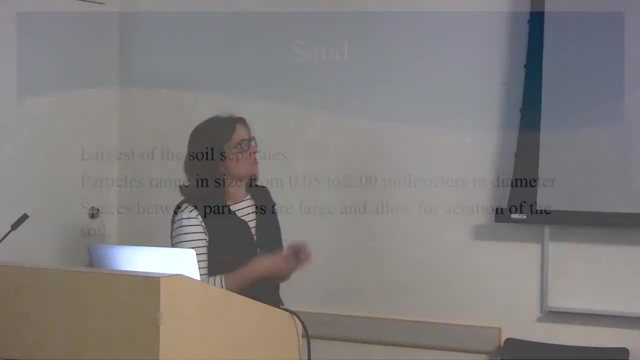 I just picked that up last night. Oh, interesting. Okay, From the book. Is that the same definition of harsh? That is a weird word to use for that. So again, sand is the largest. Okay, It's the largest. 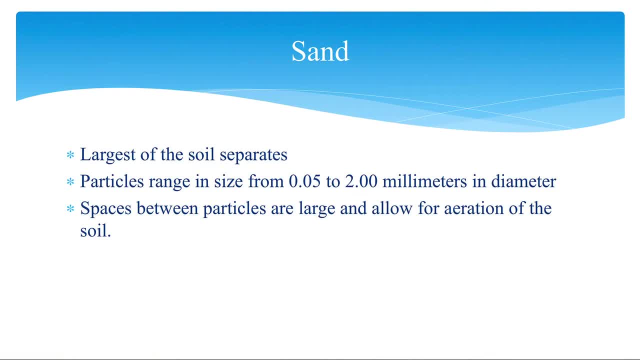 It's a very large. It's like a basketball, golf ball, whatever, And again, the size range that they have And the spaces between them are very large, Just like our golf balls had big spaces. Or if you had a bushel basket full of tennis balls or basketballs or soccer balls or whatever. 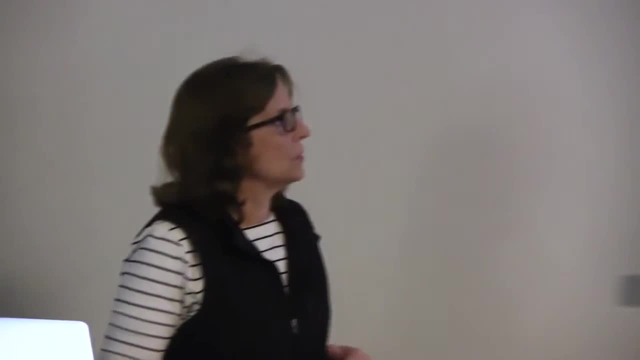 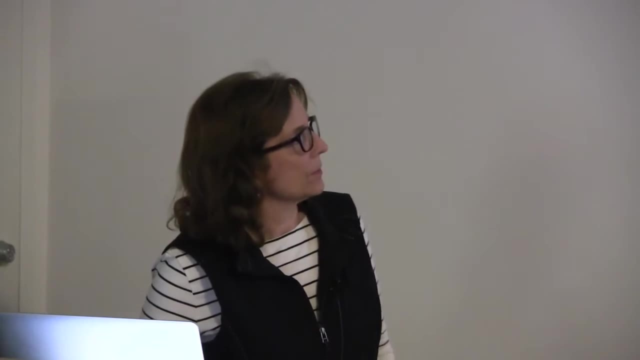 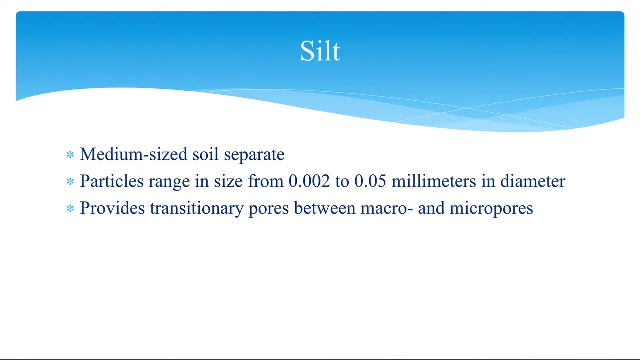 Big particles, big spaces in between, And that's going to allow for lots of oxygen and aeration And very little water. holding, compared to the others, Is silt, the medium sized one, The medium sized ones, so to speak. Again, the strict measurement, definition of those. 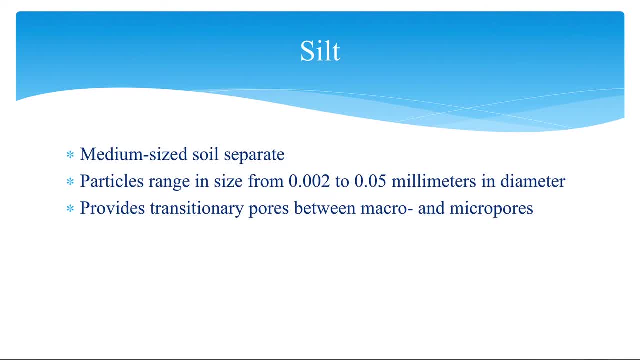 And they're a transition between the macro and the micro pores, So they're the medium, so to speak. And then when we talk about clay- and I've kind of changed my little thing here to water droplets because they're the smallest- 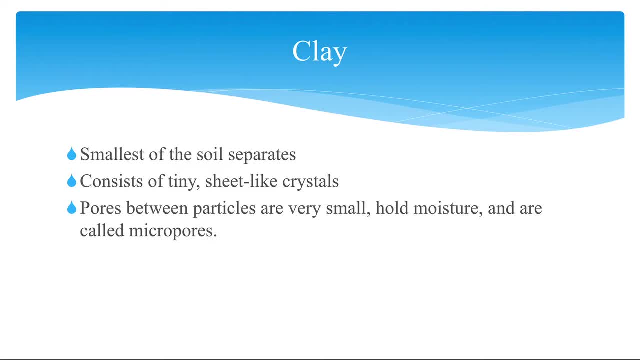 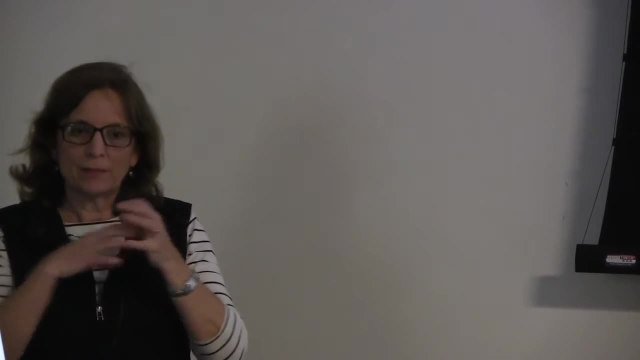 Oftentimes they're actually crystal formations. interestingly enough, You can see that sometimes with the right types of magnets, Magnification, The pores between them are very small, They hold moisture- And these are referred to as micro pores- And sometimes, within that crystalline structure, sometimes water gets in there as well. 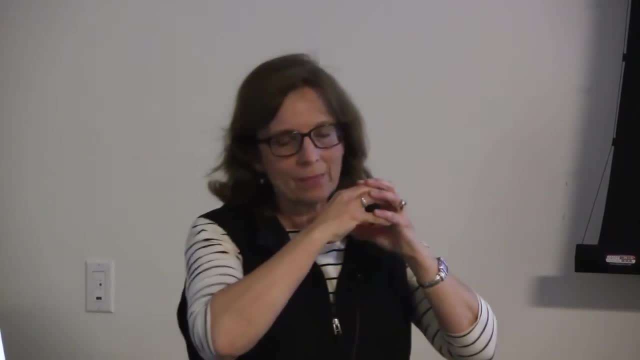 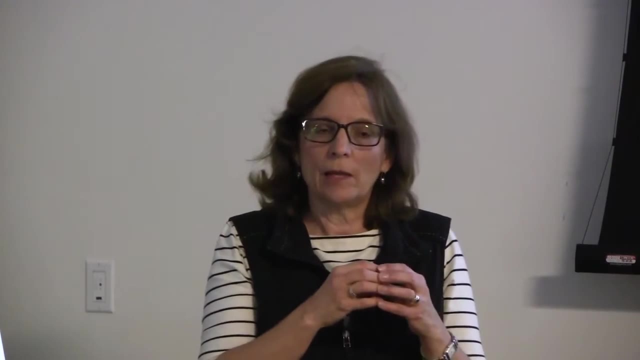 And it can cause the crystals to swell. Not that you'd see this at all. It's still invisible to our eyes and to a lot of microscopes. But if you think of and you may have seen, like when clay gets dry, you have those big cracks and crevices. That's when it's shrinking. So when it's dry it shrinks, And then when it gets wet it swells back up. Guess what that does to your foundation? Ooh, You know, the engineers want that foundation to be right next to your house and kind of holding it there the soil. 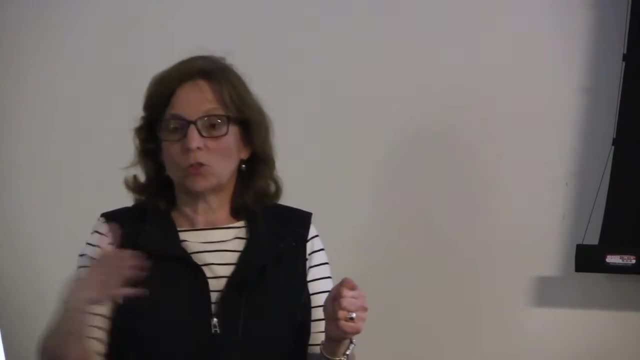 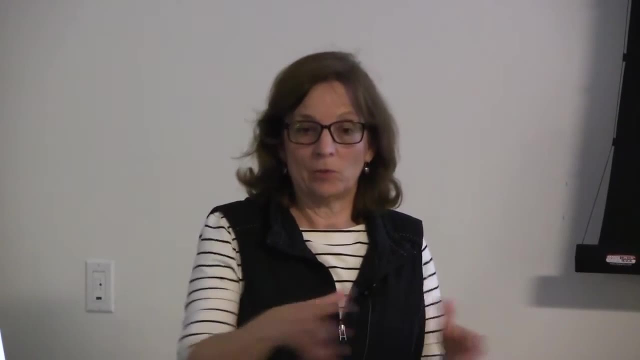 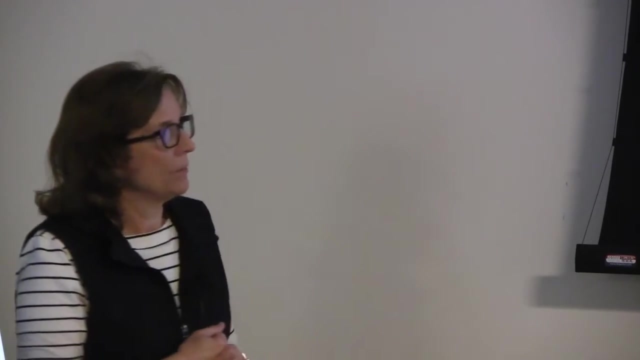 And so clay is actually really good. But when clay dries it shrinks away, And so every once in a while you may hear a call: go out. It's like water, your foundation. You know, keep it. So it doesn't shrink away and, you know, cause issues with cracks and settling and that sort of thing. 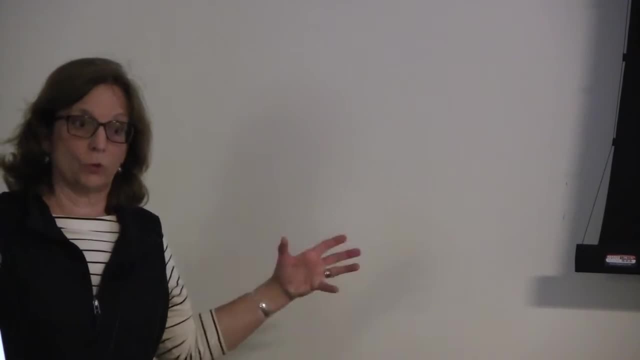 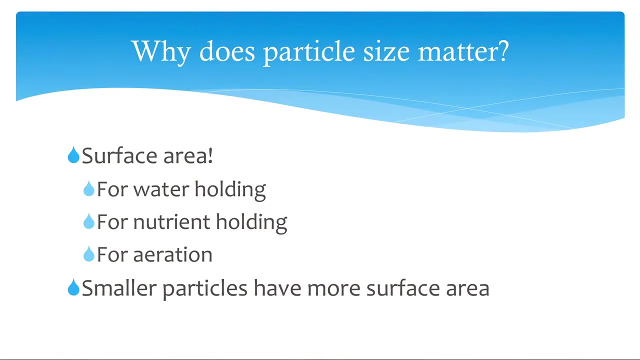 Because if we have a real long period of drought, that can happen where it will go away if you happen to have clay-based soils there, Okay, So why does particle size matter? Again, you probably don't need to memorize the size. you know definitions or anything like that. 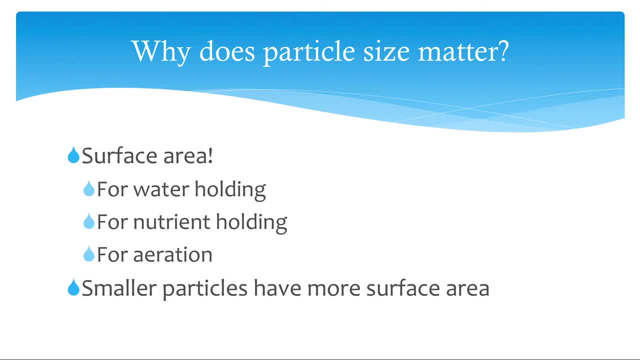 But you know small, medium and large Surface area. Again, as we demonstrated, It holds water, It holds nutrients And it also determines how aerated something is going to be. So the smaller the particle, the more surface area you have for volume. 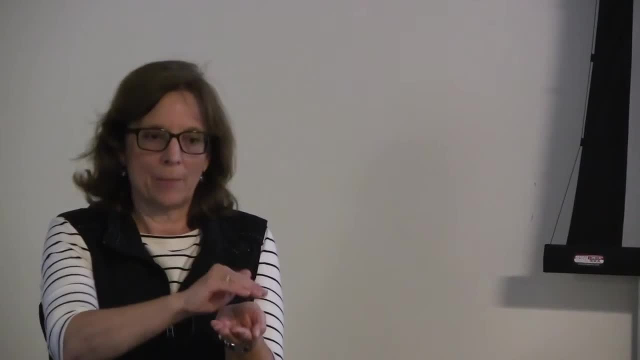 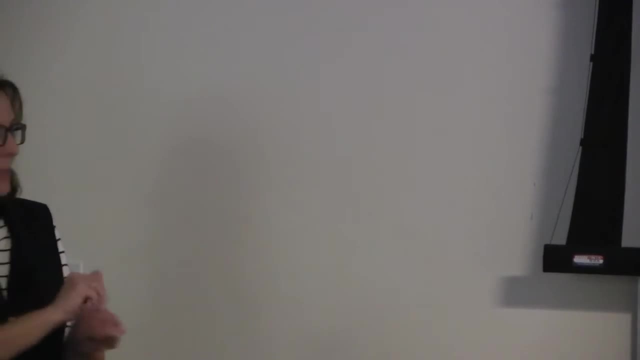 In other words, if we had a cup of those tiny beads, a cup of the medium-sized beads and a cup of golf balls, the surface area is going to be much higher in those cup of the tiny seed beads if you added up all those surfaces. 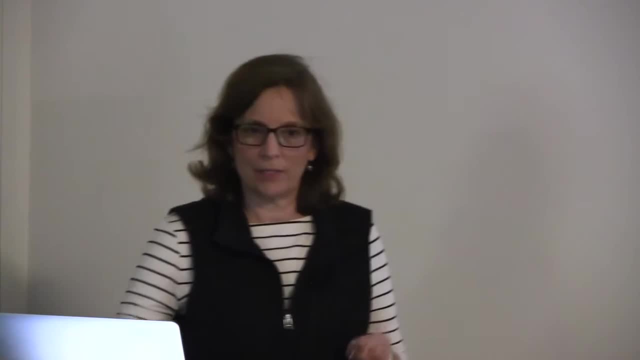 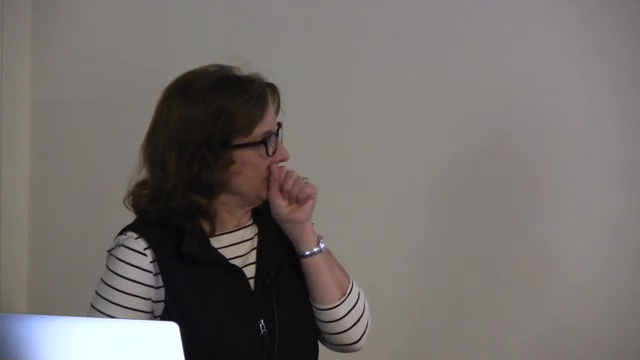 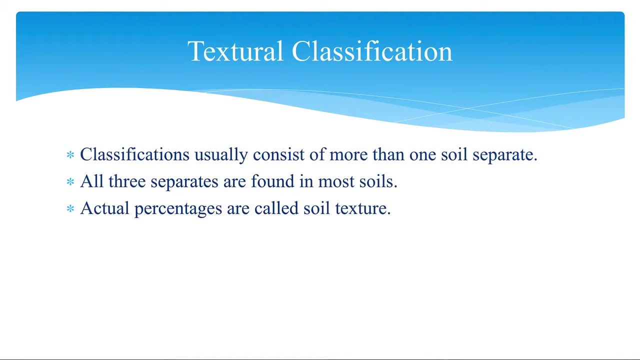 Okay, So it's going to cling to more water and it's going to have very tiny air spaces, So not a lot of drainage. Now again, your texture classification is what you get from that soil texture triangle is consisting of usually all three of these separate sizes. 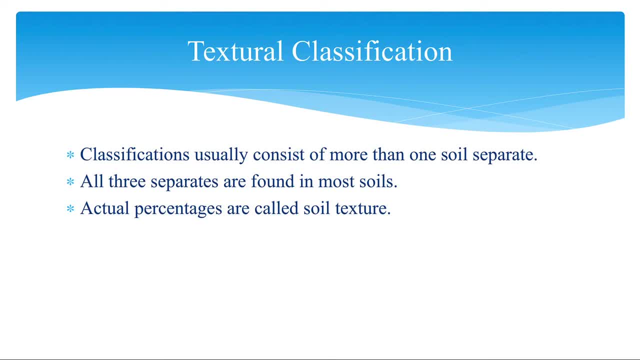 In other words sand, silt and clay, And it's the actual percentages. So when we use that term soil texture, we're actually figuring out what's the relative amount of sand to silt, to clay in your particular soil. 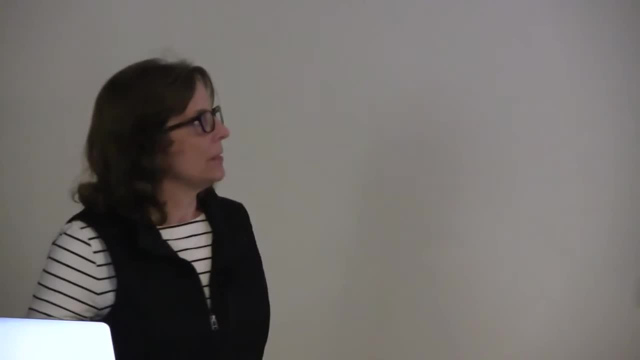 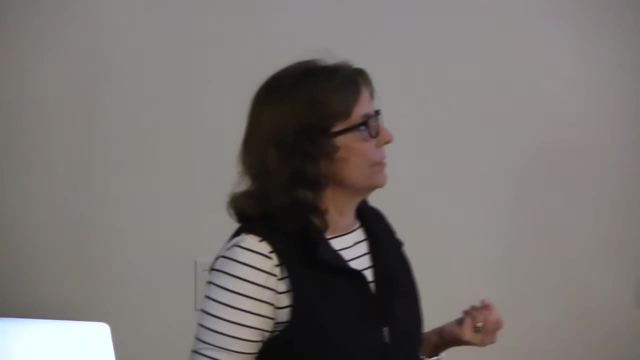 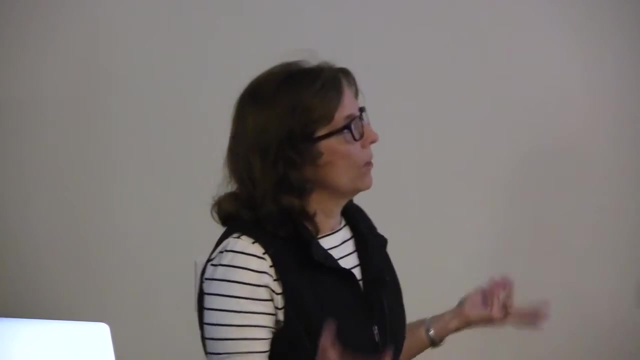 And that's our jar analysis there is going to help us determine that. So even within that triangle, we can refer to our soils as being predominantly coarse, predominantly fine textured or something in between. So if you have a very sticky clay soil, 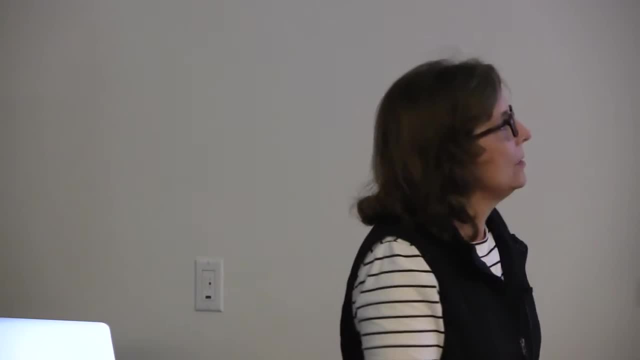 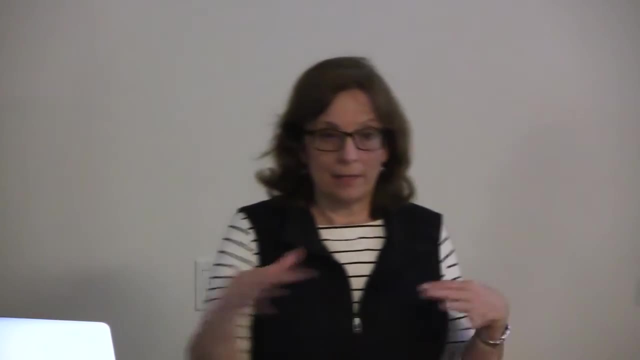 if it turns out you've got a high percentage of clay, you probably have what's called a fine soil. If you have a lot of sand in it, it's considered a coarse soil, And something in between is usually the happy medium. Because all of these things? 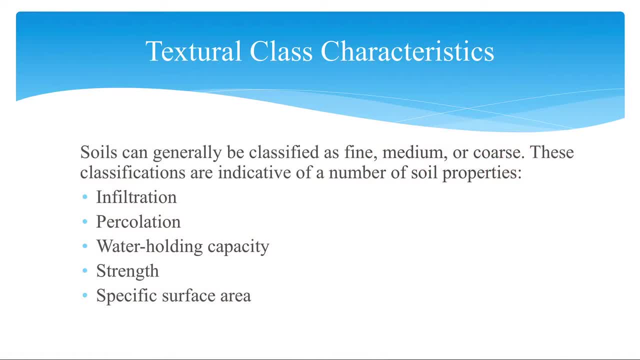 infiltration. in other words, how does water get into your soil? it's very tiny little holes. It's very difficult for water to get in that And it tends to just go over the surface and maybe even take the soil with it, Whereas if it landed on sand or some gravel or whatever, 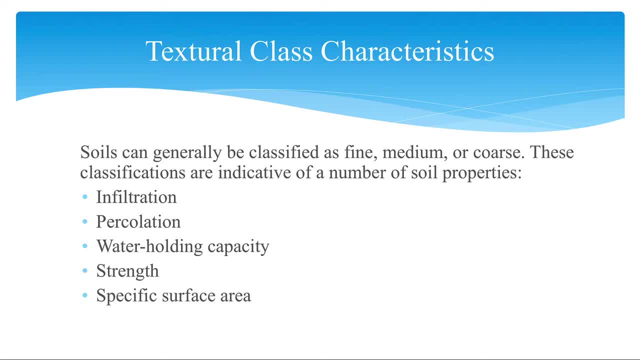 you could imagine the water percolating in at that point and infiltrating and then moving through the soil. So infiltration is the initial, Percolation, is what happens afterwards. And then how much does it hold on to that water? Maybe how strong it is? 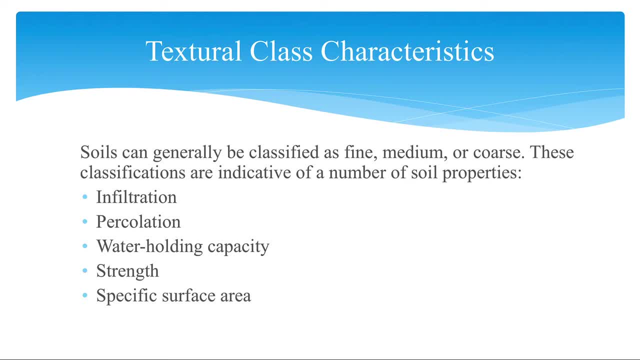 And if you have dry soil here with you in a bag and any clods of it, we're going to do a thing called dry clod breaking, And if it's really hard to break it apart, it usually has a high amount of clay. 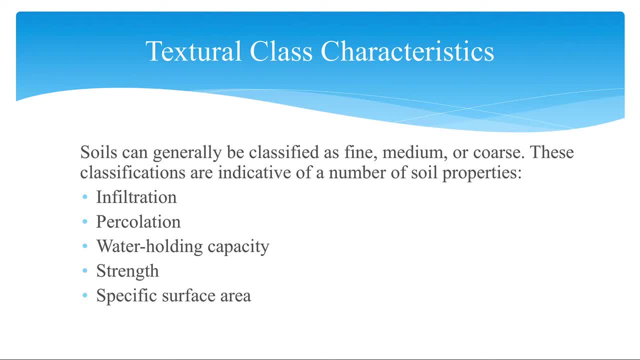 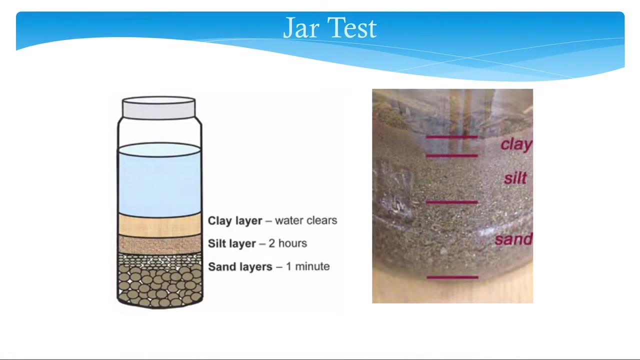 If it's real easy to crumble apart, it may have more of the sand. And then again your specific surface area and amount of surfaces that you have. So in your jar analysis, again, your sand layers, you know, and just as a ballpark figure, 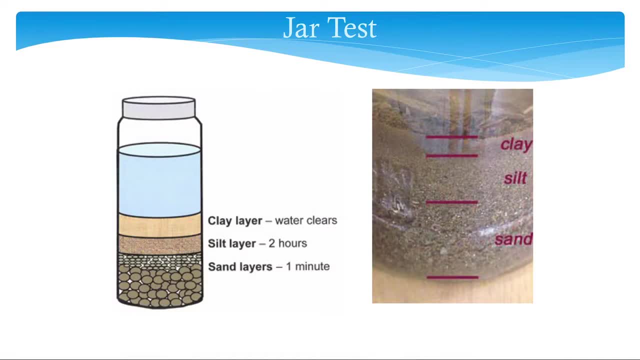 I gave you the 40 seconds. 30 minutes dah dah. dah you know 24 hours. Some other people just sort of break it down into something a little easier to remember. You know all your sand's going to drop in the first minute. 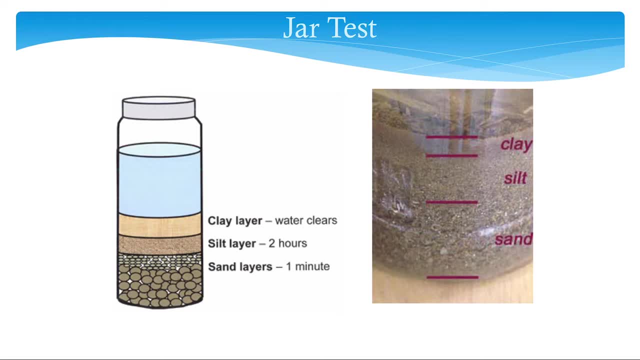 If you come back a couple hours later, you'll see probably the silt And then your clay. you know, go take a walk, come back next week, maybe your clay will have dropped down, And so if you're watching this, you can actually 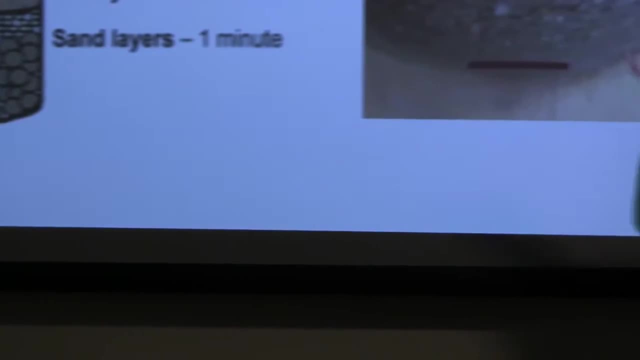 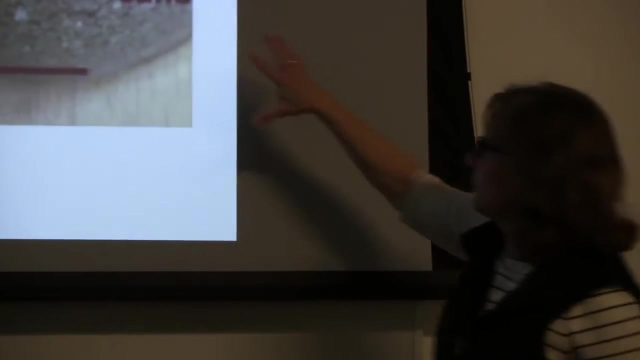 if it's not too cloudy, as it's coming down, and the cloudiness would be due to that, you can start marking on your jar where the actual layers are, And always those visible particles that drop fast And again, this is kind of showing. 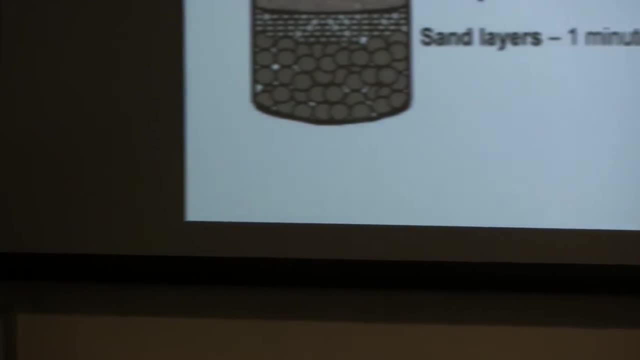 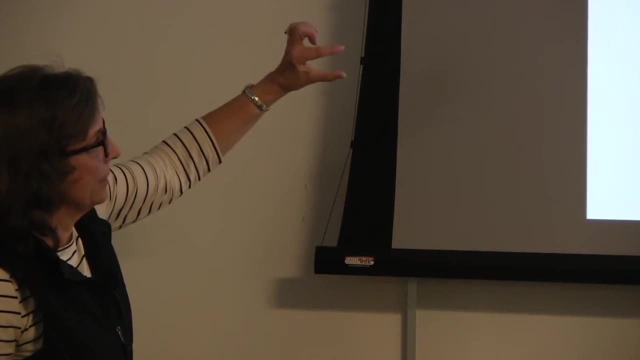 some of the different sizes of sand particles. You know it's not just one size, It can be up to four different sizes. That could be your sand layer And then your silt layer drops later And then the clay layer takes the longest. 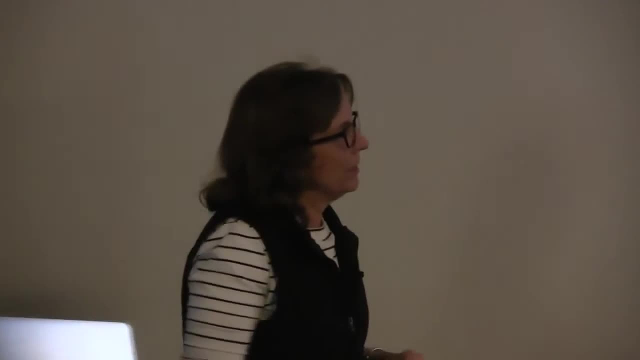 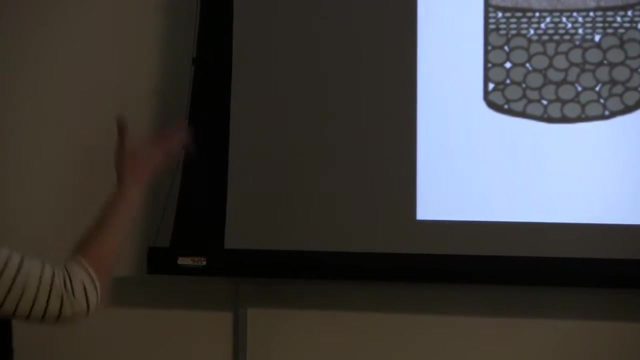 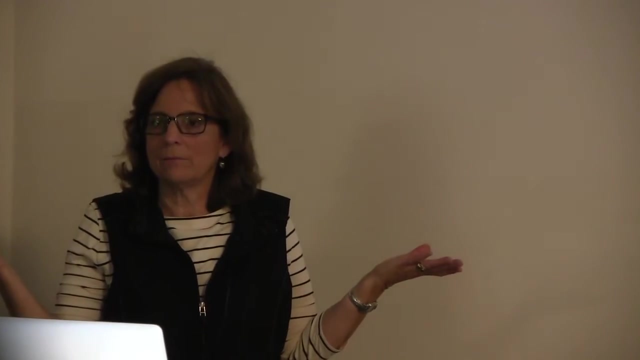 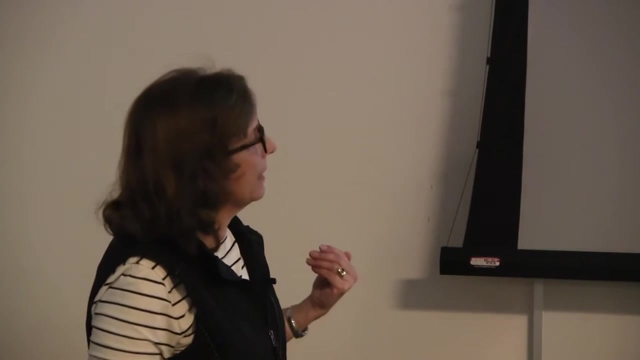 to come down When we measure these percentages compared to each other. if we were just to look at this, what would we think about this particular soil sample? It's predominantly sand, So we would think this is probably a pretty decent soil that looks like it's over 50% sand. 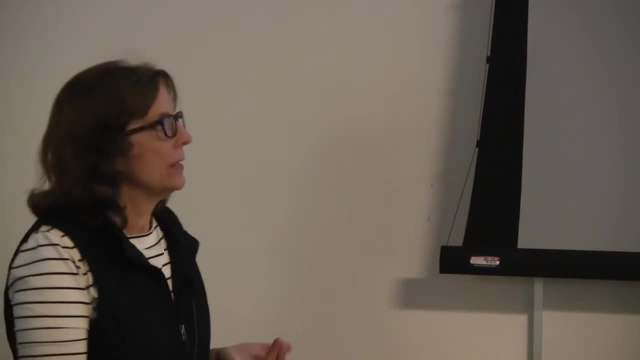 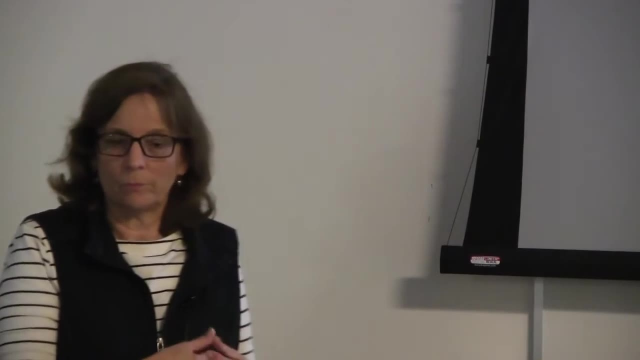 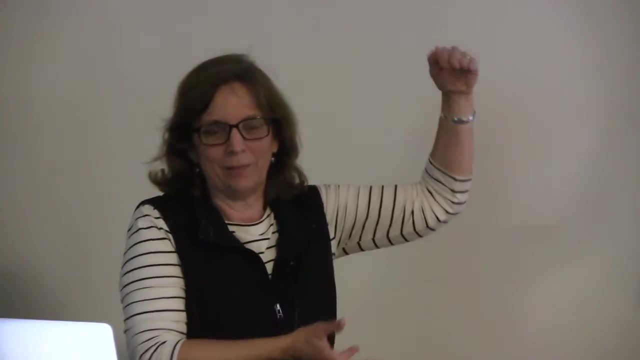 So we're going to have probably good aeration. We're going to have good water movement and percolation through it. So these are all pretty decent characteristics about a soil. When it's the opposite, if that was the clay, that was 50%. 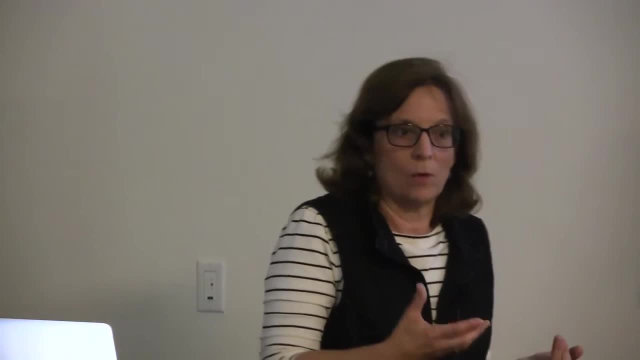 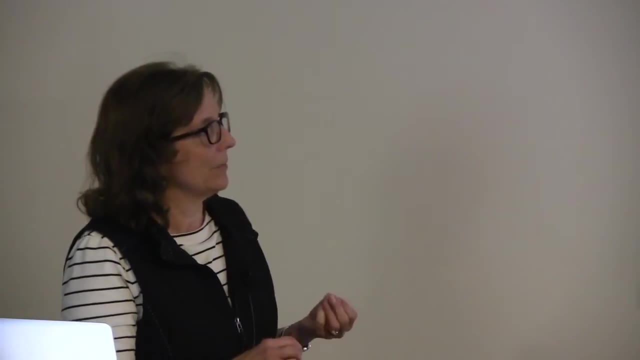 then we'd have a whole different situation. We would think: whoa, You know, it's going to be poorly drained. We're going to have to really be careful when we water it. It's not very well aerated. We're going to have to maybe even do something about it. 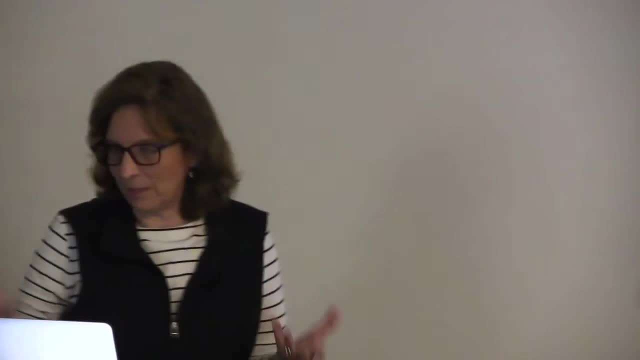 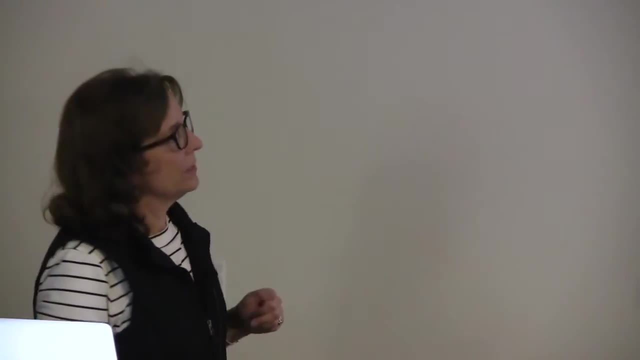 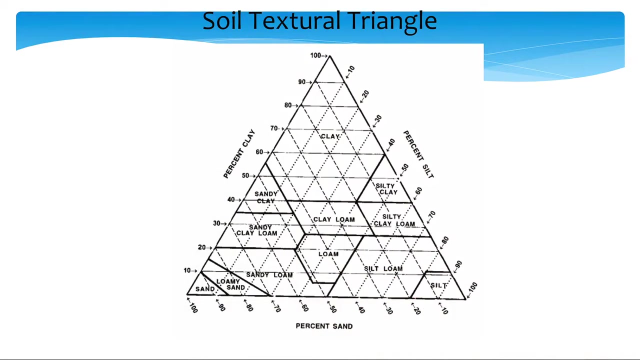 if that's the situation. So there's a lot of things that we need to make some compensation for when we actually figure that out. Now, what we do with this is what we refer to as the soil texture triangle. We'll take these percentages. 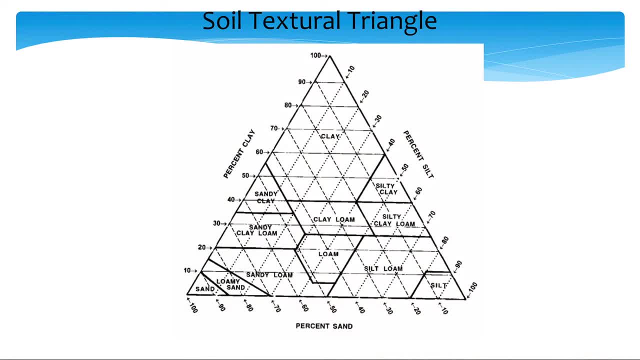 and we'll plot them on this triangle. If our soil type ends up in these upper areas, these would be considered fine, And then if they end up more down in this area, we would consider these coarse soils, And then, if they're somewhere kind of in this middle zone, 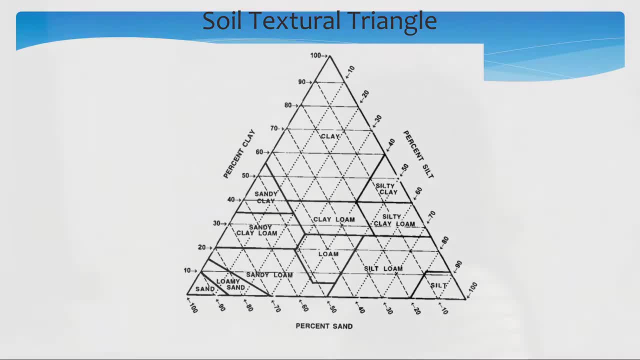 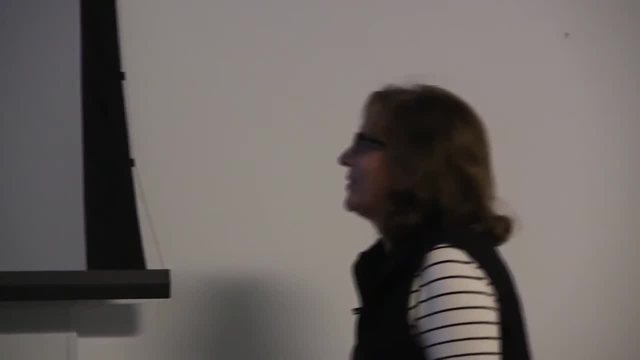 these are more of the ideal soils, with loam being considered. you know the holy grail That is like: if you've got loam in here, you're cool. You know that's going to be your ideal soil. You probably don't have to do much to it. You can grow anything. Most plants are happy there, Et cetera. You know your crops, your veggies, whatever are going to do really great. It's the people that have a lot of clay or a lot of sand that have to really think about. 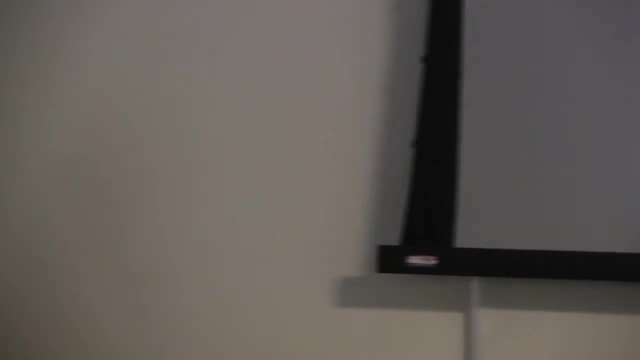 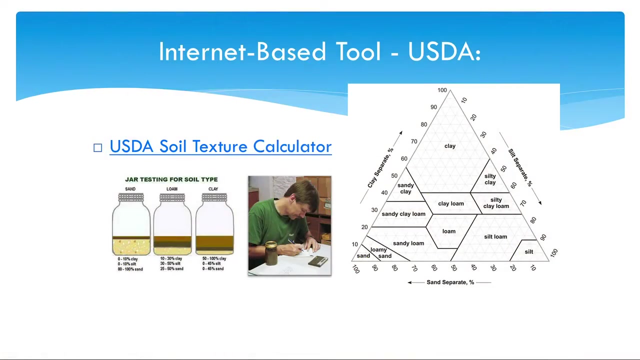 how they're going to manage that soil. Now we're going to actually do by hand and do a little math, but USDA does have a soil texture calculator online, So you can. You can plug in your percentages of sand or just two of them anyway. 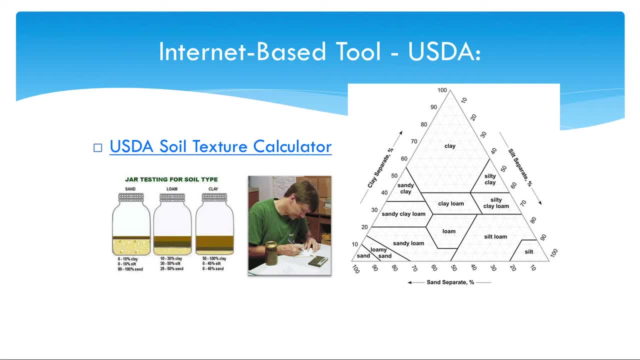 and it'll spit out the third and tell you exactly. you know where it lands on this triangle. It'll actually give you a little pinpoint for that, But we're going to do it actually using the triangle, so you get a chance to understand. 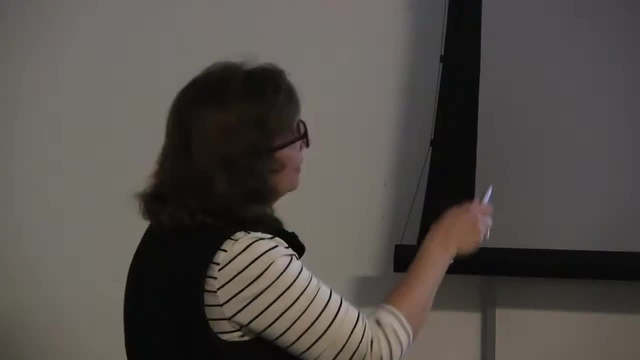 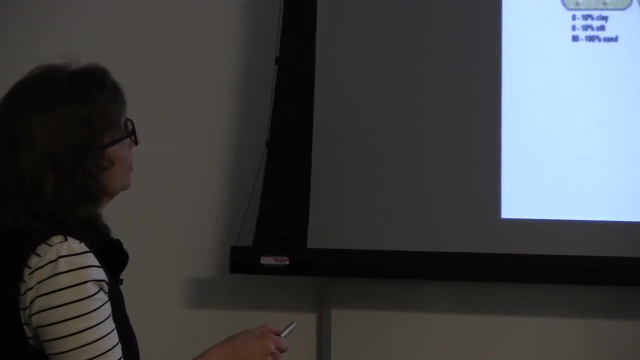 how that actually works. So again, our first sample here is predominantly sand. This one is what we would consider loam, where we have a good distribution of sand. This is one of the three types, And then this is more of a clay-type soil. 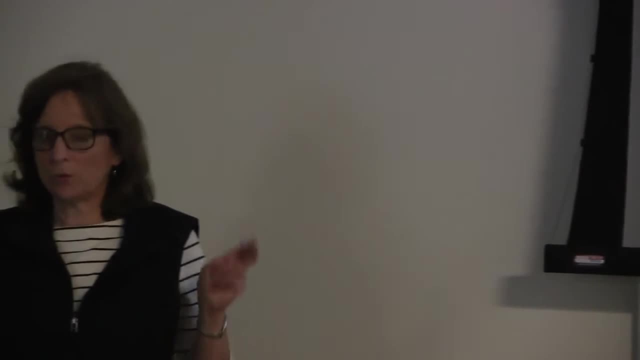 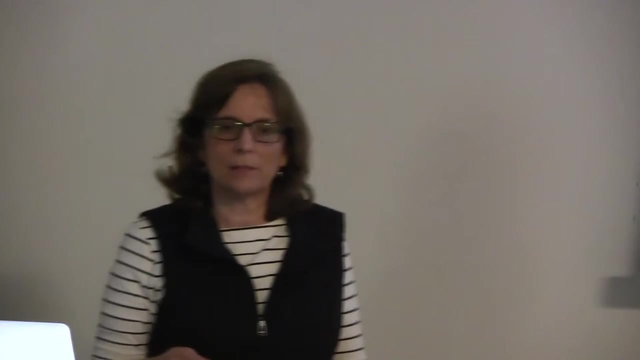 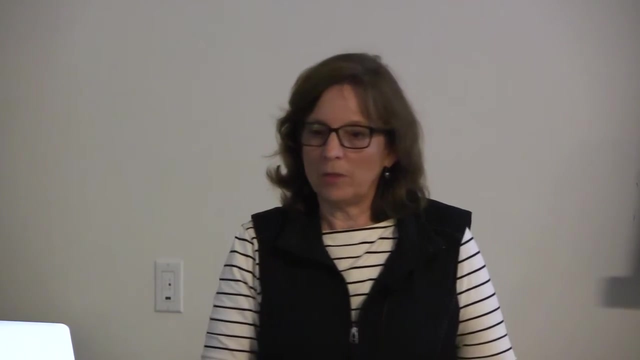 Okay, So yours will land probably in one of those three major categories. Now we want to know this because if you've ever looked at a bag of, maybe, gypsum or a bag of sulfur to add to your soil, maybe you've looked at even some different supplements. 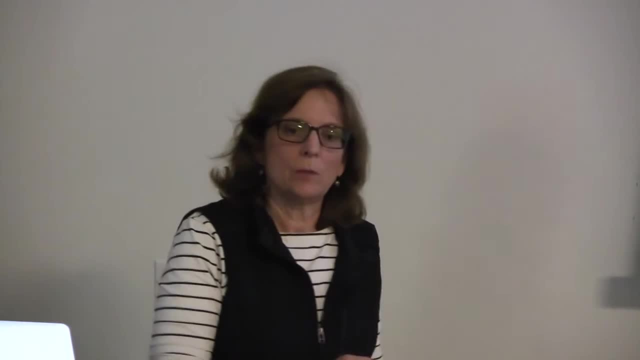 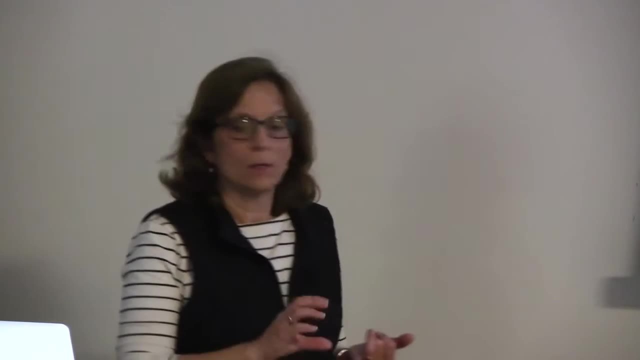 Perhaps you've looked at irrigation schedules. It's going to give you a different amount of minutes, a different of pounds per thousand square feet, based on whether you have coarse, medium or fine, Because, again, the surface areas are going to react differently. with calcium, with lime, with sulfur, with whatever you're doing to change your pH. It's going to react differently with certain types of- maybe even pre-emergent herbicides, depending on your soil texture or whatever else you're adding to the soil. 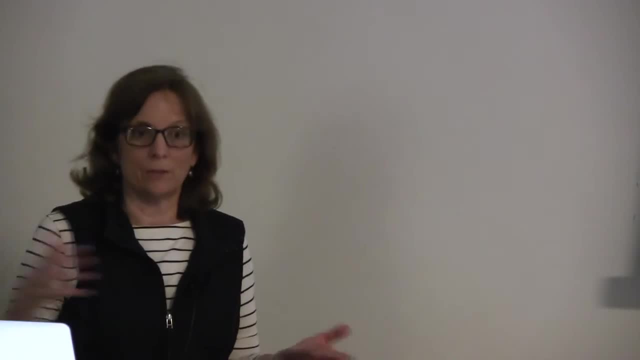 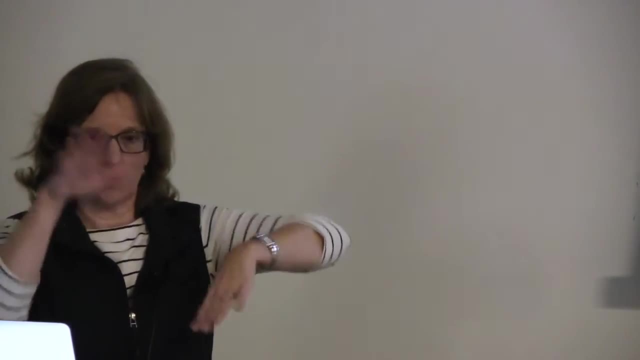 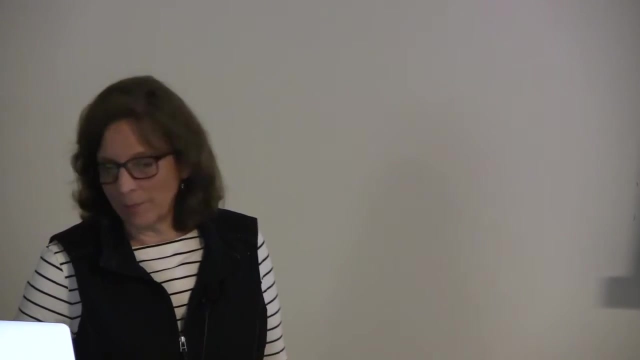 So your watering schedule again is going to vary depending on that. So we can come up with a pretty decent if our soil layers cooperate. by plugging it in here to the soil texture triangle, You can come up with that texture. 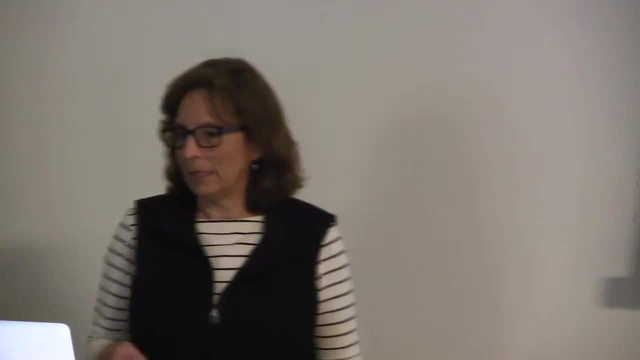 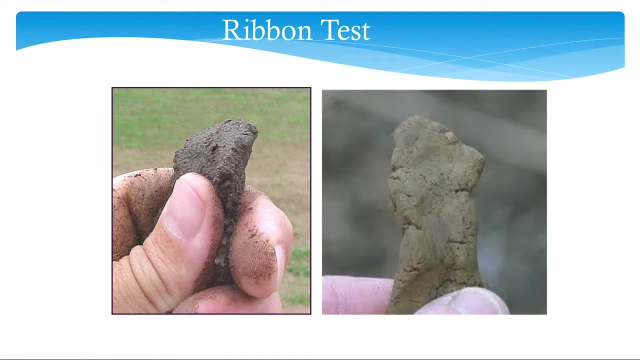 But we can also do what's called a ribbon test, And this is something that you can do. that is a little more of a ballpark, Okay, Something that you can feel once you get used to it, And we'll do this a little bit later. 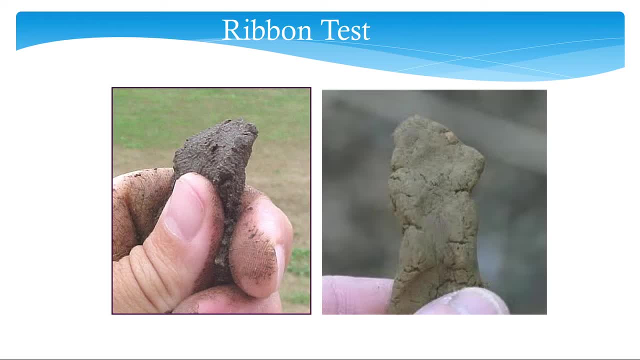 Julia, are you here? Are we going to do this after lunch? Yeah, Get messy, Okay. So we'll make mud pies later And I'll go through how you do that and the procedures. But let's say you're out visiting a client or somewhere. 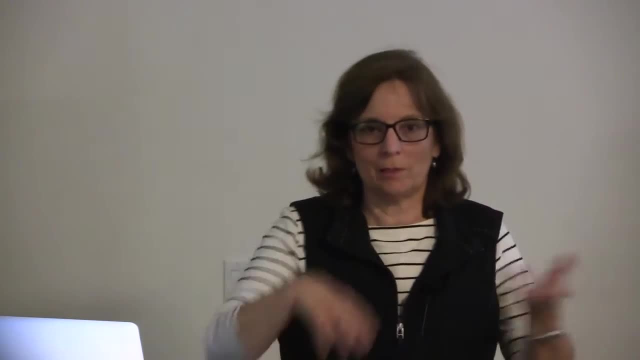 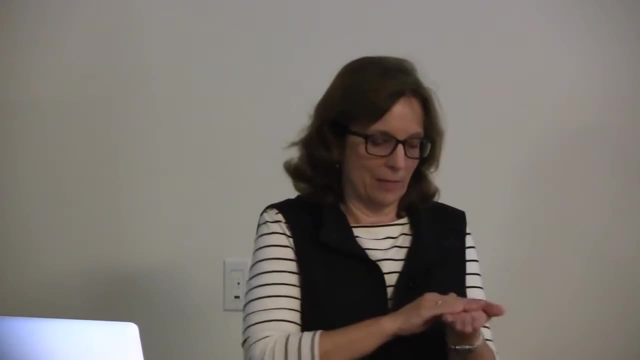 and you don't have time to do this jar test. You don't have two weeks or 24 hours or whatever to do it. They need to know now So you can actually do a ribbon test and just make a little mud pie, so to speak. 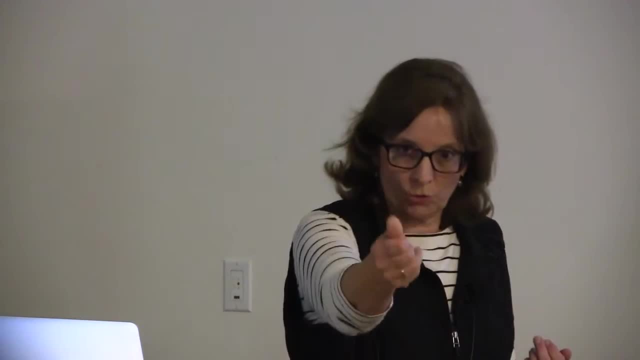 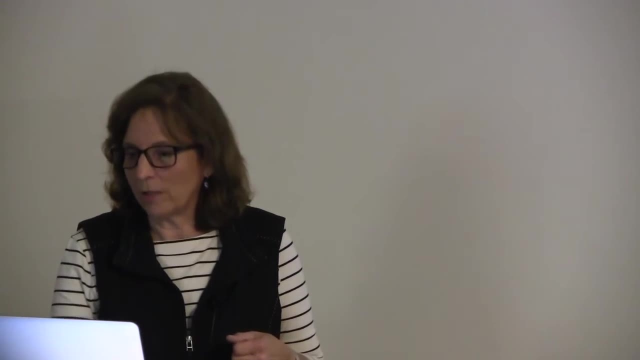 a little ball of soil in your hand, wet it and try to extrude it and feel it and see if you can form it into anything, And it will give you a good ballpark figure of the type of soil that you have. Now, again, we have a little bit of a YouTube thing. 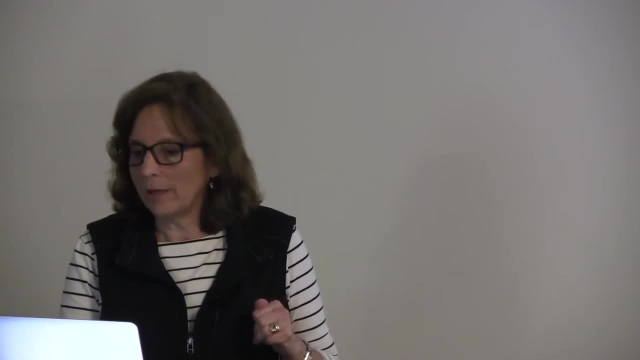 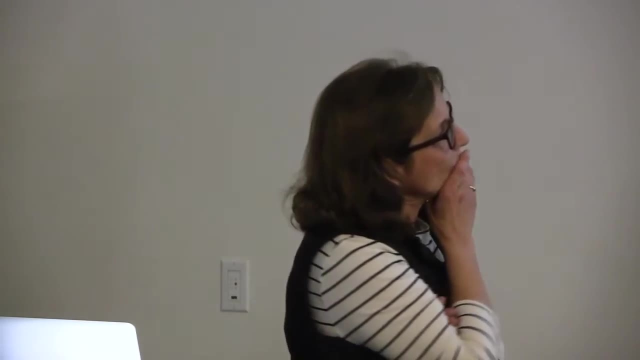 I think you've seen this, perhaps if you had a chance to look at your resources. But we'll show that later. We'll do it while we're actually doing it to give you an idea, But when you actually get that wet soil in your hand. 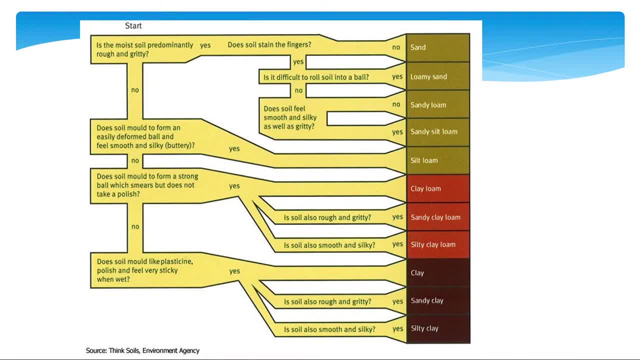 you're going to say: is the soil predominantly rough and gritty? And if the answer is yes, and it does not stain your fingers, you probably have what's referred to as sand. And again, when we say sand, we're going back to our soil texture triangle. 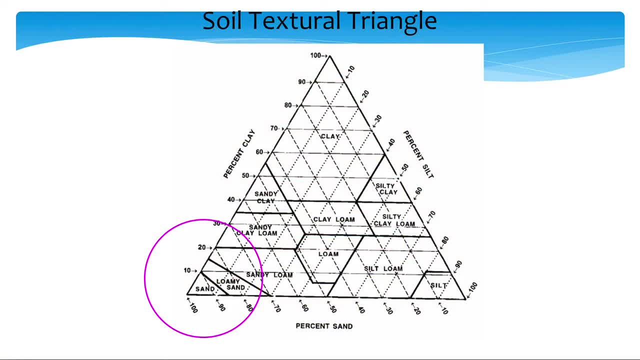 and we're talking about this little section here. So if you have somewhere between it looks like 80% to 100% or 85% to 100% sand in it, chances are you're going to end up in that particular area. 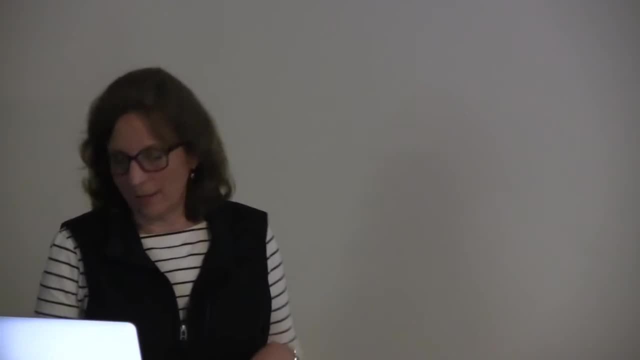 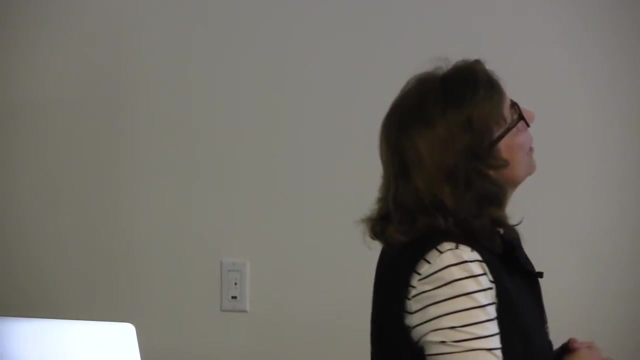 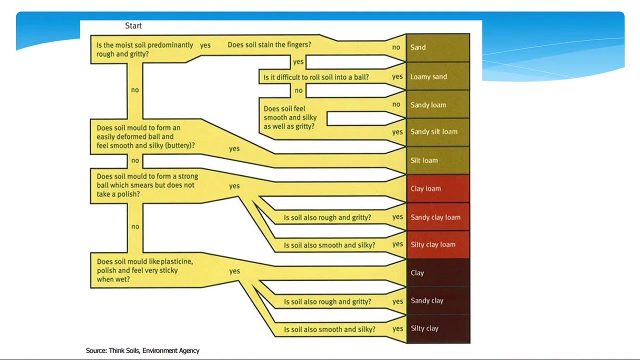 especially if you have less than 10% clay. That's where you're going to end up in the soil texture triangle and that's how this little hierarchy works. If, as you're feeling it, it does not feel rough and gritty and it forms a ball, 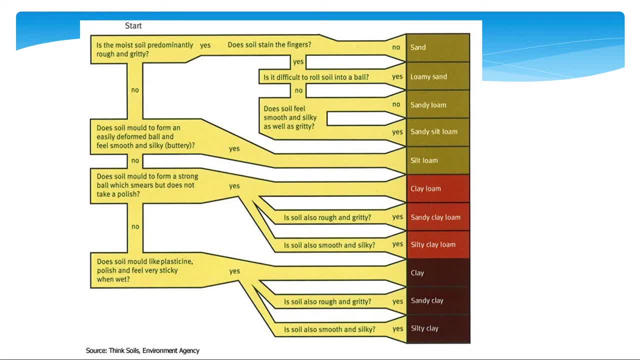 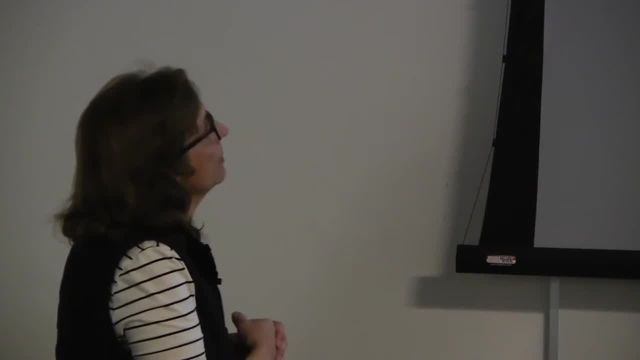 and feels smooth and silky, maybe even buttery, you'll end up with what's referred to as silt loam, If that still does not describe your soil, in other words, if you can make a really strong ball out of it and you can start to make vases. 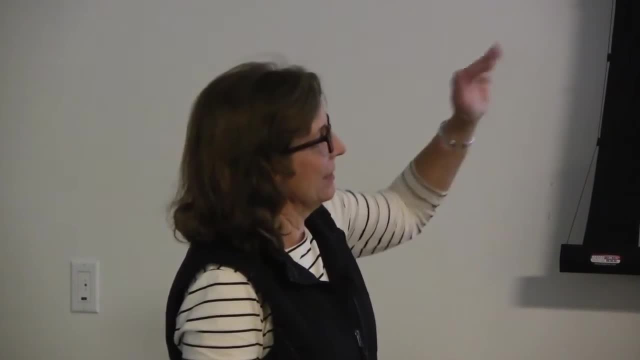 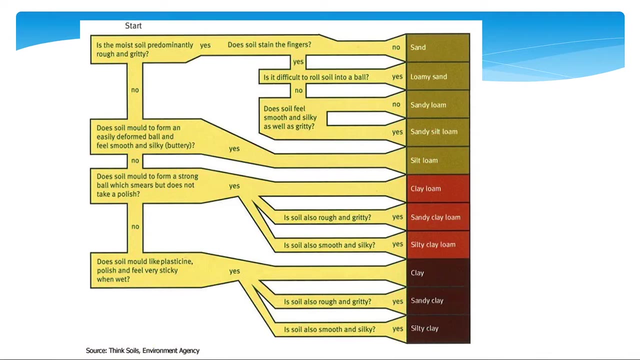 and snakes and that sort of stuff. now we're getting down into the really really truly clay And I'm not sure what does not take a polish means, but anyway. But if you have it, and it's also rough and gritty- 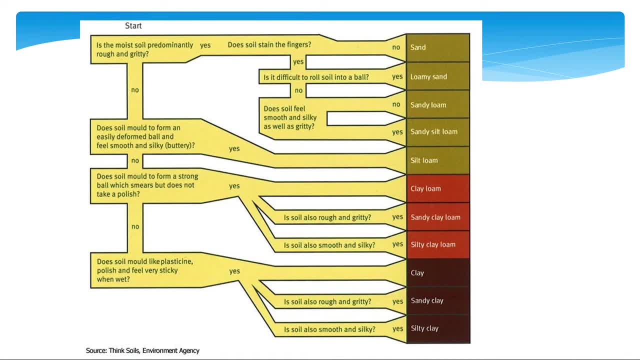 you can have what's called sandy clay loam, But if it's moldable and smooth and silky, it can be silty clay loam, But if it does mold like plasticine and it's a very sticky one, wet and you're really getting stained. 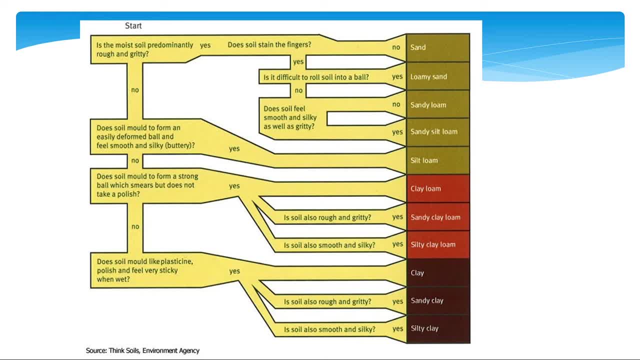 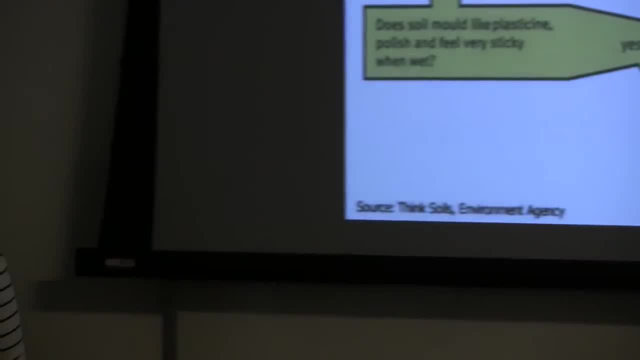 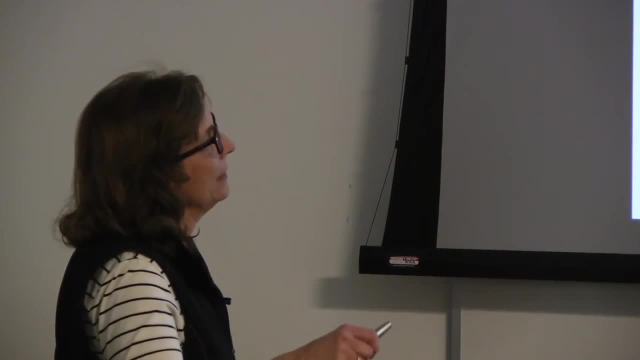 and it's just kind of a mess, you probably have clay. If it is rough and gritty, sandy clay, and it's smooth and silky, then it's silty clay. Now, the operative word in all of these is usually the last word in it. 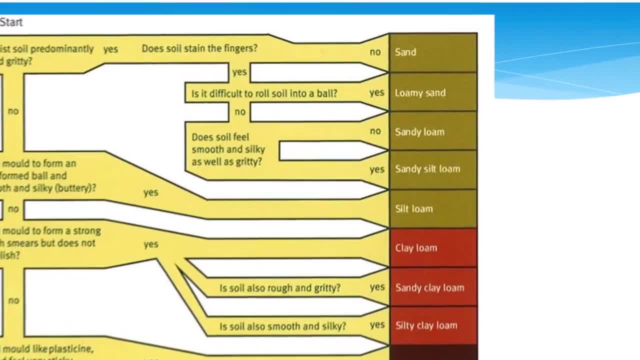 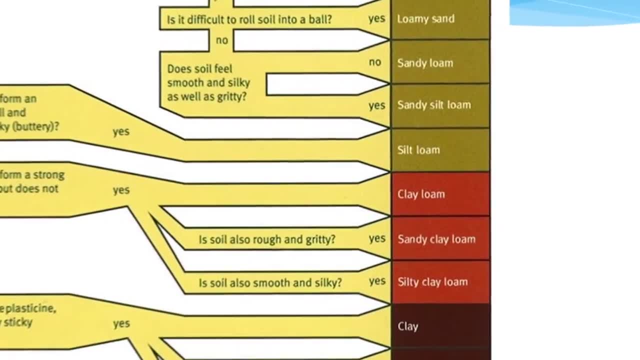 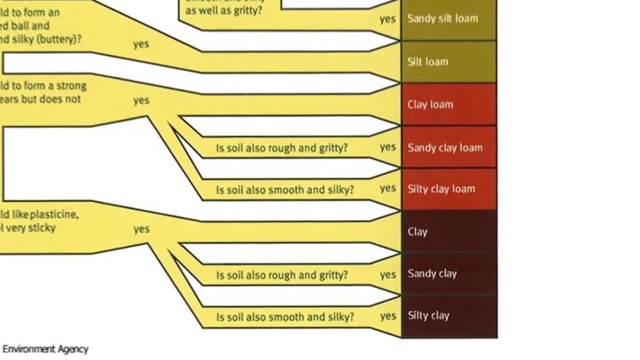 So we have these are really types of sand, sand and loamy sand. These are types of loam, Okay. so these are all halfway decent, Okay, And these are all types of clay. This is your very fine soils that are going to cause you some consternation. 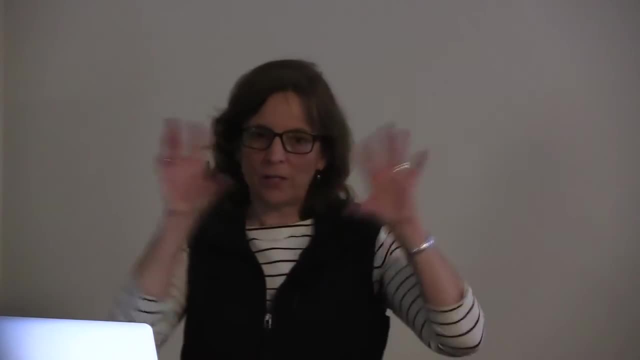 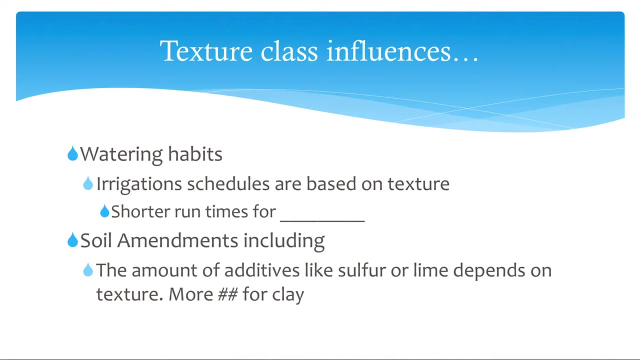 Probably Okay. so when we figure out our texture class, then we can make some inferences about watering habits, irrigation schedules and then again the amount or type of soil amendments that we might need to add to it. So if you're doing an irrigation schedule, 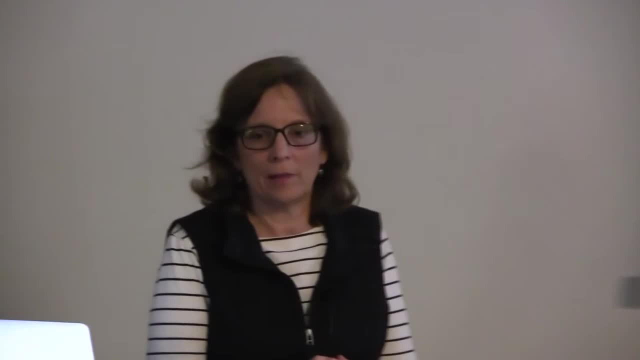 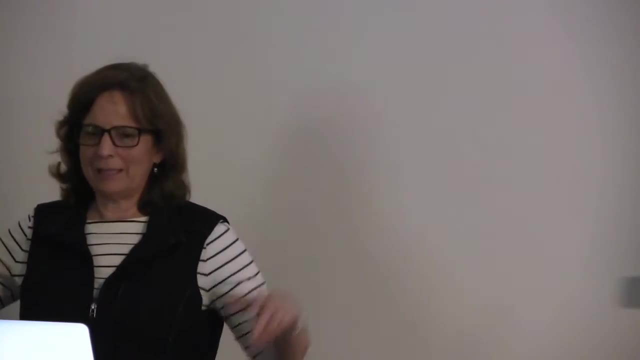 which one do you think is going to have the shortest run time allowed? Clay, Clay, yeah. So when you're doing your schedule, I know a lot of people say, oh, 10 minutes, or there used to be this ad. you know, don't water for more than 10 minutes. It's like 10 minutes is way too much for most types of soil. But you know a lot of old irrigation clocks. that's the default thing, especially if you lose power sometime. My neighbors. I'll tell you Crazy. I can go out almost any night of the week at a certain time, you know, sometimes it's midnight, sometimes whatever, and their irrigation's going off 10 minutes a zone, whether it needs it or not. 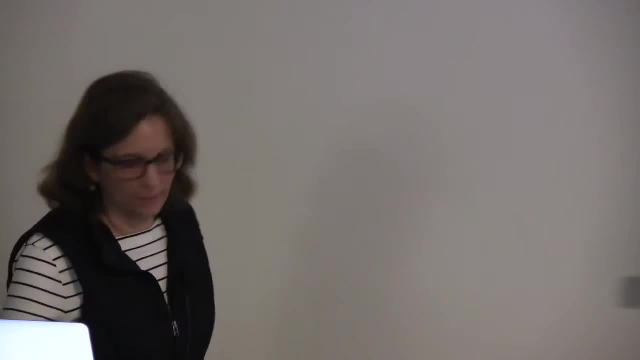 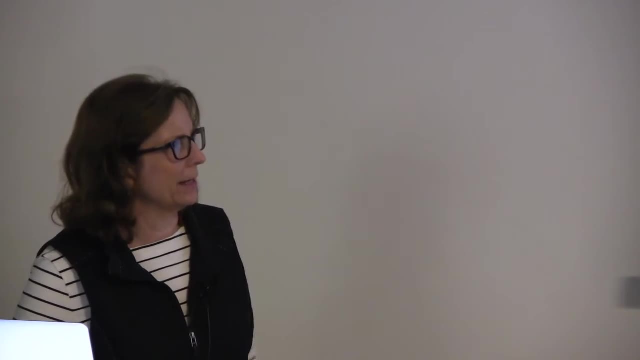 and it's you know. I shudder to think what their water bills are like, But they're not paying attention to it. They'll even be watering, you know, this time of year. Maybe they finally caught on. I haven't noticed it lately. 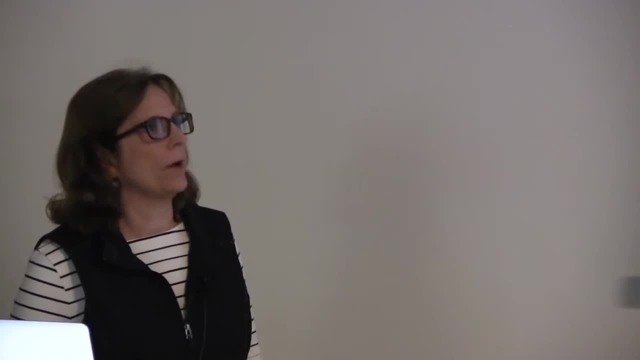 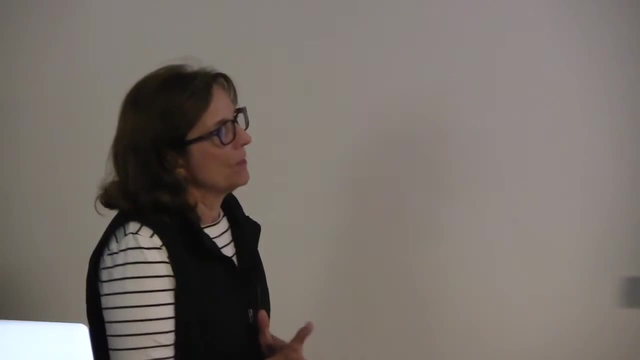 but a few weeks ago they were still watering for 10 minutes, no matter what, But you know you can't adjust your clocks. So, Anyway, this is. there's a website called Be Water Wise and it has what's referred to as 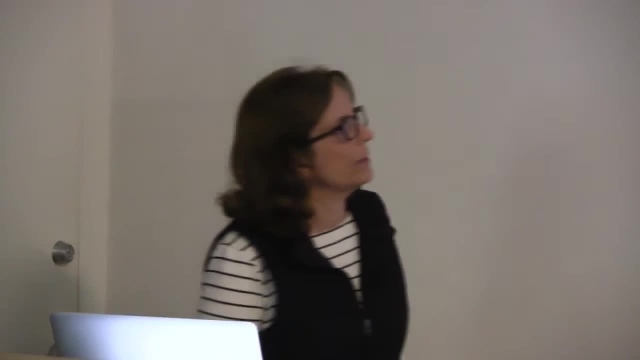 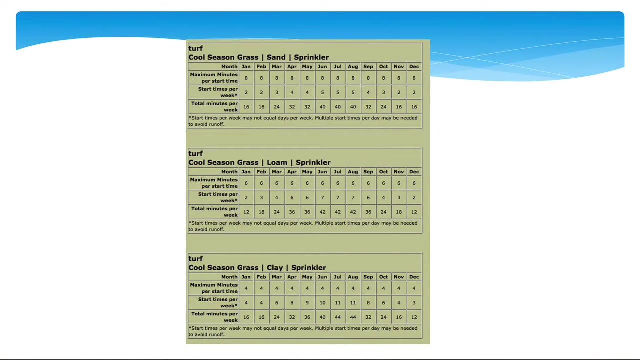 an irrigation calculator on it. that's kind of fun to play with. And I just ran through. I used the same zip code and the same type of crop, or cool season grass, same type of sprinkler. I didn't change that. The only thing is I changed from sand. 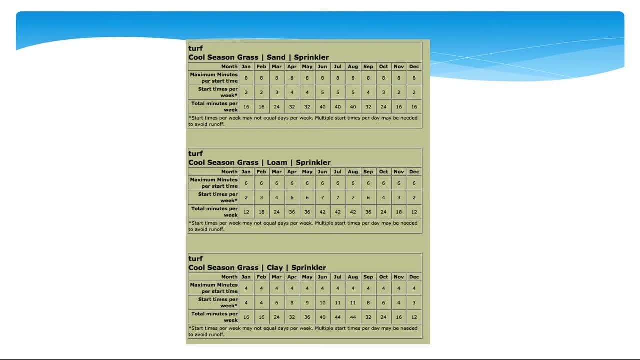 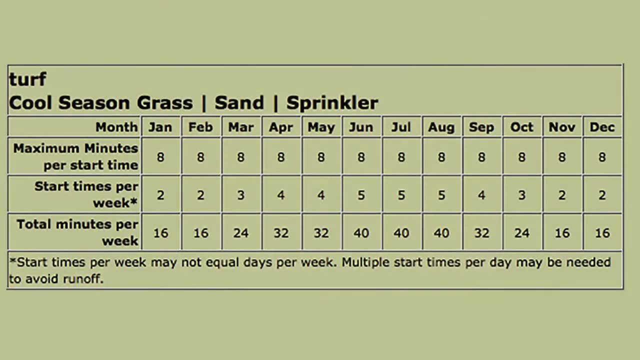 to loam, to a clay type soil, And what it told me is that the maximum minutes for start time on a sandy soil is eight minutes. In other words, you should not run any more than eight minutes on that type of soil If you have loamy soil. 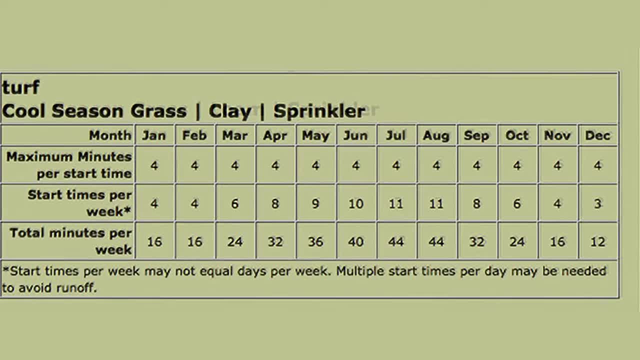 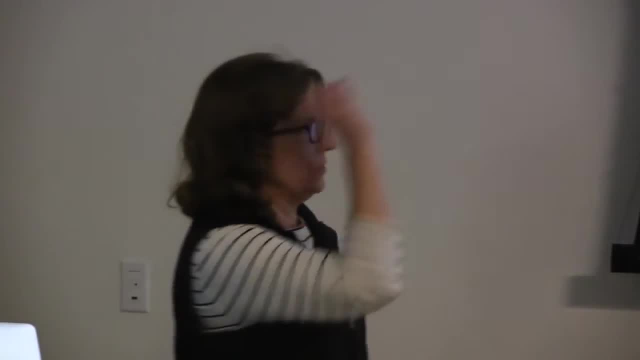 no more than six minutes. Clay soil no more than four minutes. So for a standard sprinkler, and again it depends on the precipitation rate of your sprinkler, but this is just the default type sprinkler that they have there. It's probably putting out. I want to say two gallons a minute or something like that, Which is high, very high. It's not the more modern type of sprinkler. Four minutes is the maximum that should be running. So again, it depends on the thing. 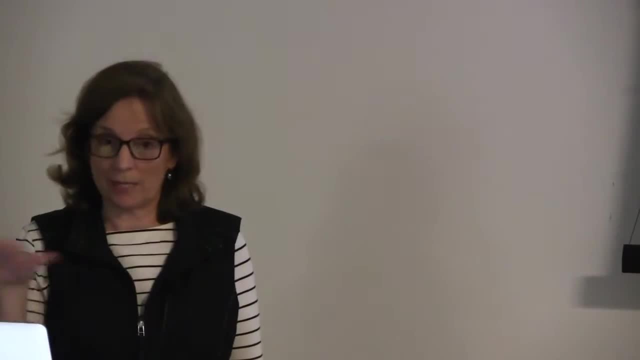 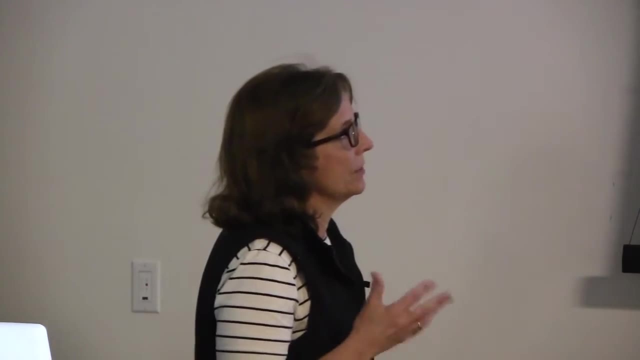 If you're using MP rotators it goes a lot longer. But if you have the standard old spray heads that are just kind of what we refer to now as kind of old fashioned or not, the ones that are rebateable, so to speak, 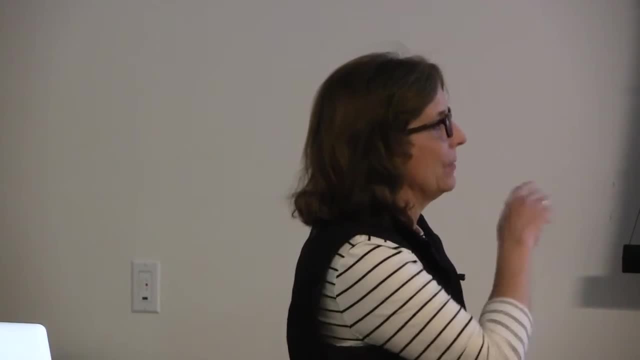 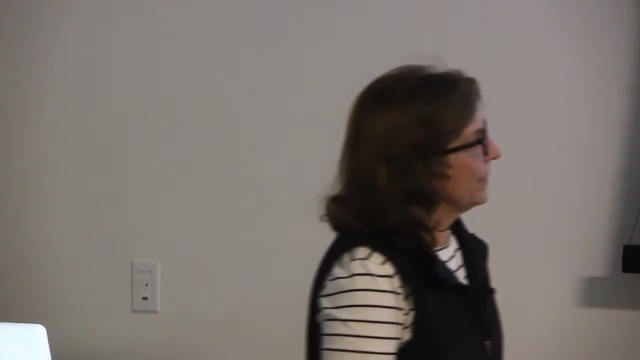 they're not the ones you should be using or continuing to use, But if you do have them, make sure, if you've got clay soil, that you don't run it for any more than four minutes at a time. Now, what that means is: 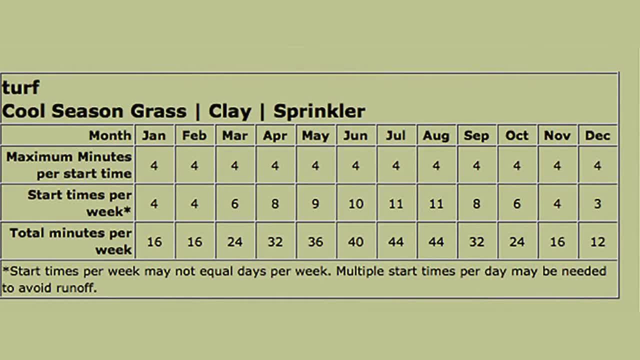 certain months of the year you're going to have to have more start times. So when we have a week where we maybe in the summer- June and July- we need 10 or 11 start times a week. that is a total of 40 minutes. 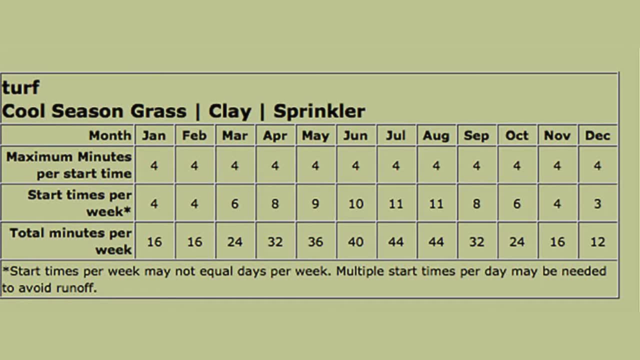 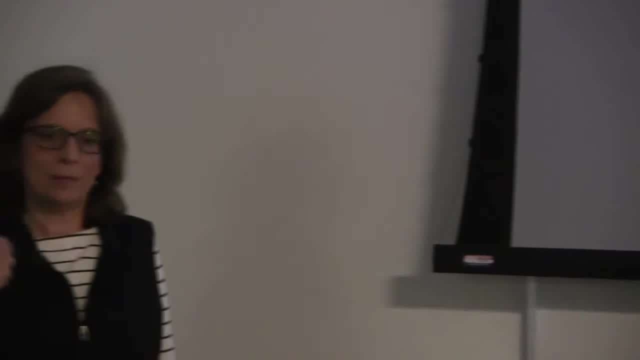 Not that we want to do it four days a week, but in an individual day we can run it for four minutes. stop maybe a few minutes, you know. half an hour to an hour later we can do four minutes again after that. first four minutes has soaked in. 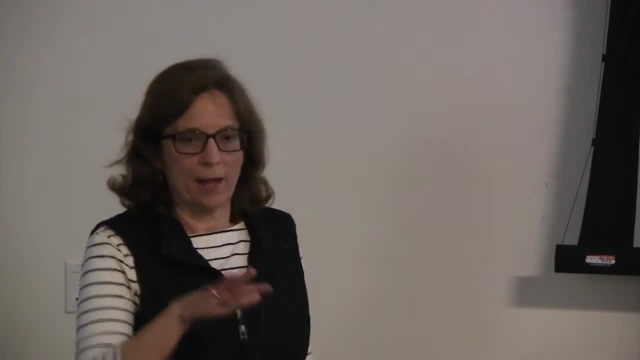 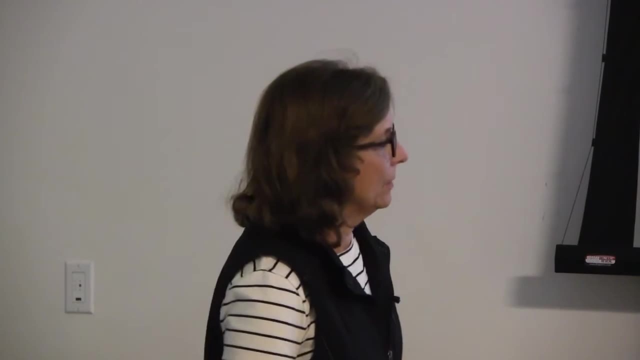 Do it again and again so that we're not putting all 40 minutes down. you know 10 at a time, or even you know 20 minutes at a time. That would be ridiculous for this type of sprinkler. that's on here. 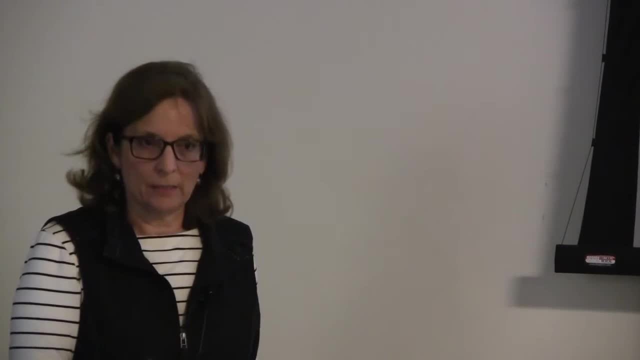 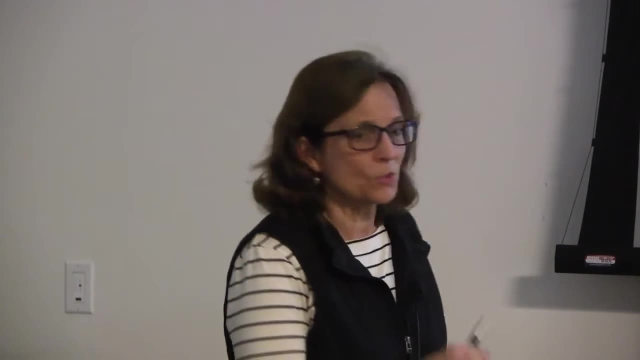 So again, you do what we call a cycle insertion: You soak and hopefully your irrigation clock is able to be set up for that type of a system. So smart controllers are important, using the right kind of equipment when you're watering. 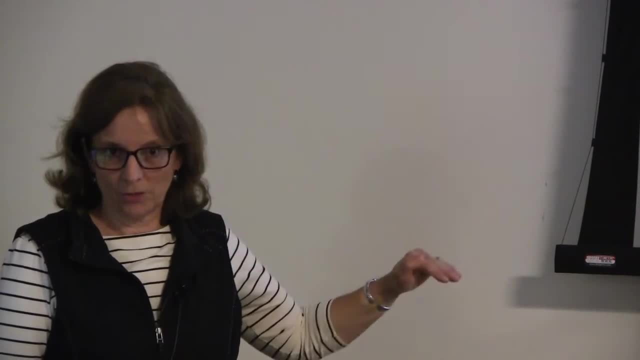 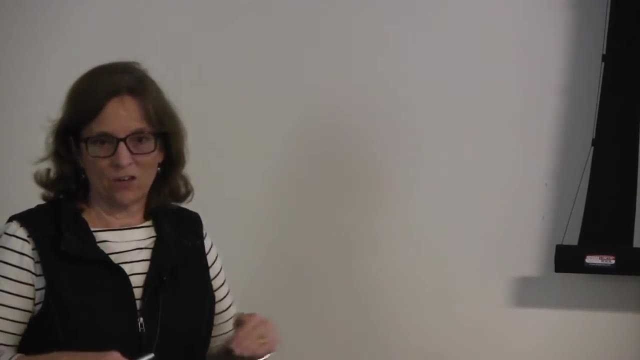 but understanding your soil texture, ballpark it. Do I have sand? Do I have the medium Loam? Do I have clay? If we can at least figure that out, you'll be much more water-wise and much more, you know, efficient in your watering. and save a ton of water And avoid runoff, wasting, et cetera. So, again, it depends on what you're growing- In this case, cool season, Depends on your zip code, Depends on your soil, Depends on the type of sprinkler. So I'm kind of simplifying it here. But if I only change the soil, it really dramatically changes the amount of run time that you can have at any one particular time. Okay, So that's one big implication of our soil texture. Now this is a little bit difficult. 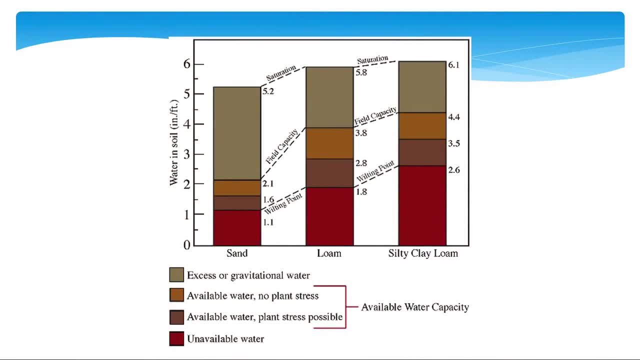 to understand sometimes. But what this illustrates to you is the amount of water holding capacity that the different types of soils have. So I guess I better talk about those soil moisture constants here a little bit. So if you can imagine a sandy soil, 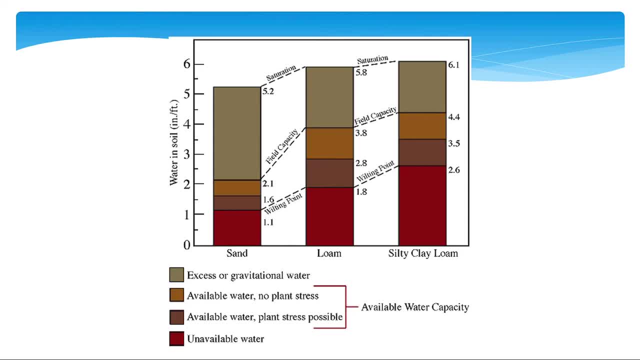 reaches saturation and then, at what we call field capacity, that's, after all, the water's drained away after a rainstorm. maybe about 48 hours later, it reaches what's called field capacity And at that point in time it is able to hold. 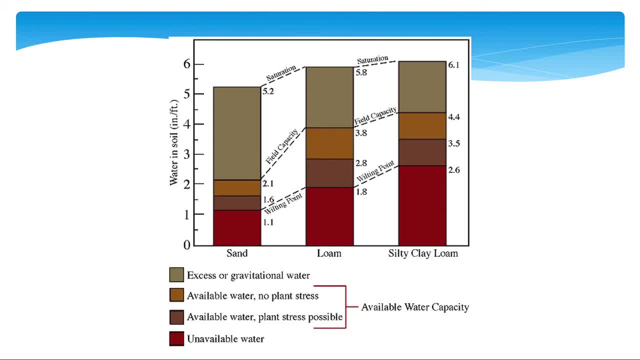 between the wilting point and field capacity. This is your ideal soil-water situation here, And so it has this amount of soil in this so-called sweet spot. Your low soil is holding a lot more at that point, And believe it or not, 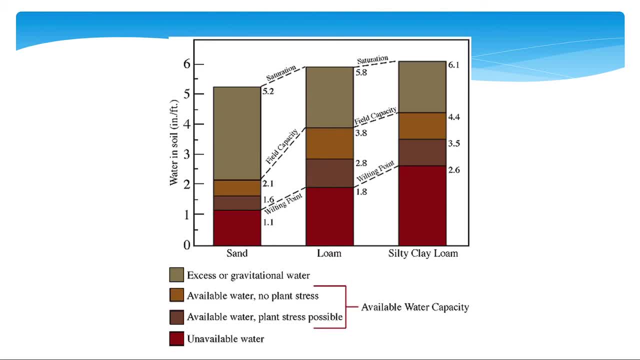 as you get more into the clay, it has less available water than it does in this ideal situation. It's got a lot more water in it overall when you add all these columns up, But this is considered saturated and that's going to just drain away by gravity. 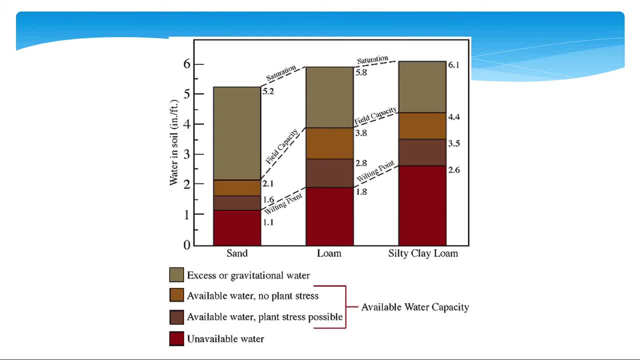 This is what's held onto those soil surfaces: soil particles. So it's holding onto a lot of water, but it's not all available And you get less and less in this particular spot as you go to larger and larger particle sizes. 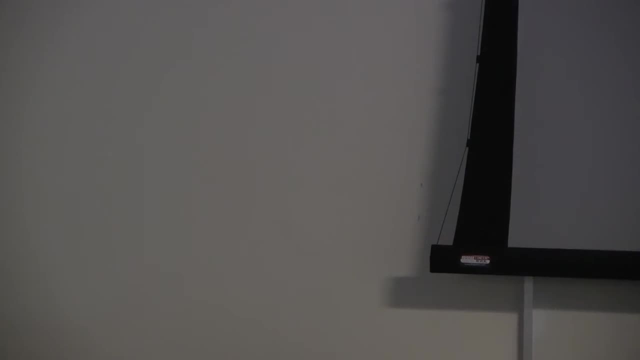 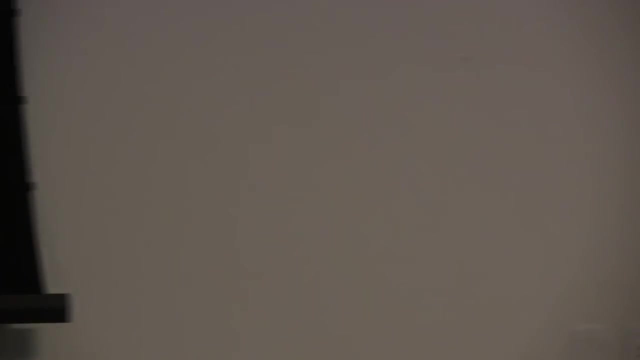 One of the best ways I have to illustrate that concept is with a sponge, And if you have a sponge, it could be my Vanna here. Is this dry? Yes, it is. We have a dry sponge. Have you two ever met before? 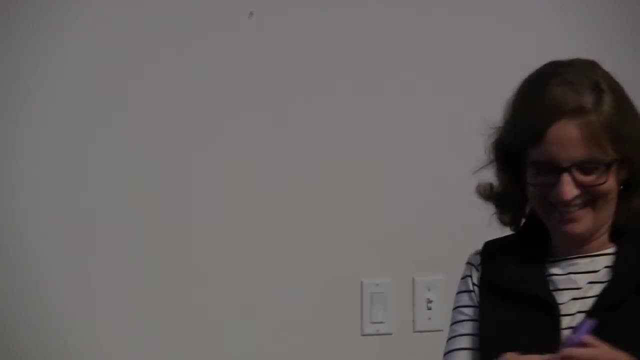 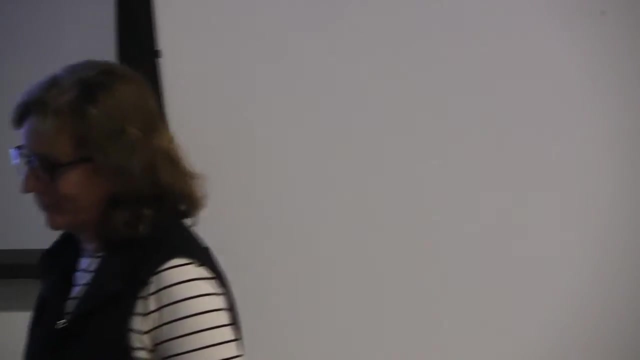 Yeah, what's that? Have you two ever met before? No, we haven't Not met before. yeah, So this is just a good old dry sponge. It's been sitting on a shelf probably for three, four months or so. 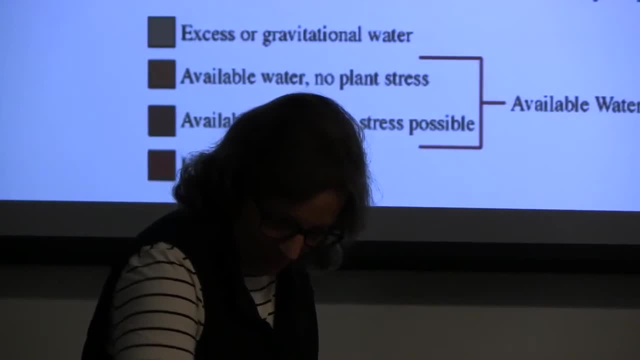 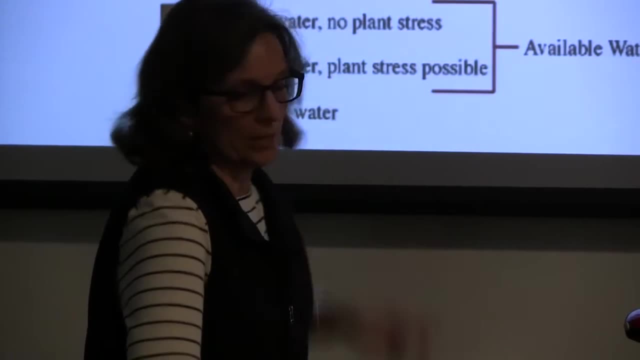 Not wet at all And I've got a little bucket of water here and I'm going to just soak it in here And I'm going to do what's called saturation. So I'm going to, at saturation point, all of the pore spaces are filled with water. Okay, so this can happen after really heavy rainfall in your soil. if you think of your soil as a sponge, It's totally filled with water. What's the first thing that's going to happen, do you think, when I pick this up? 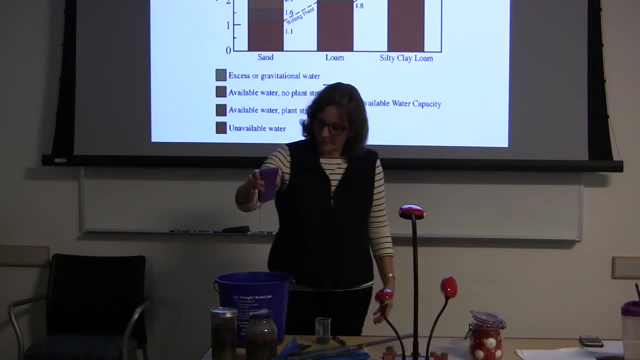 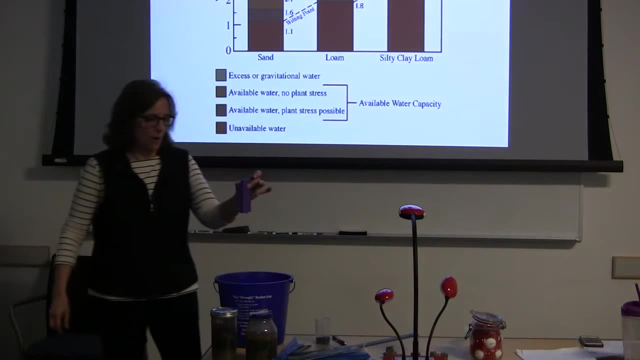 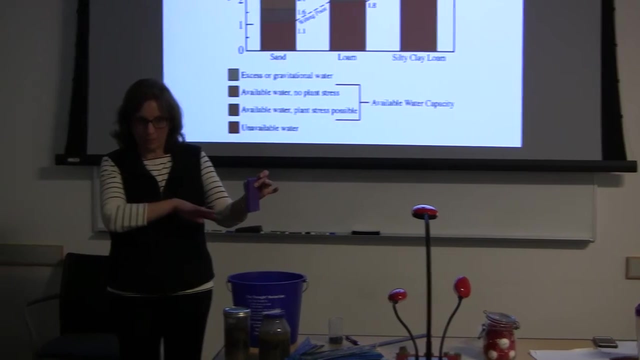 Yeah, we're going to lose some gravitational water. Okay, So the force of gravity is going to take the loosely held water and it's going to drain off, And when this quits dripping- which hopefully will happen fairly soon- we'll reach what we call field capacity. 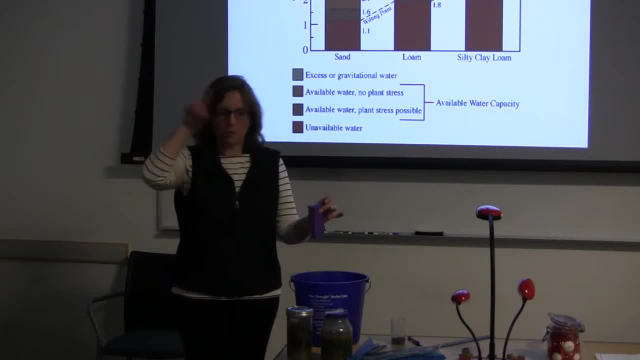 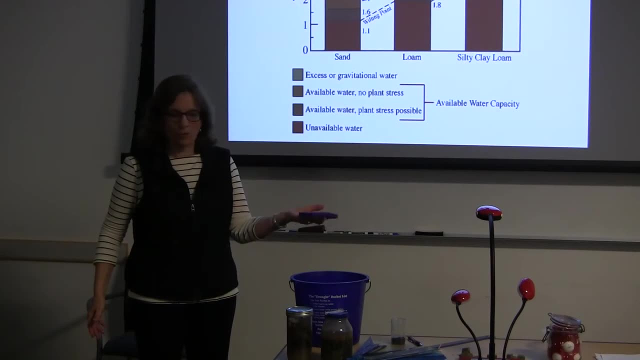 And at that point, I think that's when we have that ideal pie chart where you've got, you know, half the space is filled with air, half the space is filled with water and it's no longer considered saturated. So this is really nice for plants. 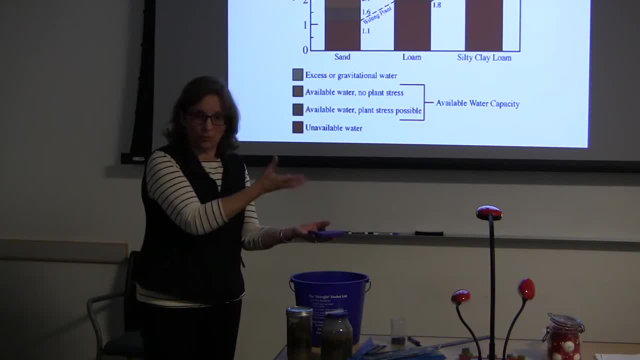 They can use this water very easily without exerting a lot of effort, Because in those pore spaces, which we've got a mixture of sizes here, water is held fairly loosely. So if I'm the plant roots extracting water, I don't have to exert much energy. 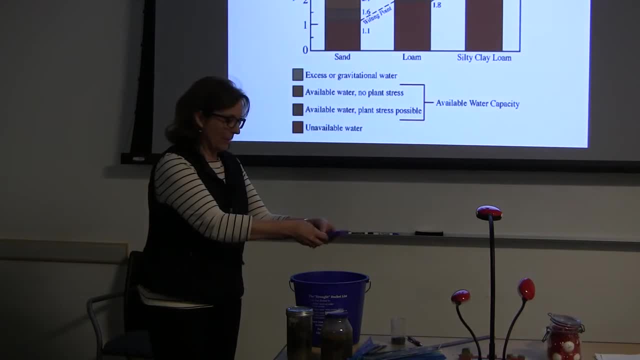 as a little root hair to get that water. Okay, So I'll go along and I'll use water and use water until I can't use it no more, or it's getting harder and harder and harder to get that water out of there. 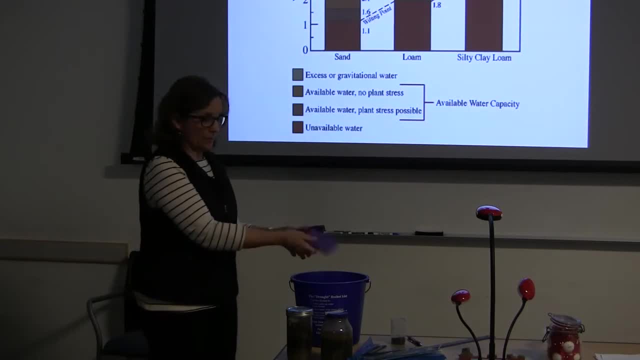 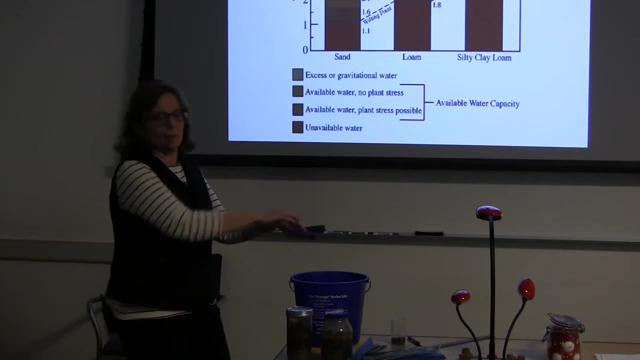 Okay, so I've got to really exert some effort. Well, if I have to exert that much effort as a plant root, I am definitely at the wilting point. I just I can't, can't even, you know, I can't do that. 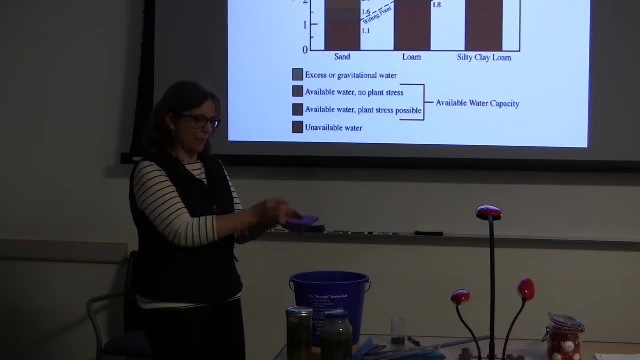 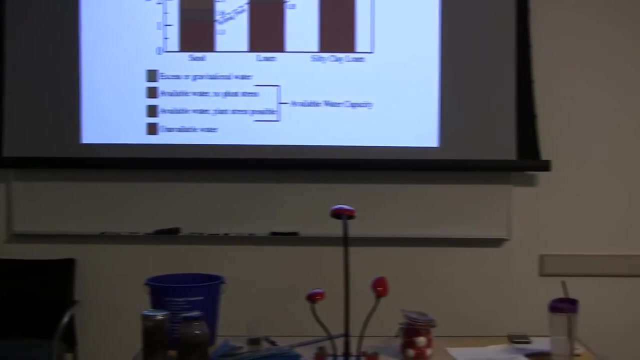 So it's just too much of a force that the water's held to that solid object, those soil particles, that my plant root does not have the ability or the energy to get that water away. So now I ask you, is this dry? 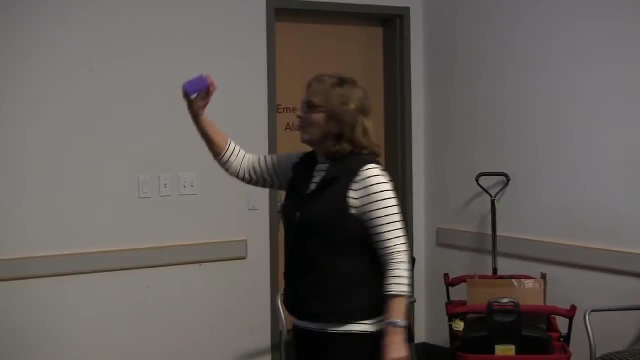 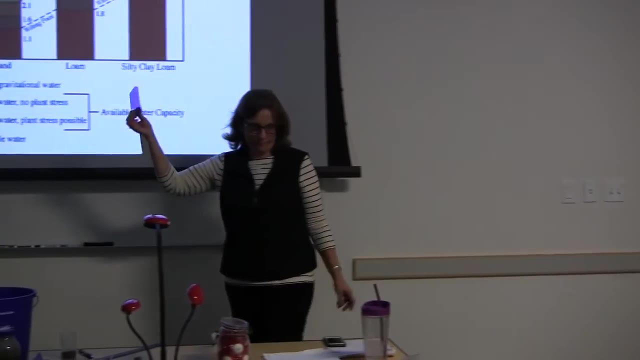 No, No, it is moist, correct. So the water that's left in here is what we refer to as unavailable water. Okay, It is at the wilting point. If I was trying to grow a plant on here, it would wilt. 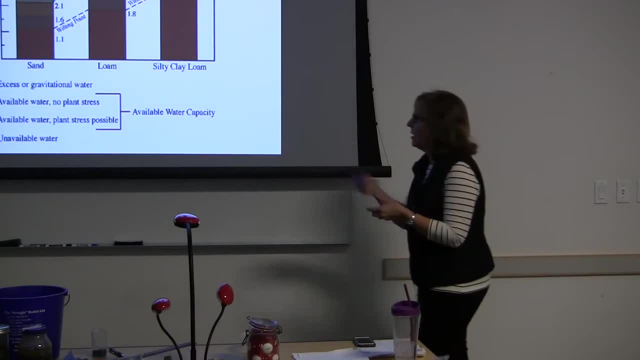 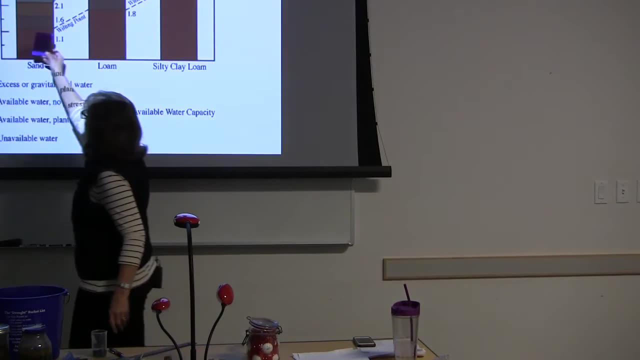 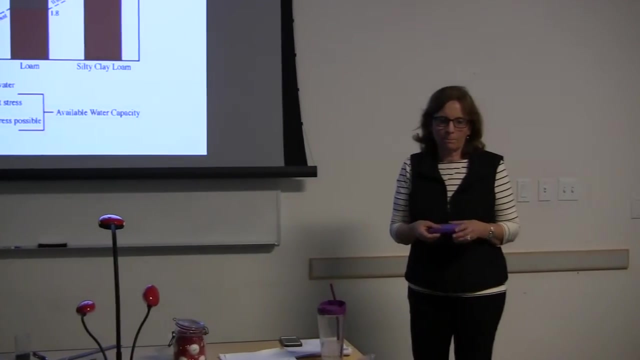 Not enough water available to it. So this is the unavailable water and this is the water that you're seeing here, in the more clay, the medium and then the coarsely textured soil. Would a plant respond the same way to unavailable water and just dry soil? Yes, When it gets to the wilting point. even though there's still technically water in the soil, this is still technically moist. It's just not available for that plant to get it, And so it will begin to wilt Now when we have an irrigation system. that's automatic. we would probably like to water it or turn that back on before it gets to the wilting point. We don't really want our plants to wilt. You know what happens when plants wilt. Yeah, they could die. That's the worst case scenario. What else? Yeah, they're more susceptible to insects and diseases. Somehow they just seem to know- it seems like that. they can, you know, go to that, And then if you're trying to produce a crop, it's cutting down your photosynthesis. It's not able to produce, Your fruit's going to be smaller, Maybe your tomatoes won't be as juicy, etc. So you want to avoid the wilting point. but you really don't want to go over field capacity either, because if you go over that, what happens? 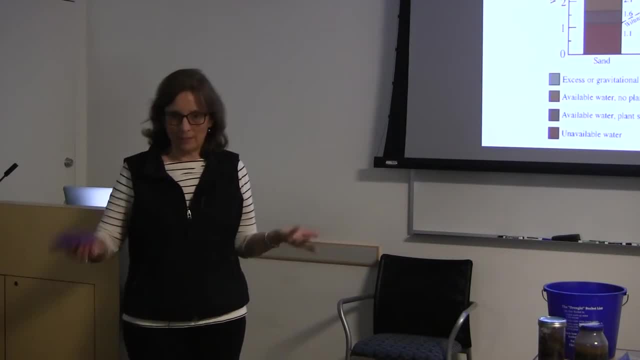 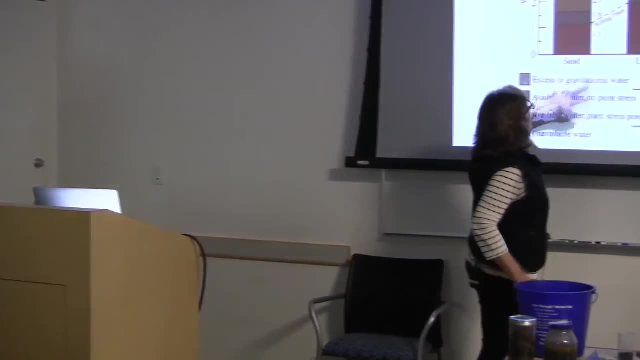 Saturation, Saturation, or you're wasting water. It's more water than it needs. So, again, to be water-wise, you want to keep it in this sweet spot here, And so when we have to do that in any particular soil, depends on the soil texture. Which one do you think we're going to have to turn on more often? Sand, Yeah, the sand, Because it's probably going to reach that wilting point a lot quicker, And so we may have to actually water it a little more frequently. 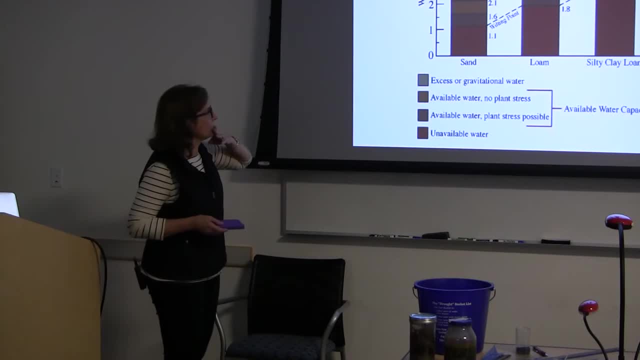 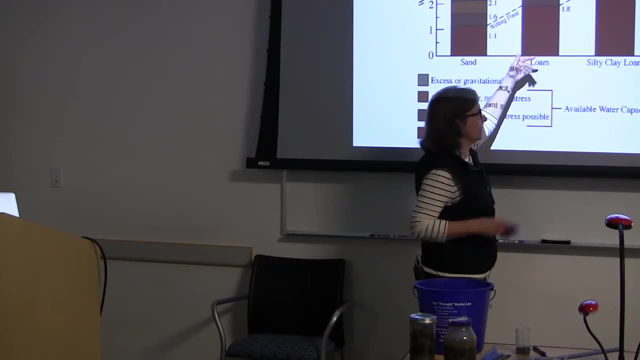 just to keep those plants from wilting, Whereas if we have some clay in the soil and we begin to get into this ideal relationship with sand-silk clay or even up here, you know, we don't have to water as often. 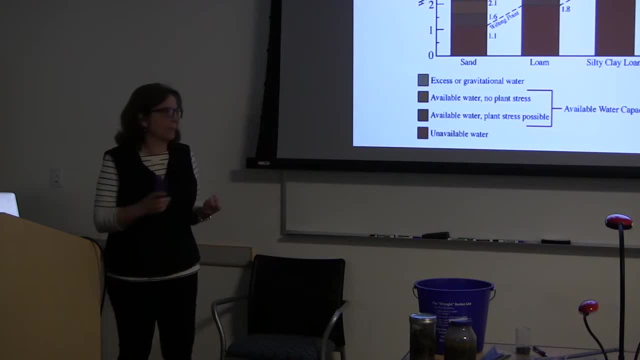 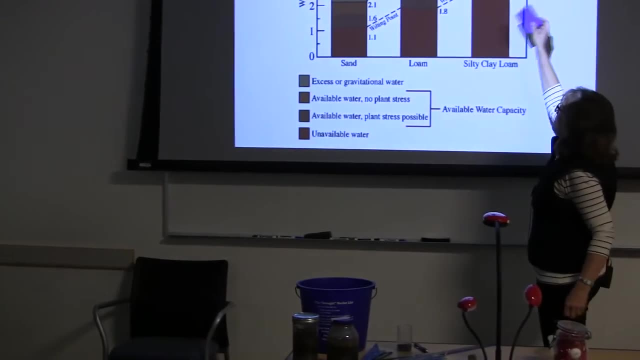 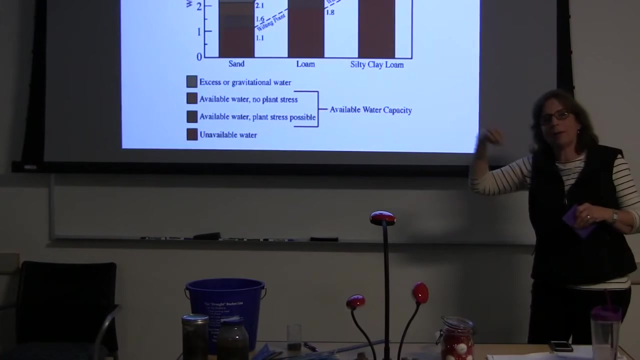 Okay, Because it has water-holding capacity. But again, if you get too much clay in it, most of it's going to be unavailable Again, holding tightly to those soil particles is a very strong attraction. It's stronger than the root being able to hold it. 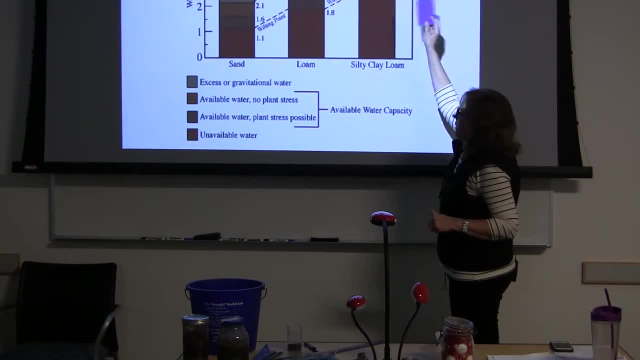 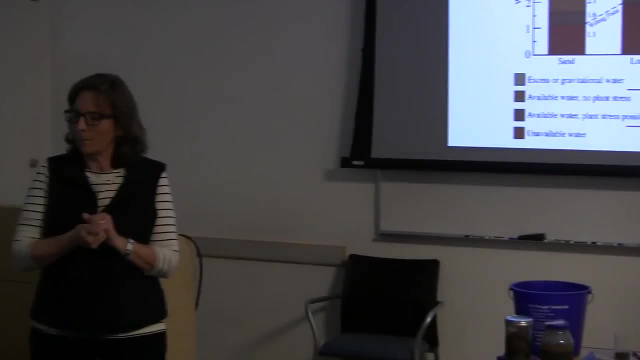 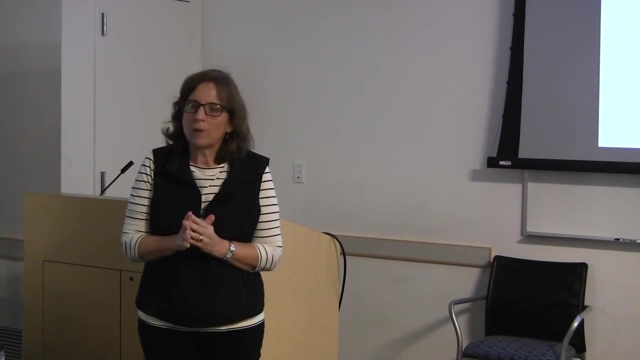 It's going to take it away. So, yes, it's wet, but it's unavailable. So, again, that's why we like that happy medium. I have a question. So is the ratio of water to oxygen the same percentage in each of these? Probably not technically, because of the larger coarse spaces. In a sandy soil you're going to have a lot more aeration because of the larger particles, And in the loamy soils you just have smaller and then as you get to the more clay soils. But I mean in each column. So depending on which soil you have. Yeah, I think technically you would find a little difference between them And I remember coming across a graphic to that extent. But yeah, So you might have that 50-50 ratio perhaps. but they're not going to be large sizes. They're going to be much smaller pore sizes. So not that there might not be some oxygen in there, but it's not going to be as frequently and or as continuous. So you know again, you either do something about your soil to amend it. or you change your watering practices. You settle on which plants are going to be happiest under which one. But to try to grow, you know something that needs a lot of water, like bamboo in a sandy soil. you're going to be wasting a lot of water. Or your water bill is going to be really high And that's maybe not the most efficient thing you could be doing. Cactus succulents- native plants, plants that are more adapted to go with those highly aerated soils, longer periods without water. 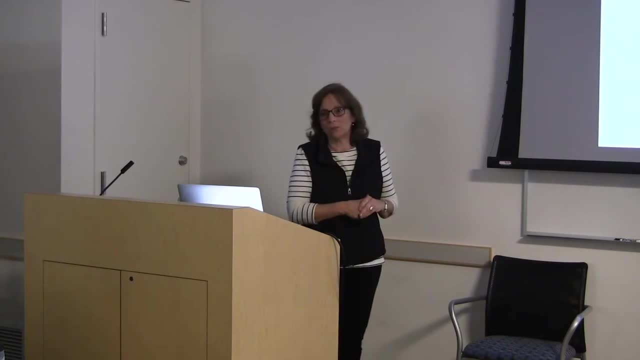 those are going to be your best plant palette to use in that situation. Or do something about the soil, Okay, So if you don't want to have that type of a plant palette and you'd rather increase your water holding capacity, 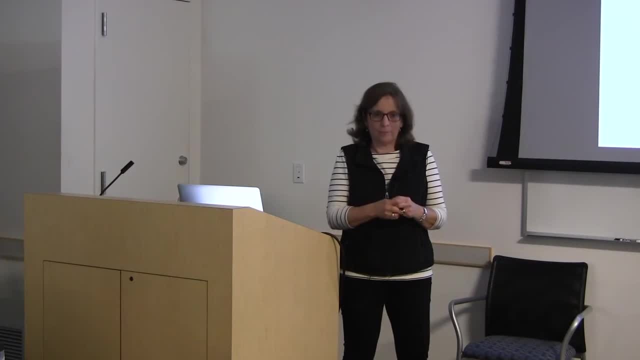 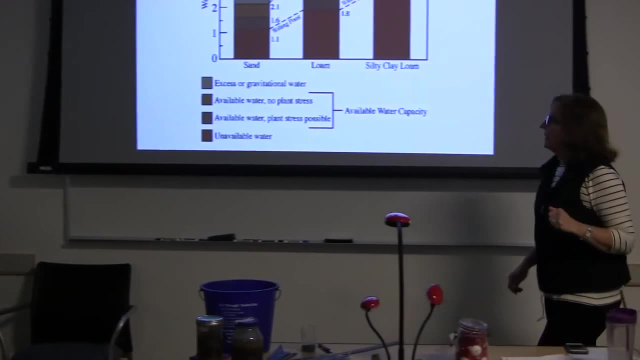 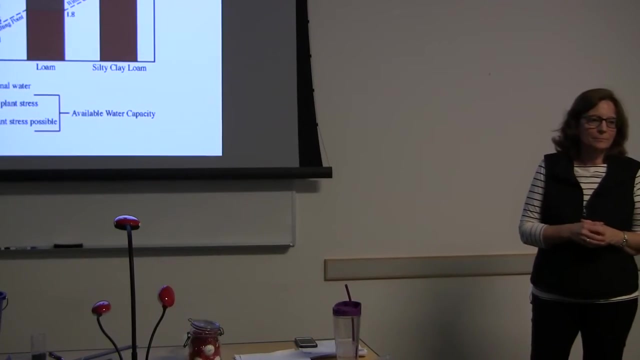 what can you do? Add organic matter. Add organic matter- Great. What if you've got high water holding soil and you don't want to just grow cattails? what can you do to increase the aeration? Add organic matter. 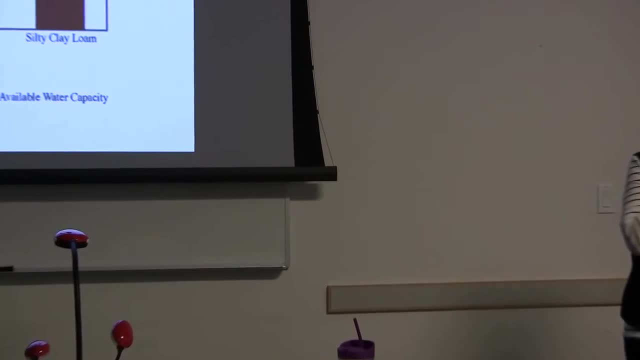 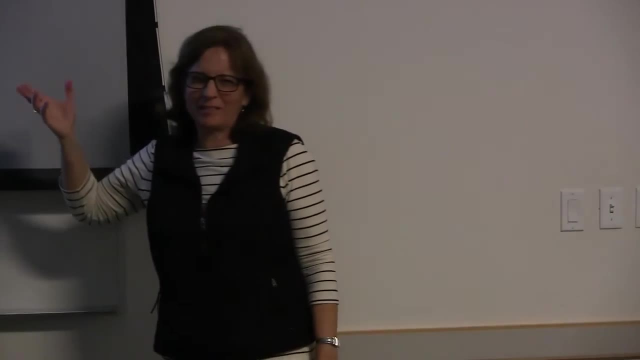 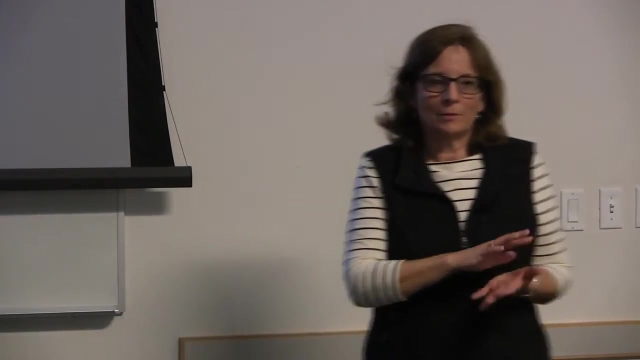 Add organic matter Unbelievably, it's the same thing. Okay, It's not really practical to add sand in this situation. It's very expensive. I suppose you could do it, but I've always been told and heard and kind of think it's true. 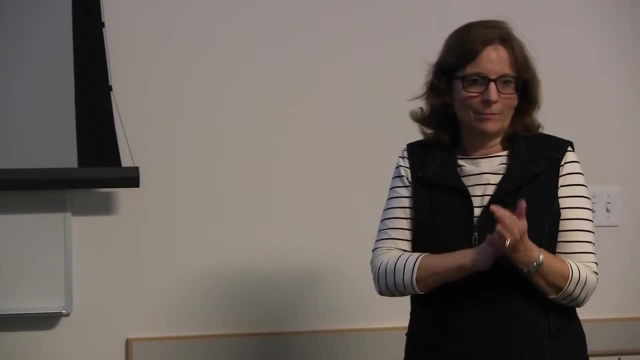 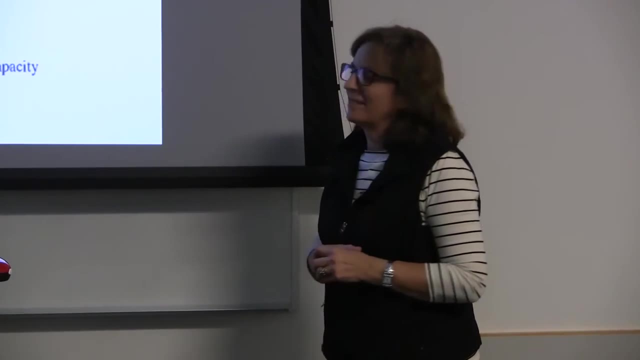 when you add sand to clay, what do you get? Cement or bricks. That's how they make adobe, The adobe walls and bricks and stuff. So it's not really a practical thing to do, but organic matter is going to get you what you want a lot quicker. 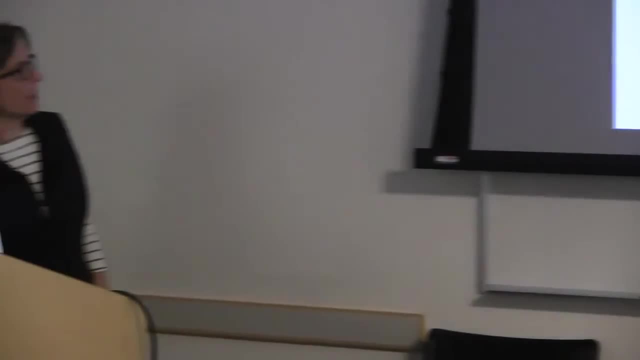 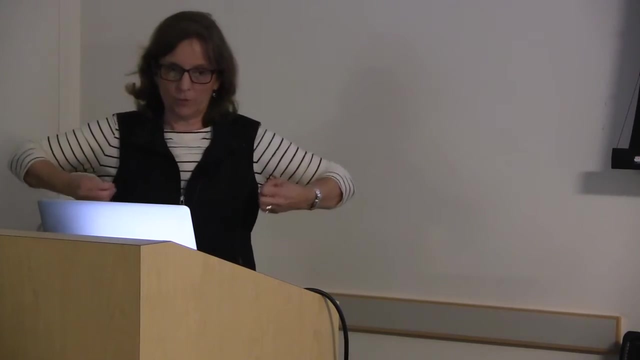 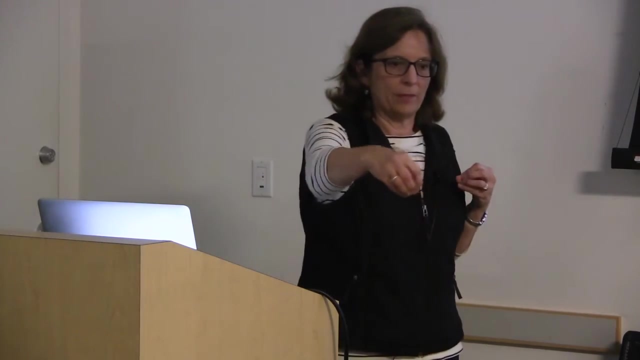 and a lot more easily. Now, another thing that's kind of interesting about your soil texture is how water moves through the soil. So if you have a drip irrigation system, especially those inline drip emitters where you've got every 12 inches- 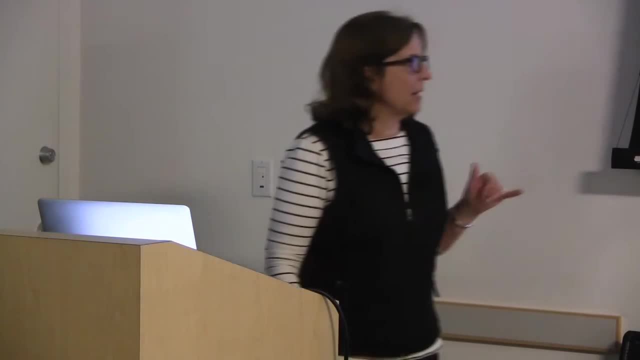 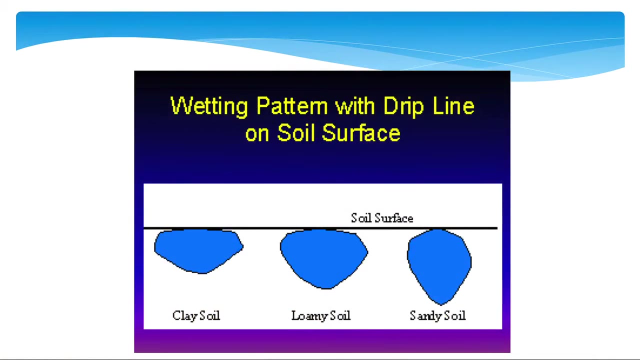 every 8 inches, every 18 inches, whatever, depending on your soil texture, your spacing should be different. So if you have a sandier soil, your water column is going to go more vertically, In other words, gravity in those larger pore spaces. 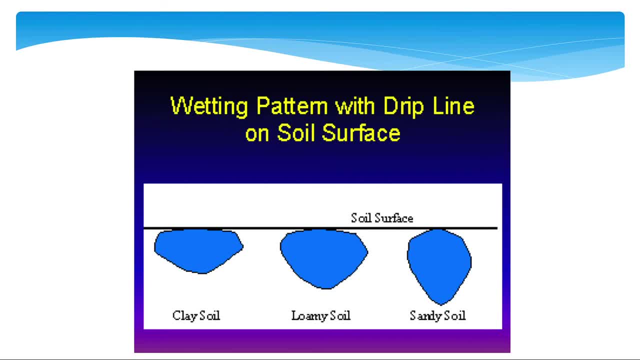 is going to be more of an influence, Whereas when you get into these soils that have a little bit more clay in them, the clay-sized particles are going to take over and those pore spaces are going to move water laterally So you can actually space. 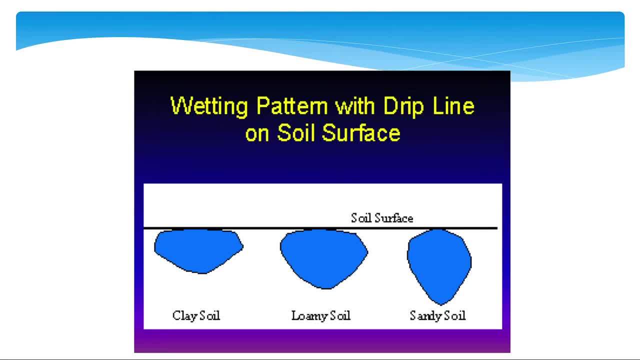 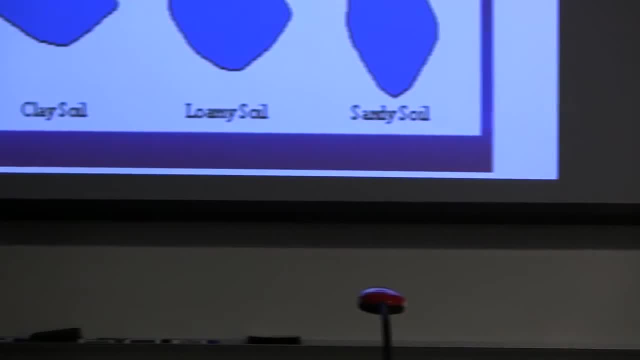 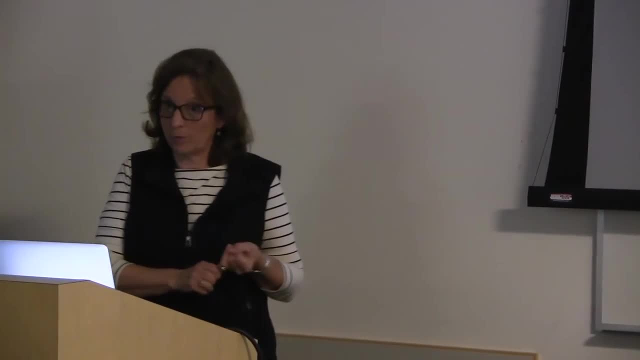 your emitters a little further apart in these types of soils and a little closer together in the sandy soil. So if you're working on irrigation systems like this, it's not one size fits all. Most of these emitter types of systems have different amounts of gallons per hour that they put out. 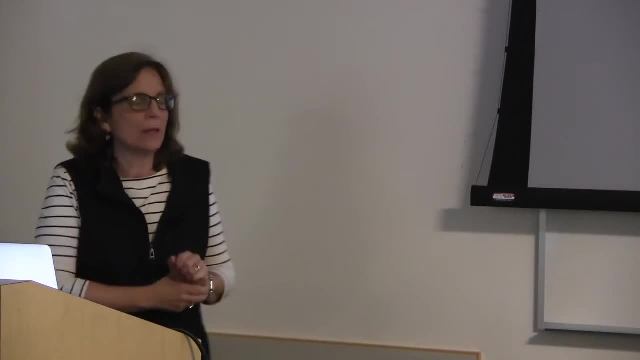 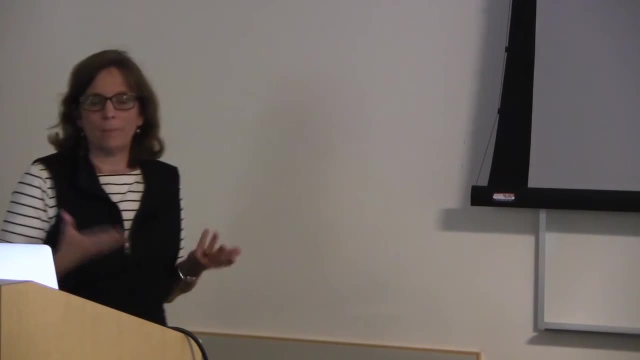 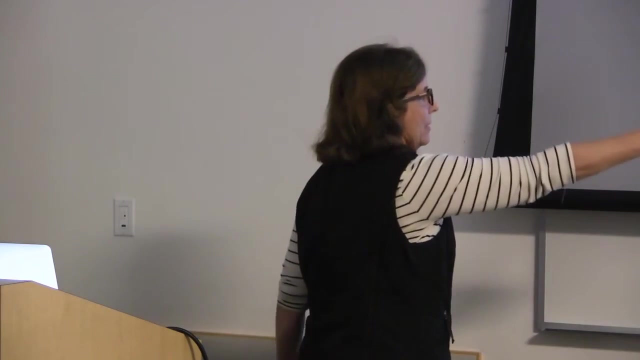 and they also have different spacing available. So there's charts and things available and I'm sure you guys are going to have an irrigation class, but you do want to correlate that with your soil type, your basic soil texture- Again, very coarse medium. 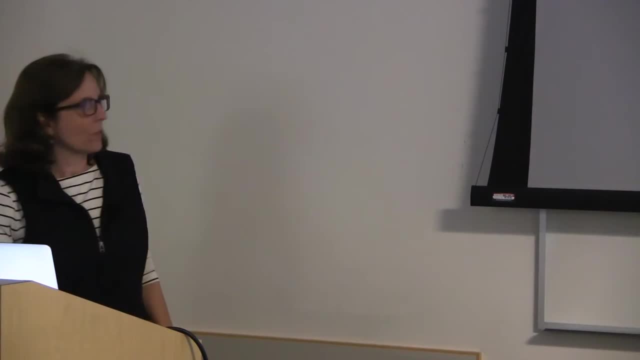 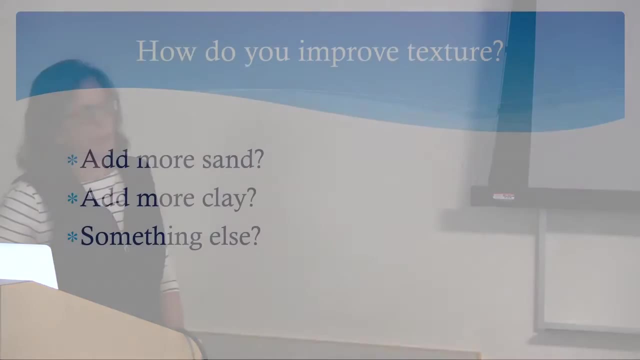 and very fine textured soil, as we call it. So that's going to influence that particular part. And again, we've kind of already talked about this: What do you do to improve the texture? Do you add sand, more clay, something else? 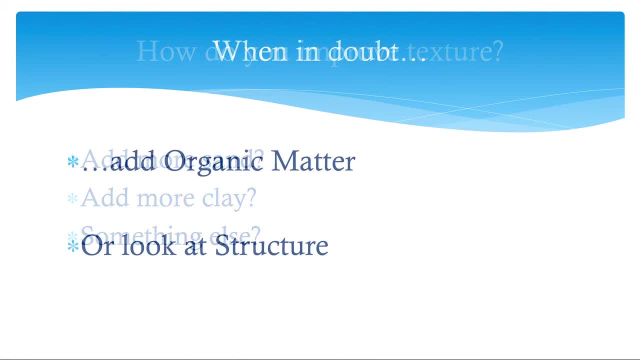 Organic matter, Yeah, organic matter. So one of these days I'm going to make a t-shirt that says: When in doubt, add organic matter. How do you determine the wilting point? How can you tell when you're at the size of the plant's wilting? because every plant wilts at a different point. How do you determine when you're in the sweet spot, so to speak? Your plants will be more productive? usually You can- actually there's soil moisture meters that you can use- and there actually are some soils- or irrigation controllers. 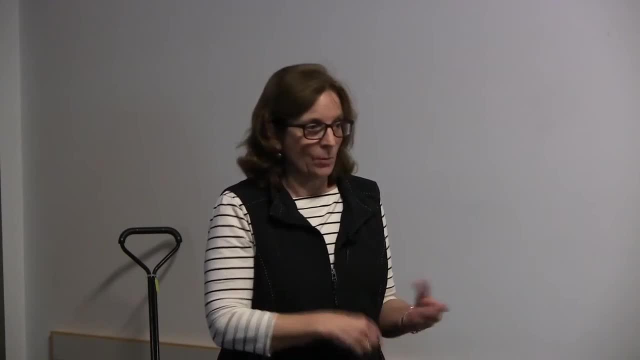 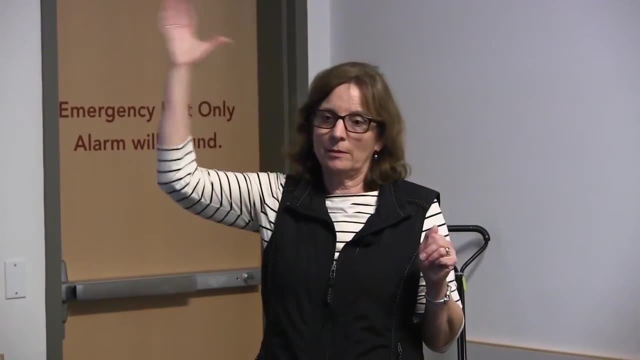 that are actually controlled by moisture in the soil. So we have smart controllers or WIVICs, that are weather-based controllers, that go on solar radiation and wind and temperature and that sort of thing to tell your, you know the ET or evapotranspiration. 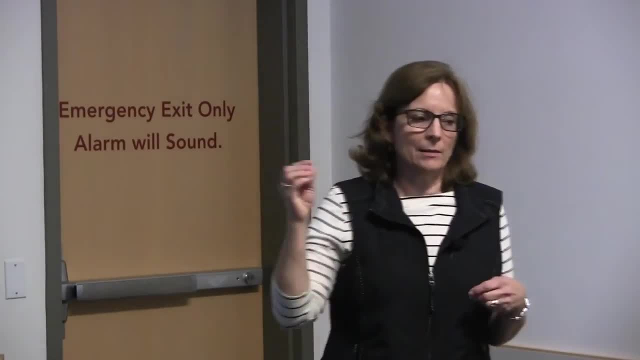 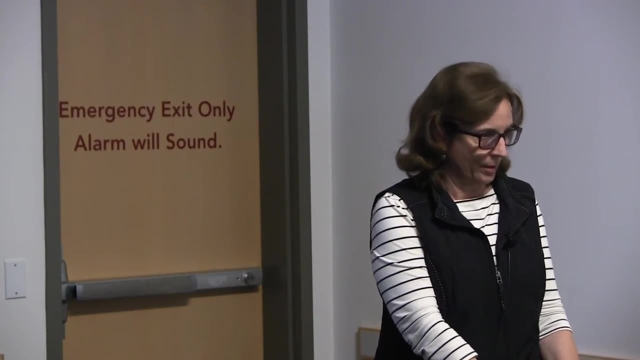 We'll probably get into all that if we haven't already. But all of that can be done and controlled by the weather, or you can control it by the soil And these little sensors in the soil. you set it, you tell it what soil texture it has and it can read it. 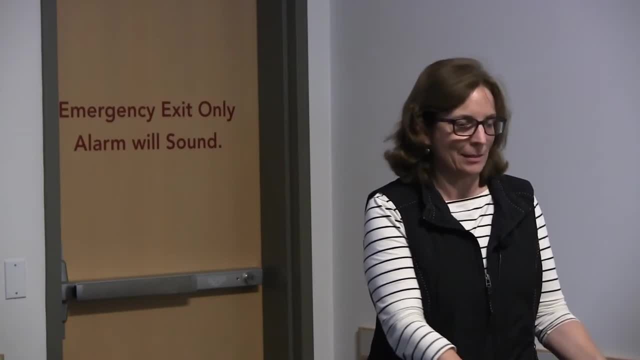 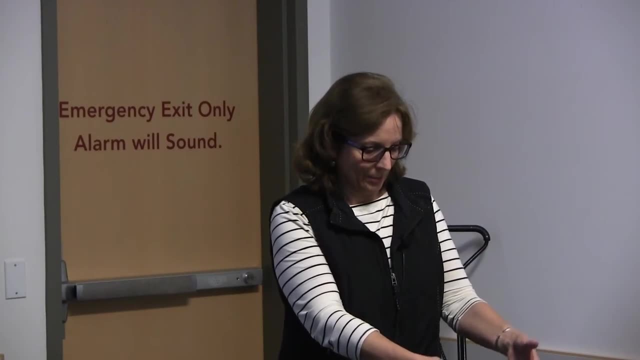 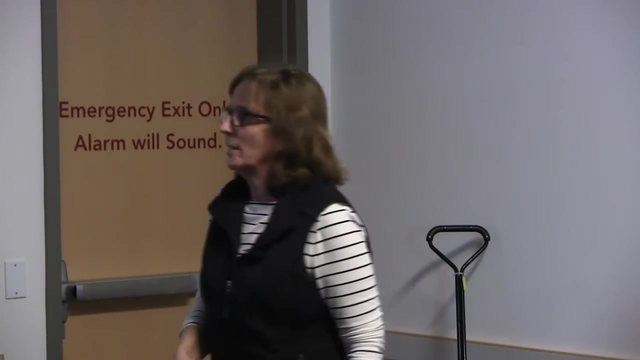 because water conducts electricity, I guess is the basic theory, and then it can adjust accordingly. So you can put one here, one here, and then this one gets to a certain point and that one gets to a certain point. Time to turn the, you know the irrigation on. 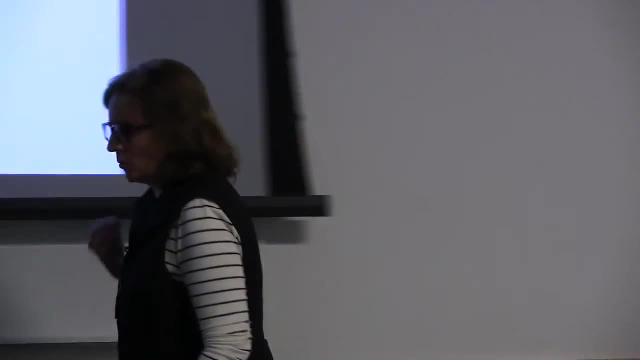 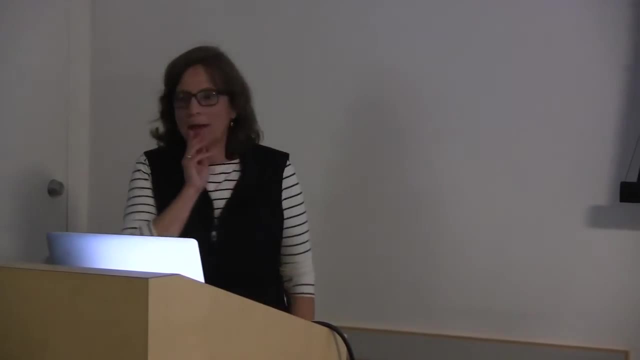 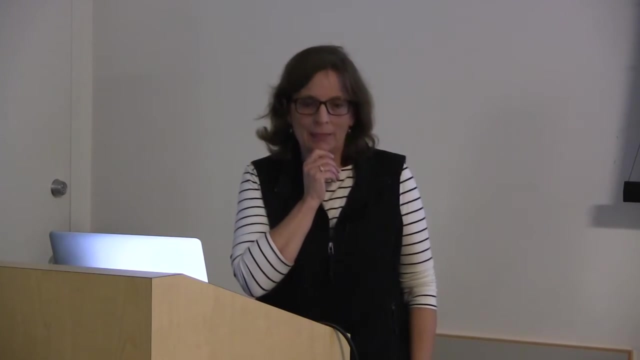 So it knows or it can sense when to do that. So soil sensing is another way to control that. Now, the other thing I also say that you can do if you have lousy texture is to look at your structure. So what we did in this jar analysis. 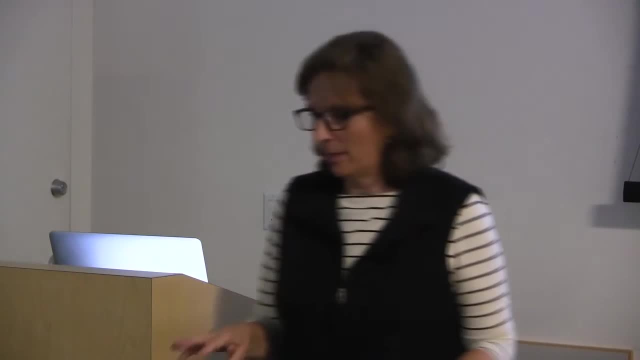 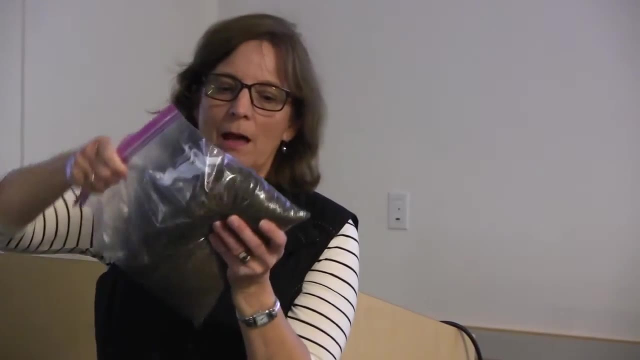 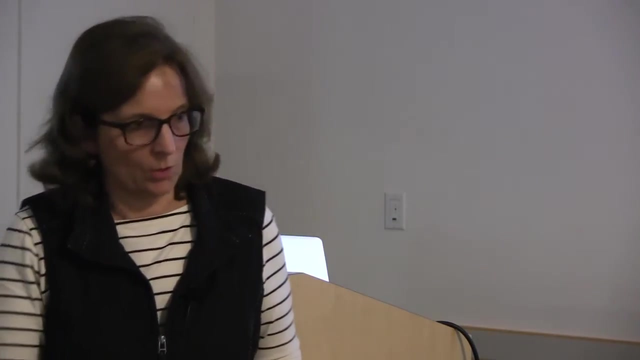 is: we destroyed the structure of the soil. This is your structure, what you have in your plastic bag. You can see clumps and clods and you know things that are visible. okay, That is not in the soil. These are individual grains of sand or individual grains. 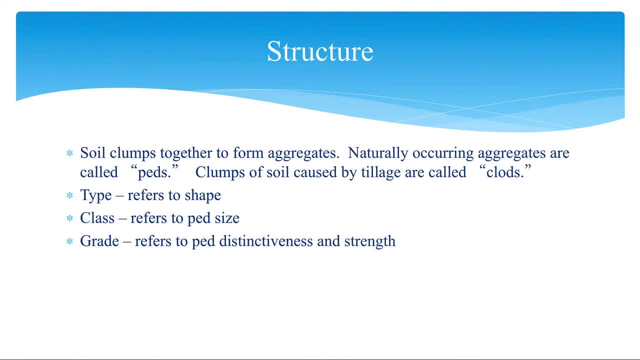 like you're seeing in your jar here that we pulverized and shook the bejeebers out of okay, So structure takes over if you should have poor texture, Does anybody have real chunky soil, Big clods or clumps? And again, sometimes it's more visible when it's drier. 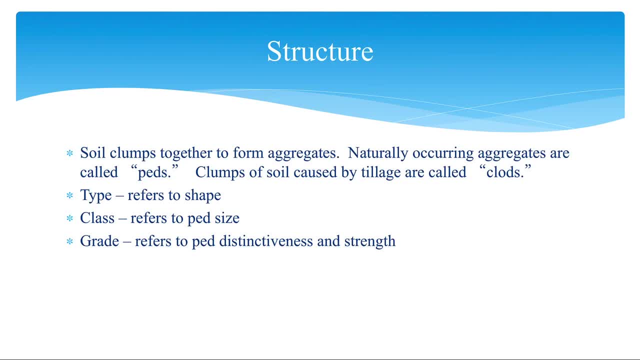 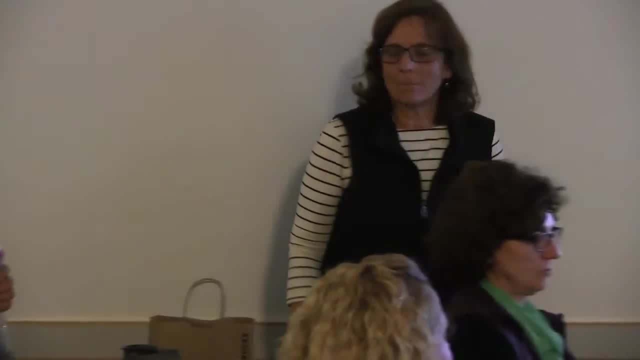 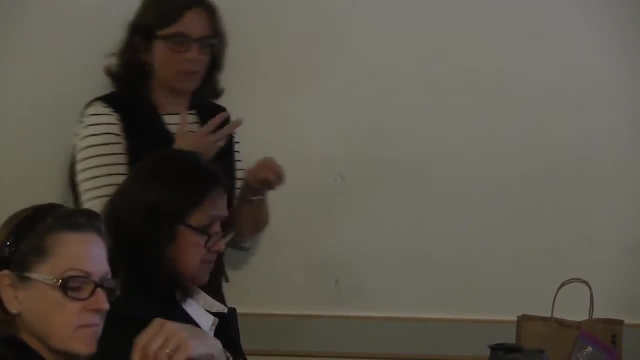 Yeah, these are kind of tending a little towards chunky, but not too bad. Very good structure in there, okay, And so that structure again provides big clods and little clods that are going to add more aeration to your soil. 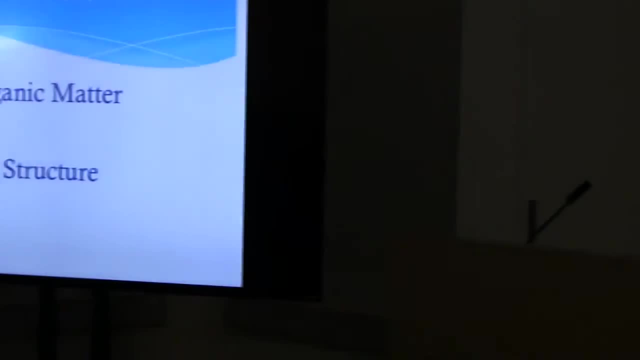 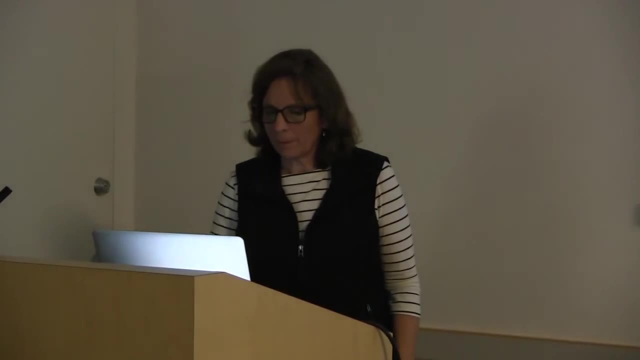 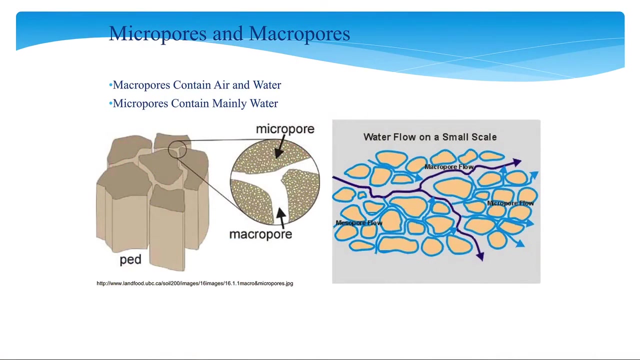 and also contribute to some of these. you know, aeration, drainage, percolation, issues that we might have. So again, we've talked about the concept of macropores and micropores. Mostly it's the macropores that are going to have the air and water. 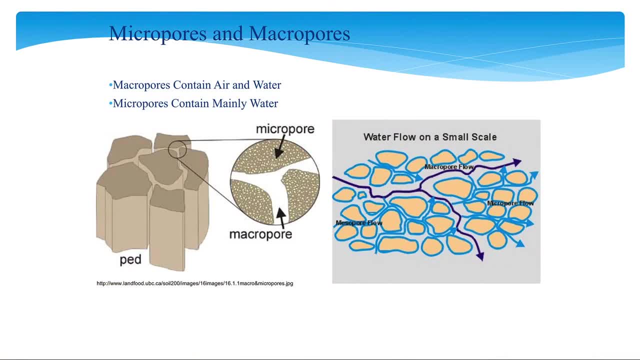 and it's the micropores that are going to have mostly water. So that kind of gets back to your question about that. So the more micropores you have, the more likely they're filled with water. But it does depend a little bit. 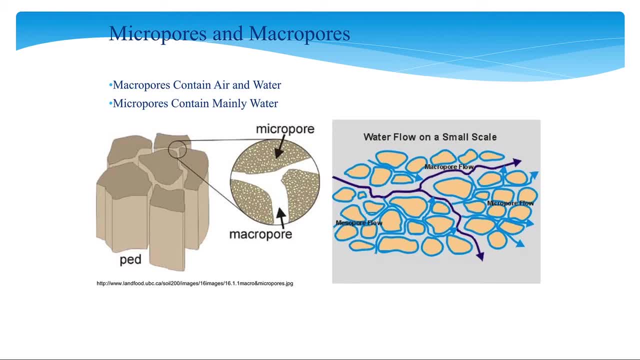 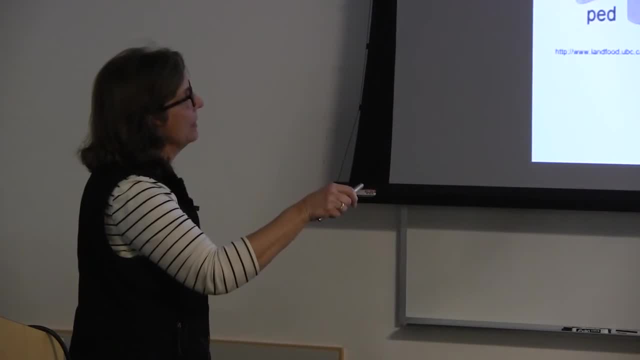 So you can see these little, teeny, tiny little spaces up there. Here's my handy-dandy pointer here. These are little tiny micropores and this is a macropore. okay, So we've got macropores here because of the structure. 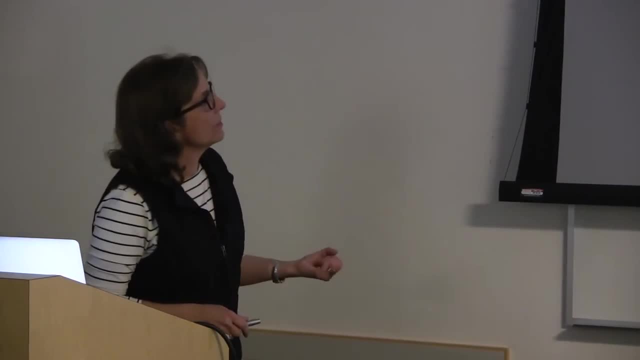 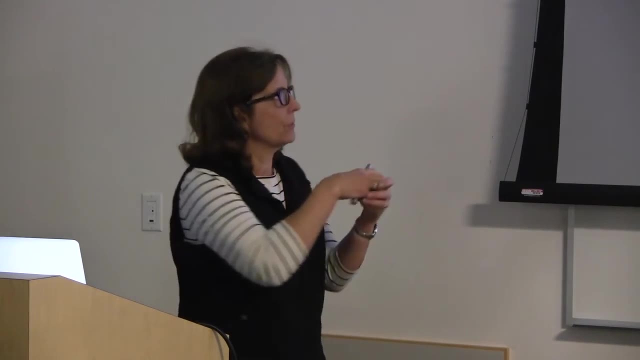 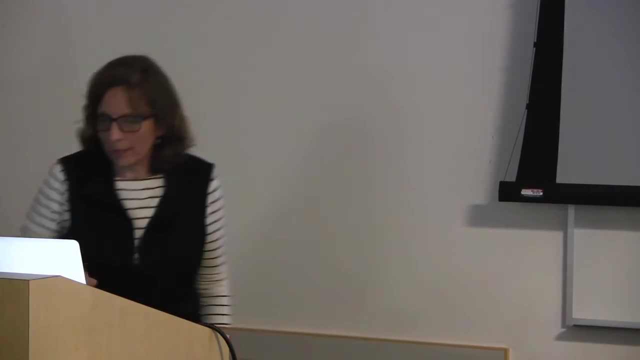 and that's going to allow some drainage through there and some aeration, whereas in the soil clod itself, those individual particles are forming what we call micropores. So water flow then on this sort of small scale is going to be happening, either with the macropores going sideways or downward. 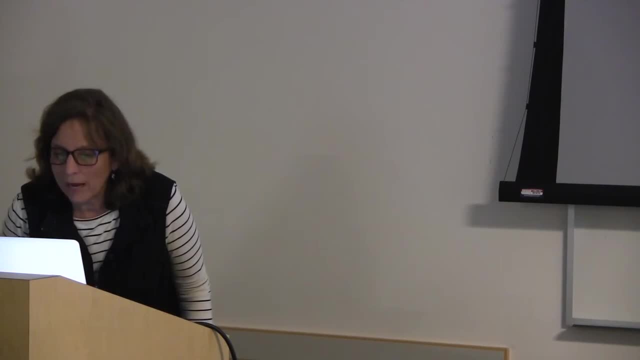 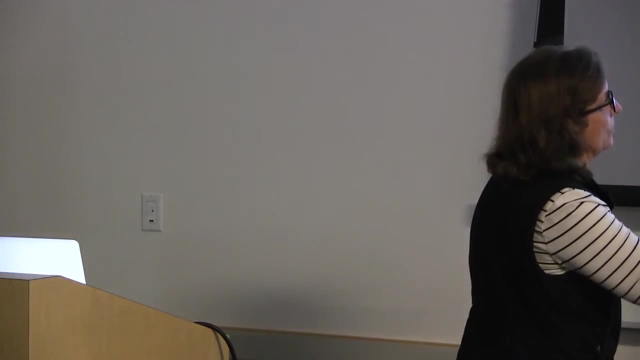 you know, or this convoluted path, and then we've got the micropore flows in between these other areas where it actually seems to be more saturated. here, where we have a lot of smaller particles, We have more water than we have air. 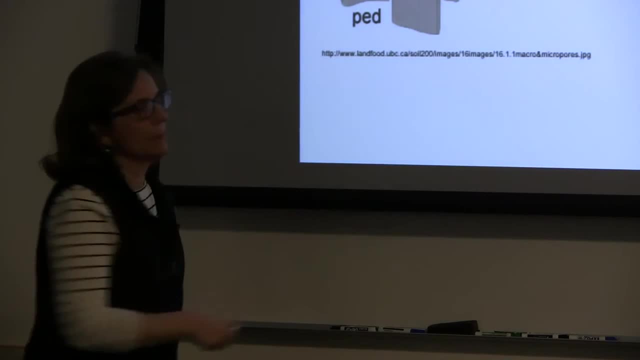 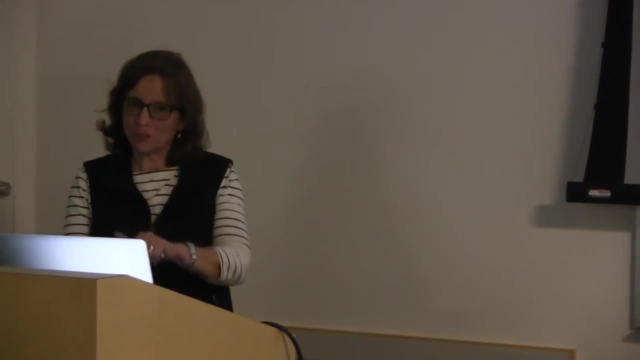 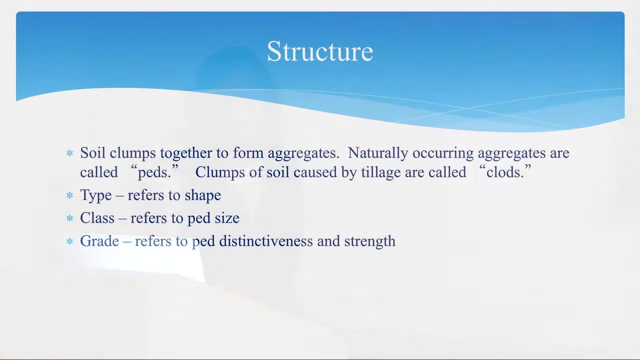 whereas between the bigger particles we've got some air flow and some water flow that's able to do that. So don't despair if your texture is bad. Your structure might actually be pretty decent. So structure is formed when the soil clumps together to form aggregates. 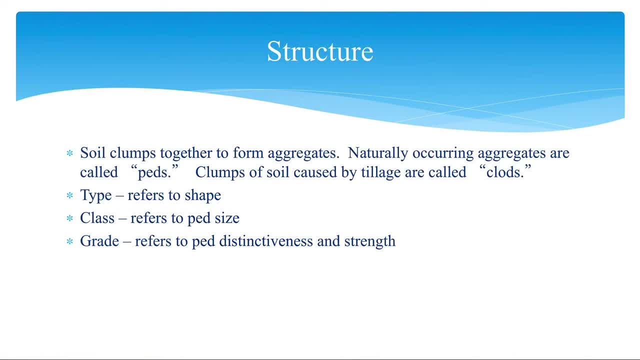 and these naturally occurring aggregates are referred to as peds and if they happen to be caused by rototilling or some sort of tilling, we refer to them as clods. So you may have seen, you know a field that's been plowed. 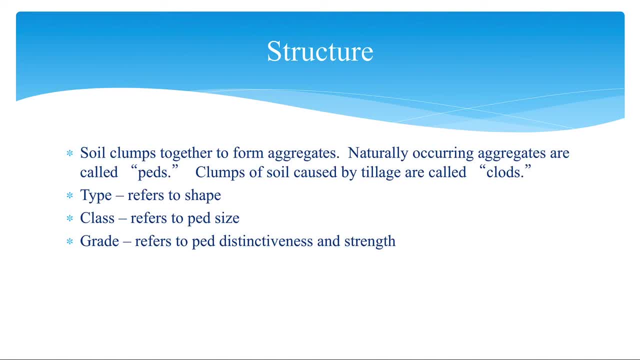 and these big clumps that form. those are going to be called clods, whereas if it's something that you have on a small scale in your bag, those are usually referred to as the peds. So there's various types, as you can imagine. 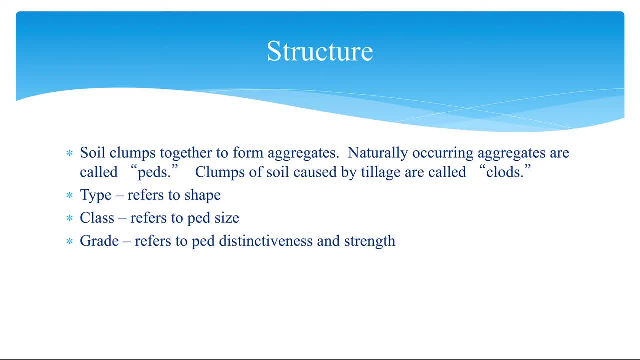 like. there's all different types of things- and this is another physical thing that we can look at and view- and there's types, classes and grades. We don't need to worry about that so much. But again, when you dig up soil, 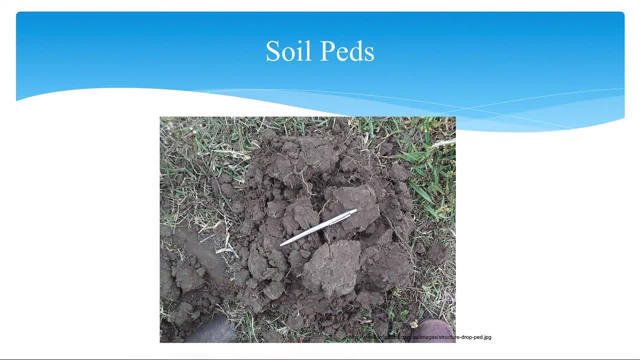 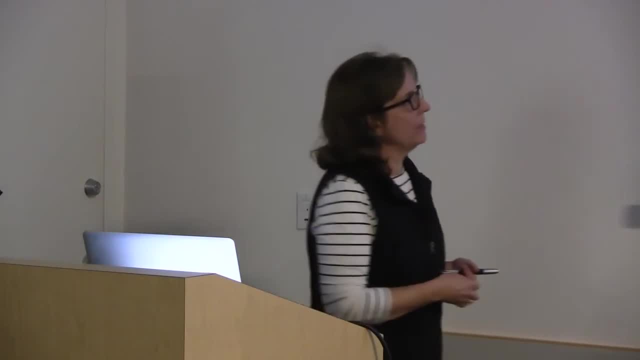 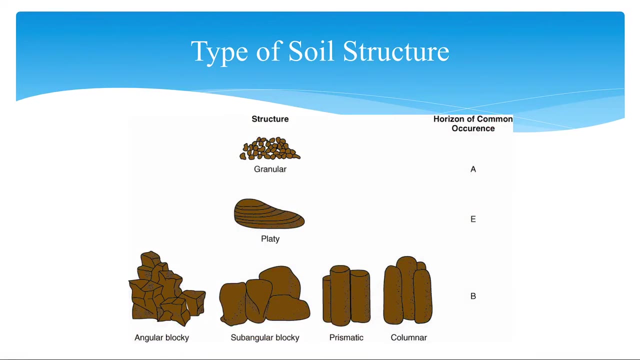 and you kind of expose it and throw it out there. it usually is in these clumps or clods here, And what they can be are what we refer to as granular. They can be platy, They can be angular, blocky, subangular, prismatic or columnar. 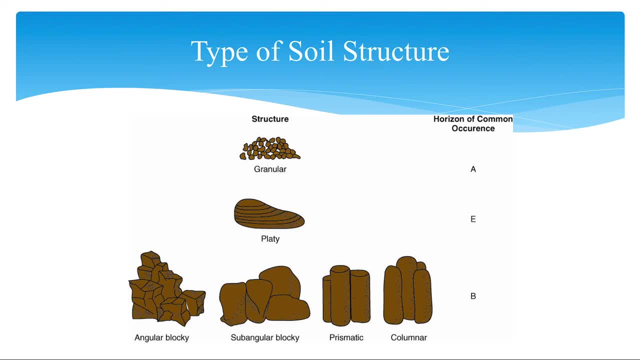 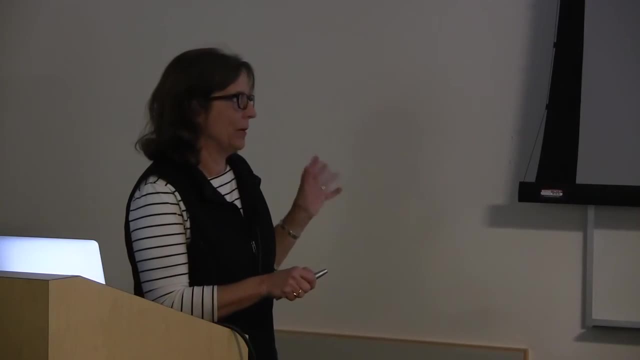 Now, this means a lot to a soil scientist And, as you can see, these occur in different parts of the soil horizon. So typically in that topsoil layer is where we have the granular, but if we have this E zone, which some people may or may not have, 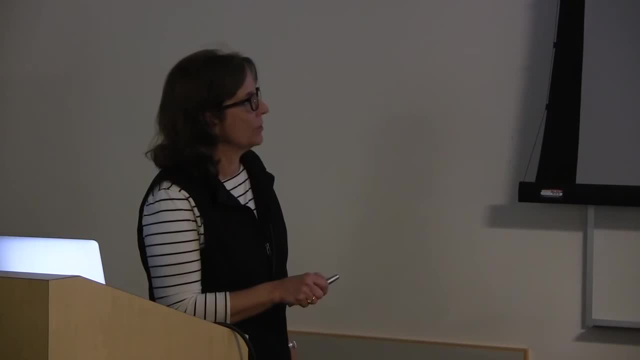 they may actually have platy types of structures that have formed. But oftentimes if you don't have that E zone you may go just A over B In the B zone down in that subsoil, the part that they leave behind after they scrape away the topsoil. this could be the type of structure that was left after the bulldozers went away. Now, the other thing they did is they probably compacted it quite a bit, which adds to the issue or the problem. It squeezes out the air. This destroys the structure. 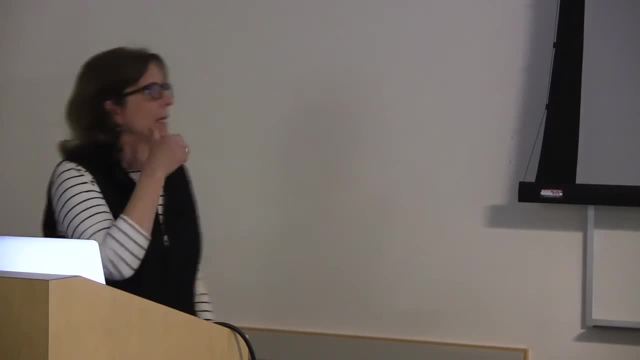 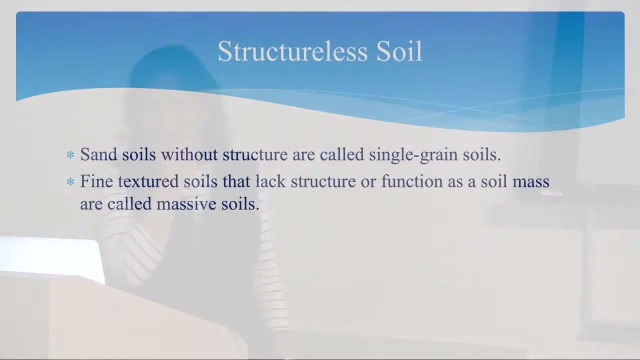 But by far probably the one you want to shoot for is the granular structure. Now we can also have what's called structureless soil. You can destroy your structure Or naturally, maybe there is no structure. So sand on the beach, No structure. 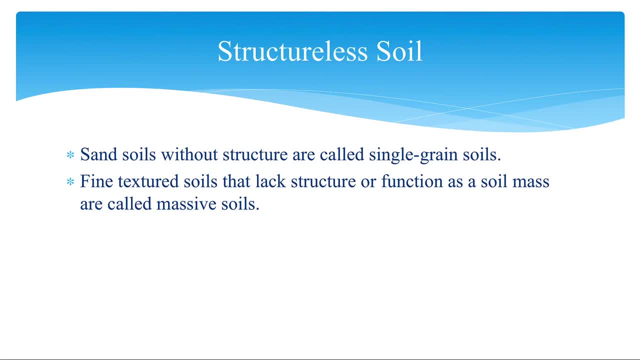 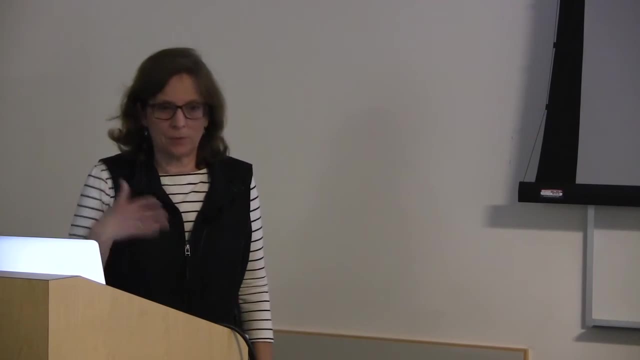 That's just grains of sand. Nothing is clumping or holding together, because it's just continually tossed and the individual grains are ebbing and flowing as the tide goes in or waves crash on it, et cetera, And so that's considered a single grain soil or in your sandbox. Fine textured soils that lack structure or function can be called massive soils, And that's sort of the opposite, but it's also a sort of structureless soil. In other words, if you have soil that you have continually, you know, run vehicles over, it's just massive. There's no air space. There's no clumps or clods or anything, It's just one big like a rock, a big monolith kind of thing. The structure has been destroyed. You can overtill your soil Rototilling too much. Need to break it to you, those that own rototillers or like to get out there and do that. You're really destroying structure sometimes when you do that, So it is something to be aware of, But the good news is you can build structure. 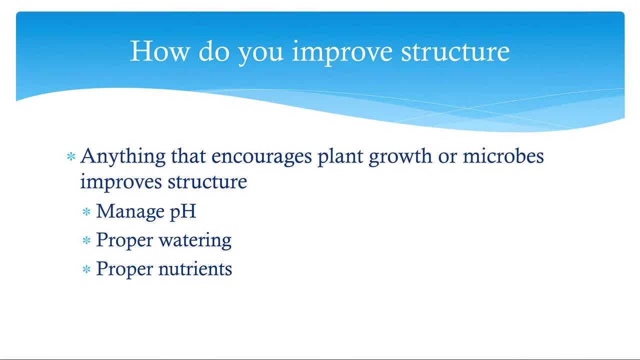 and you can encourage structure, because structure is formed by plant roots, microbes, all those little things that they give off organic matter. All of that helps to build structure And one of the things we also found that microbes are really important in building soil structure. 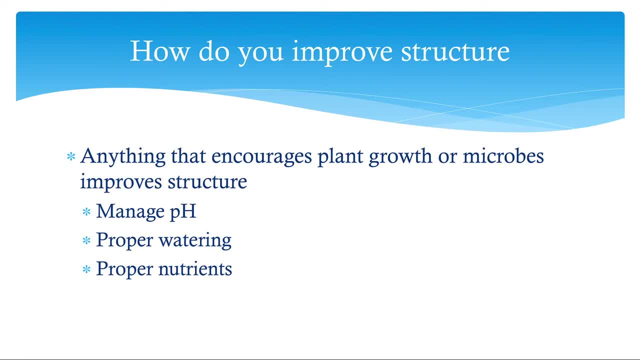 If you can keep those microbes happy, you will end up with decent structure. Microbes are living organisms. They can be fungi, bacteria, whatever. They like a certain type of pH, They like a certain amount of oxygen, typically. And if you go back to that little video of the belching, I forget his name, but anyway, the guy who was burping all the time, he didn't like oxygen methane. Yeah, he wanted that anaerobic bacteria kind of situation. Well, he's not much for structure, But other organisms are. 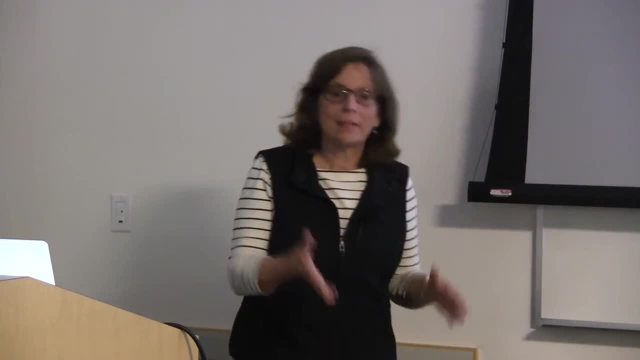 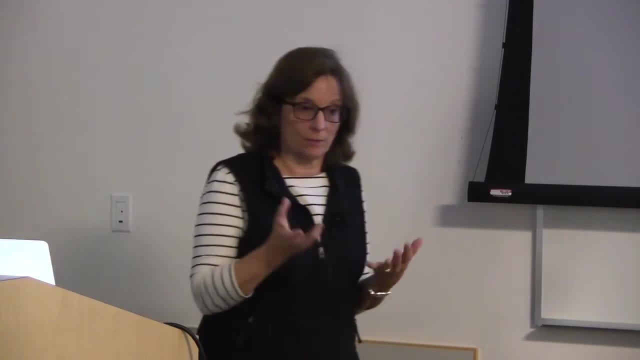 And so we've got the things that make plants happy. Typically, that's also what's going to make microbes happy. So later on this afternoon we're going to test our pH. We'll talk a little bit about chemistry and how that works. 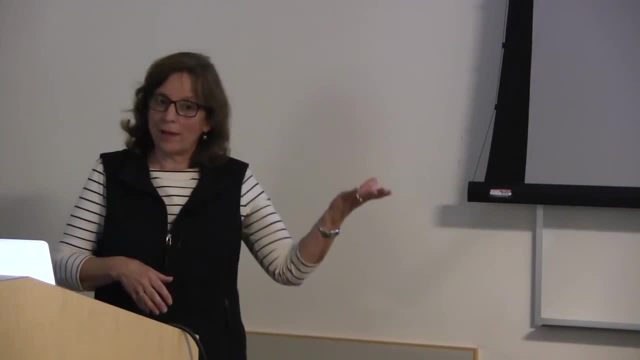 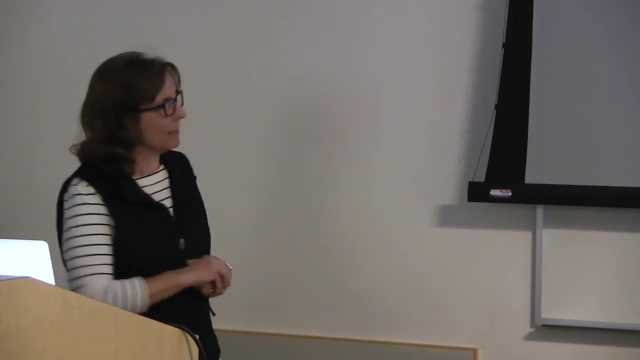 And then again proper watering, not too wet, not too dry, And then of course the proper nutrients. They like all that. A word about compaction. We face this a lot on a college campus. Students like to go from point A to point B. 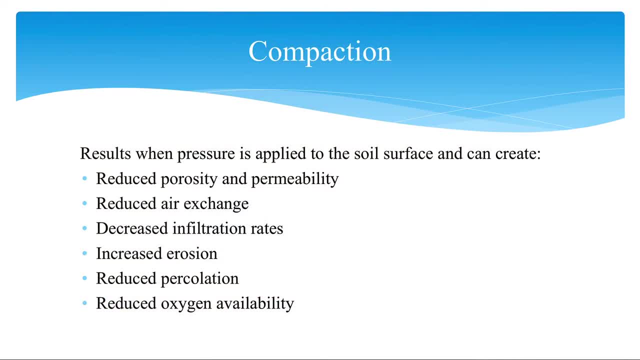 and they don't care where that sidewalk is. They want to get to that class from their car to wherever, And so they're constantly making paths, And as they do that, they're destroying structure. Okay, so nothing grows there. That's fine. 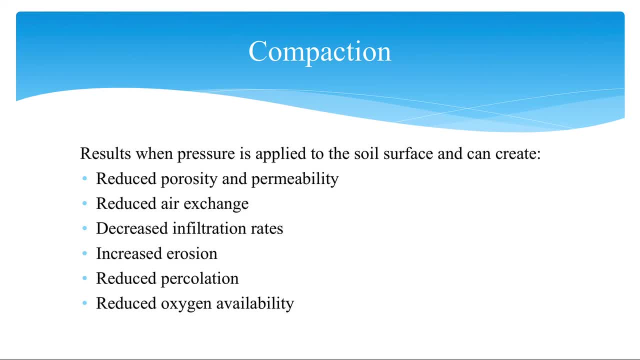 You put a sidewalk there in the first place. So human behavior sometimes can do that. But running equipment over wet soils destroys structure And when you destroy the structure you reduce the pores, that permeability, the ability of water to percolate through. 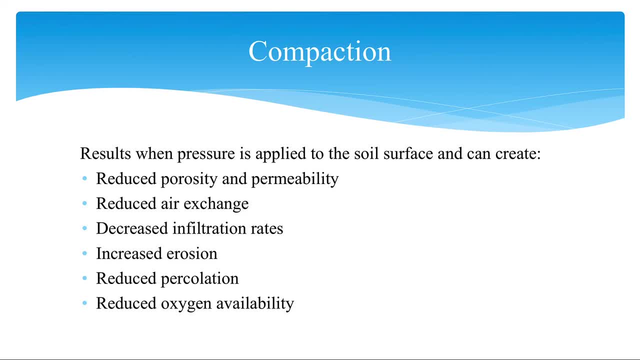 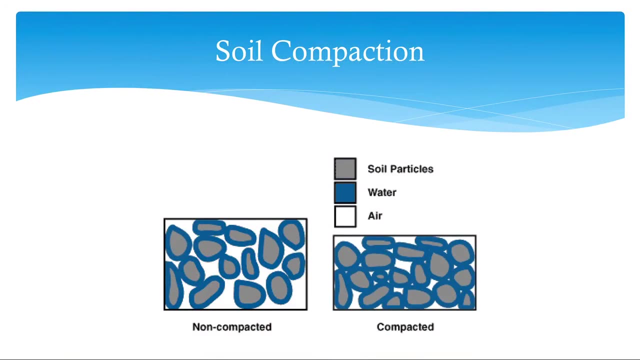 You've cut down on the air exchange, You've decreased the infiltration, You've increased erosion, reduced percolation, You've gotten rid of the oxygen. So bad things happen when you compact the soil And just kind of again showing you a more natural situation. 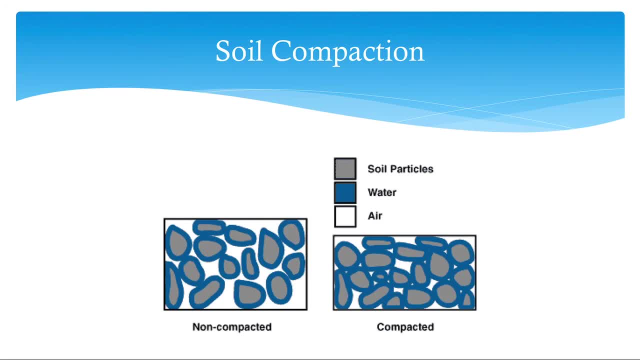 versus compacted And soil particles aren't going to change. They are what they are for the most part, But what's changing is the pore size. You're going to have more water holding capacity, less air and, again, probably not happy roots. 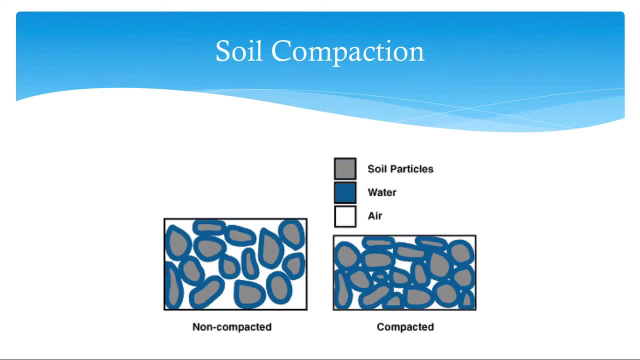 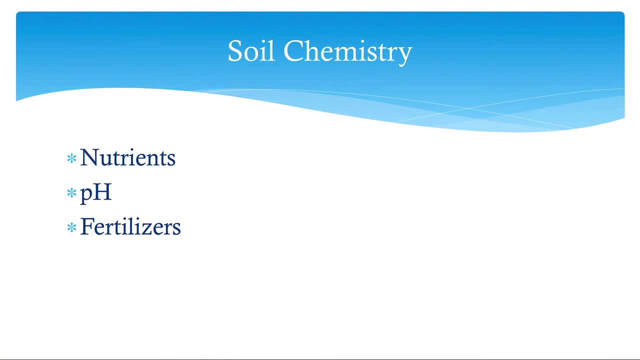 and probably not happy microbes. Okay, let's talk a little bit about chemistry, And when we talk about chemistry we're getting into fertility, okay, and things more of a chemical nature. There is a relationship to the physical and the chemical. 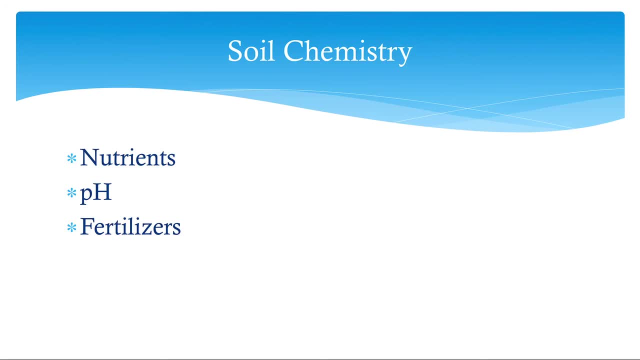 but this is almost like a different realm altogether. So we've got nutrients- NPK- Maybe you've heard of some of those- The pH, The acid alkaline, And then different types of fertilizer products. So if the soil is fertile, 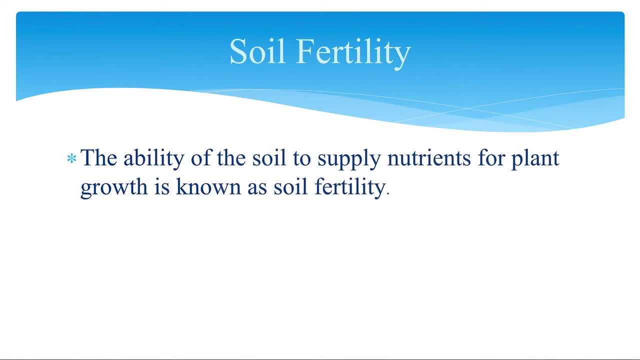 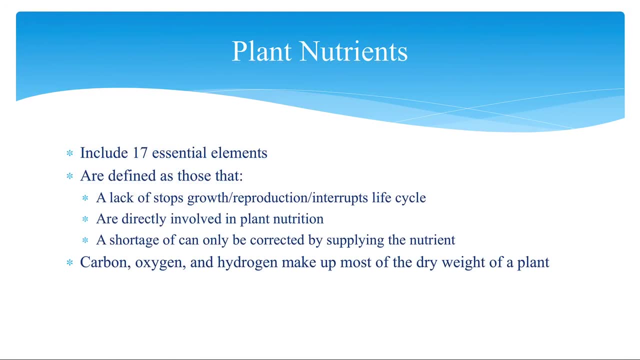 it's considered to be able to have the plant nutrients that plants require to grow And there are now considered at least to be 17 essential elements. It's depending on the plant, There can be 18, up to 20, I've heard in some cases 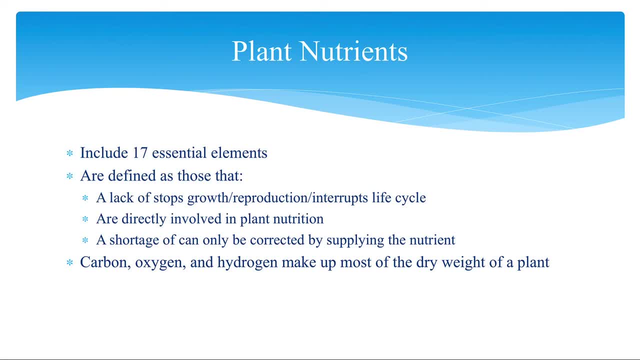 But universally across all plants In order to become essential. it means if you take one of these away, something's not going to work right with the plant growth and development And it can be just a tiny little element that's not used very much by the plant. 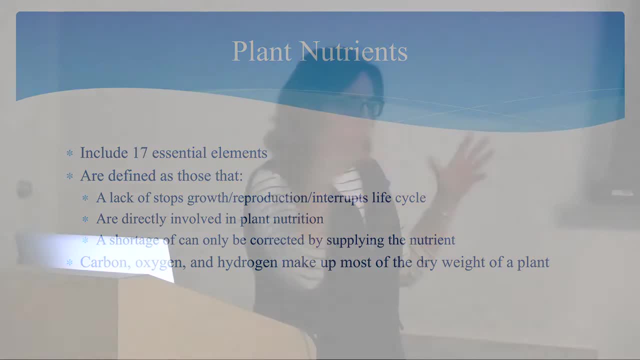 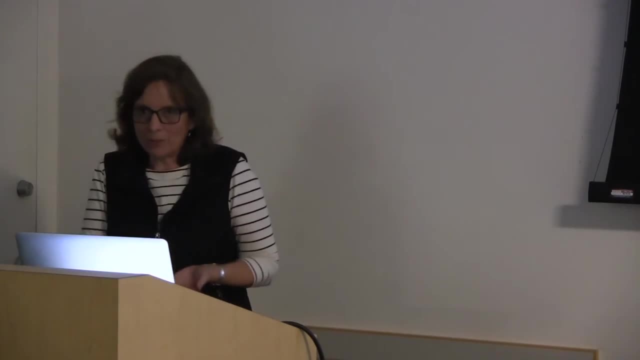 but it can have an impact on that. So it can be a teeny amount or it can be a large amount, but it can either stop a function, stop growth, stop photosynthesis, stop cell division. Something is going to go wrong if we do not have the correct mix of elements. 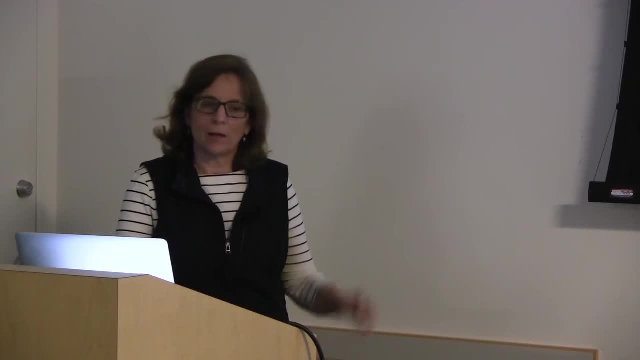 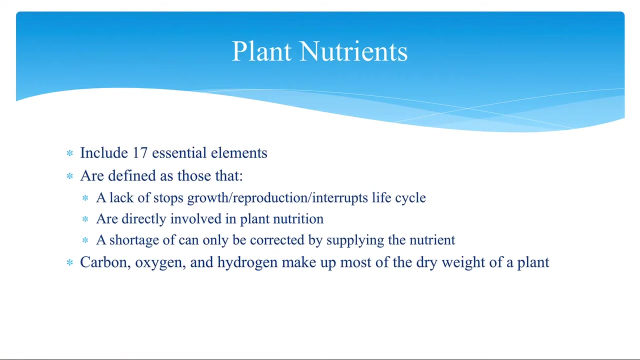 that it needs to grow These nutrients, So they're essential. If they're not there, the only way to correct it is to add that nutrient back in Now. carbon, oxygen and hydrogen are three of those 17.. These are usually naturally occurring. 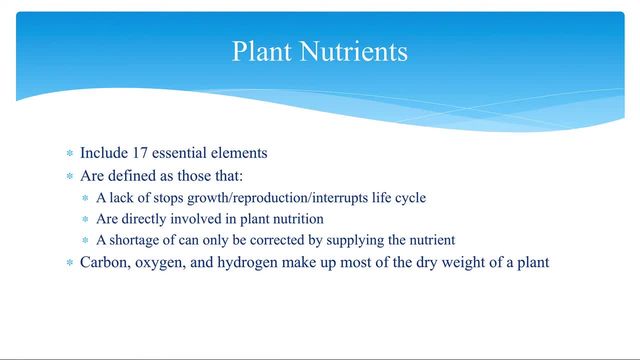 in the soil and organic matter, And those are going to be important as well. So they come from the atmosphere, from water, from organic matter. So we kind of take those for granted. It's the other 14. That we also further subdivide. 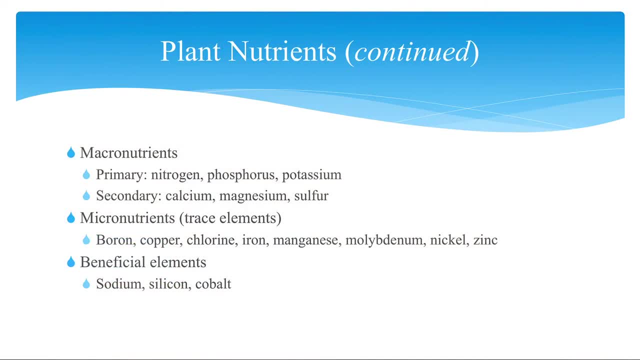 as being either a macronutrient or a micronutrient, And a macronutrient just means it's used in a large amount. Micronutrients or trace elements are used in a small amount. So the primary ones, the big three: 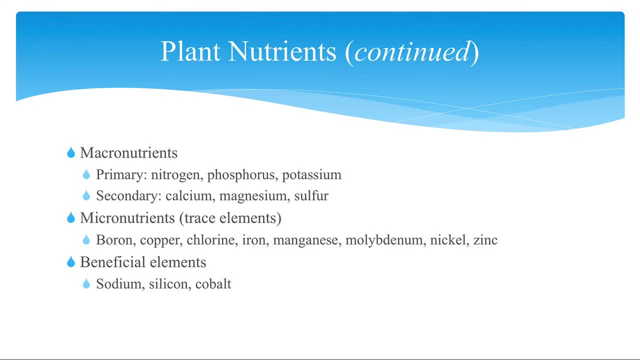 are N? P and K, nitrogen, phosphorus and potassium. Also extremely important, used in fairly large quantities, are calcium, magnesium and sulfur. Now, when we think of the N? P- K, that's usually what may be deficient in a soil. 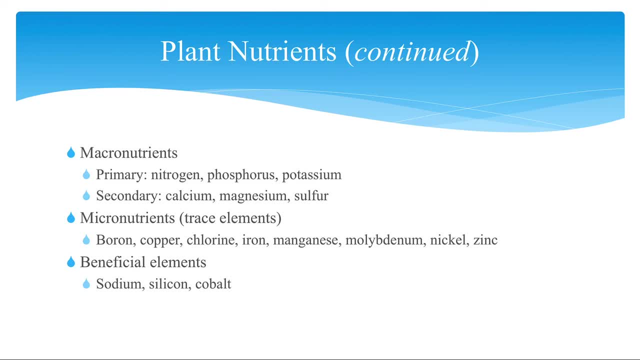 and may be. what's in a bag of fertilizer, Sometimes with some calcium, magnesium and sulfur mixed in. Read your labels and you can find out. The trace elements are used in extremely small amounts A lot of times we don't need to worry about these. 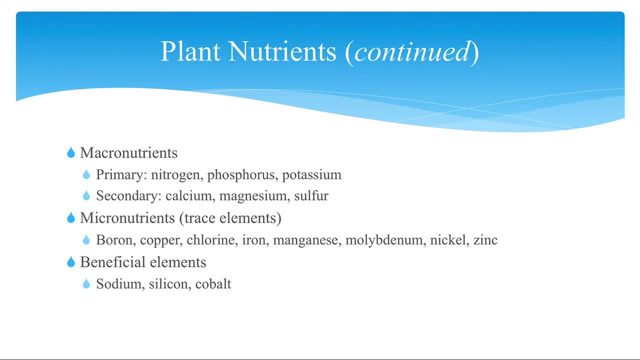 But if we are seeing symptoms of deficiency, we do want to pay attention to them. If our pH is way out of whack, sometimes, the micronutrients can also become either toxic: too much of it or not enough of it that you become deficient. 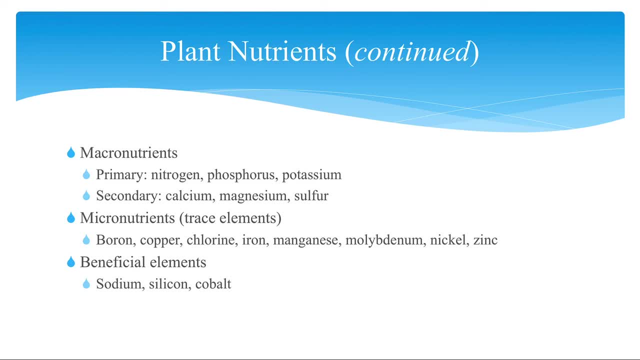 So these are your 1,, 2,, 3,, 4,, 5,, 6,, 7, 8 micronutrients, Six of them above our macro. And then the carbon hydrogen oxygen, also macronutrients, but again. they're the ones we sort of take for granted and don't usually need to worry about. Now again, in some plants, sodium, silicon and cobalt are also considered essential or beneficial, but they haven't really risen up to essential yet. 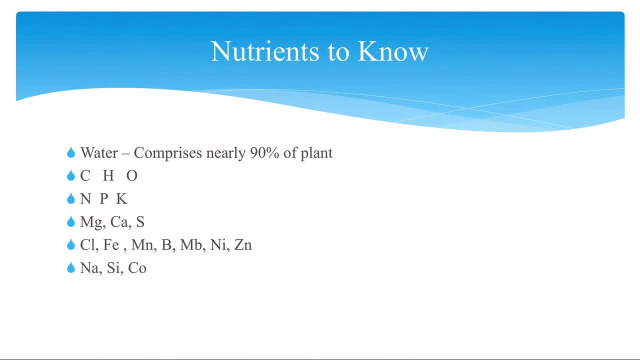 Okay, so water actually makes up 90% of the plant. Water's extremely important for plant growth and development. It keeps the plants cool, transports the nutrients and the minerals through that, and it continually is evapotranspiring from plants, So it comes in through the roots. 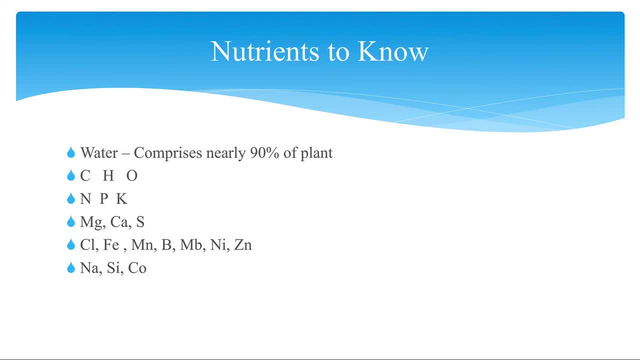 usually leaves through the leaf surface of the plant, condenses up in the atmosphere, gives us rain, et cetera, and falls back to the ground. hopefully, once we've got this sort of water cycle going on, Carbon hydrogen oxygen again. 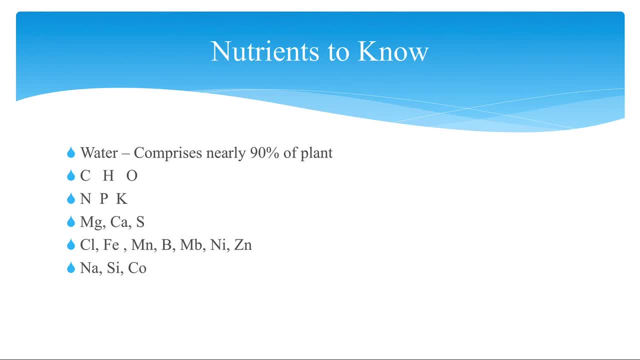 are the three that we need for photosynthesis to occur. They're extremely essential. We get them typically from water or from the atmosphere: Nitrogen, phosphorus, potassium, magnesium, calcium and sulfur, And again the micronutrients, and these last three that are important. 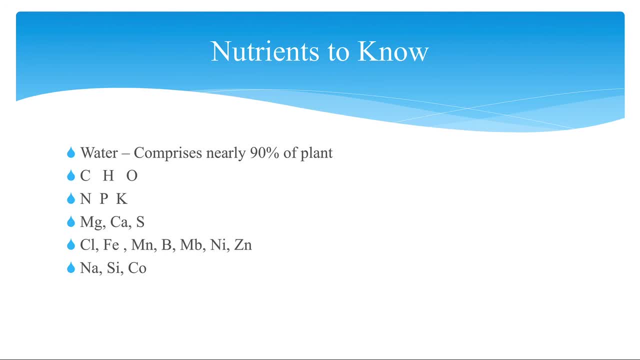 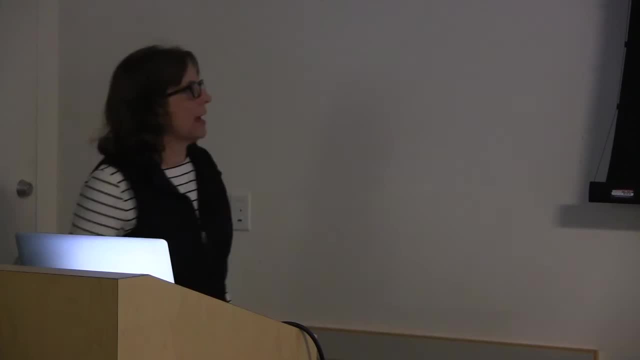 but not essential for all plants. But it's these ones up here that you kind of want to pay attention to as being a possibility of why something might not be working with your plant. Yes, I thought that chlorine was a little bit toxic for the microbes. 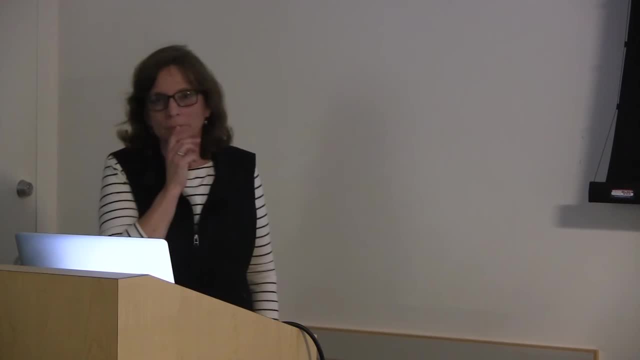 It can be. So what part of the plant chemical process requires chlorine? You know, I think we're going to get to that- There are some plants that are very sensitive to chlorine too, And so there's certain houseplants and other things that don't like a lot of it. There's some that are very sensitive to excess amounts of iron, but others that just have to have a high amount of iron, So every plant's individual. but there is I think. I have it in here and I just can't remember off the top of my head. 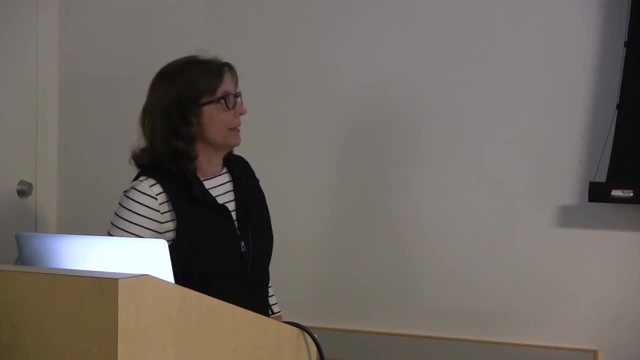 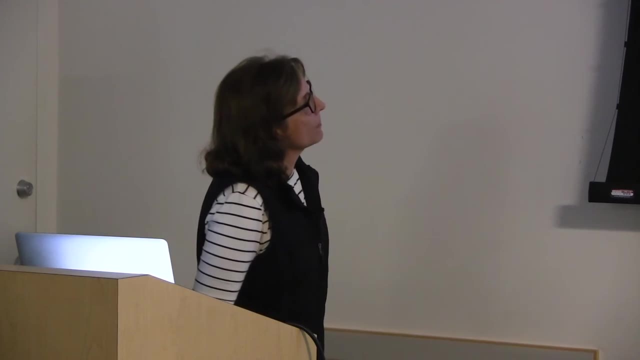 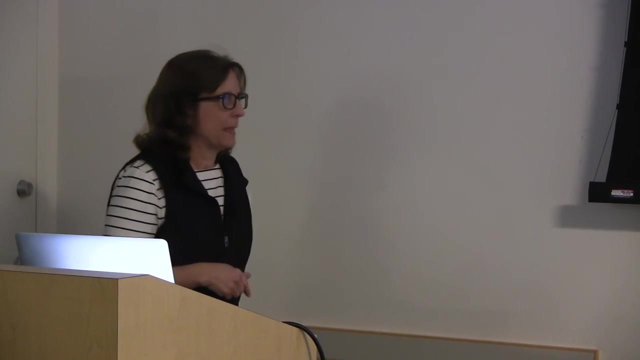 It's not a major thing, but apparently it's again probably some hormone function or something, an enzyme or something like that. Okay, So one of the other things to know about these nutrients is the plants use them in their ionic forms. They're either positive or negatively charged. When they get broken down in organic matter, you open up a bag of fertilizer and water it in whatever it's- these ionic forms of cations which are positively charged and anions which are negatively charged. 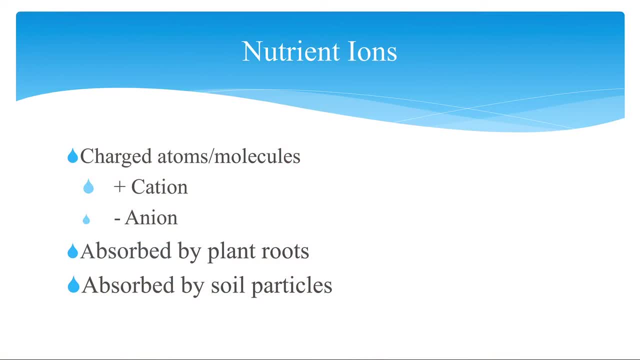 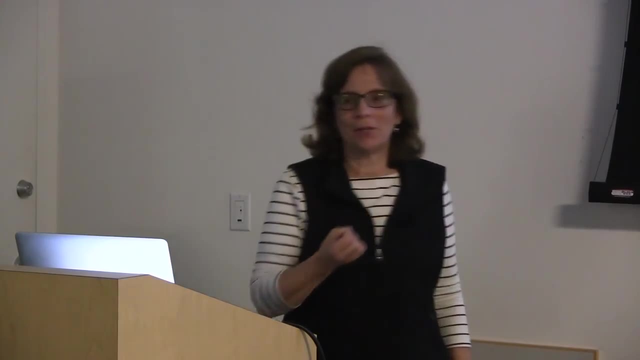 That is what is absorbed by the plant root. Again, it can be absorbed by the roots and adsorbed by soil particles, which means they can cling to these soil particles. Guess what Clay soil? lots of surface area holds lots of positively charged ions. 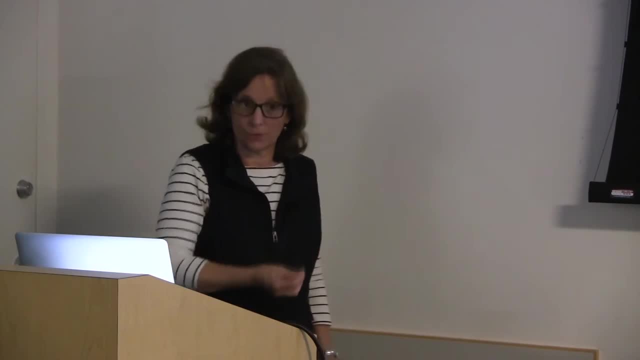 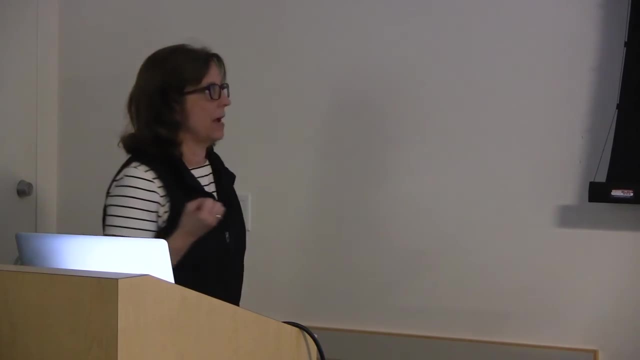 Okay. So not only does it hold water, it also holds nutrients. Organic matter is the same, Holds a high amount of positively charged ions. So organic matter and clay are actually really important in our soil for nutrient holding capacity. And again, we oftentimes look at our soil. 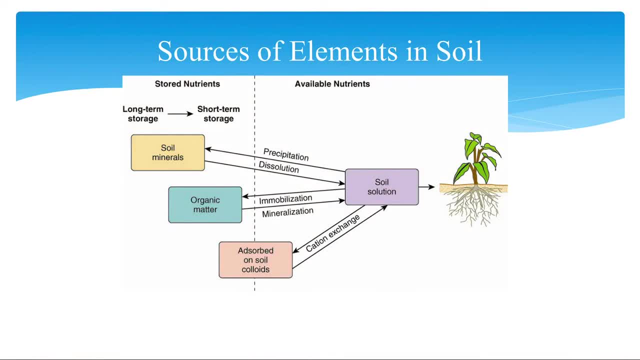 for helping us store long term Some of these minerals. they maybe even are from the parent material or they're able to hold on to them in a charged situation. Organic matter is another way we can store nutrients in the soil, And then they can also be held on the soil colloids. 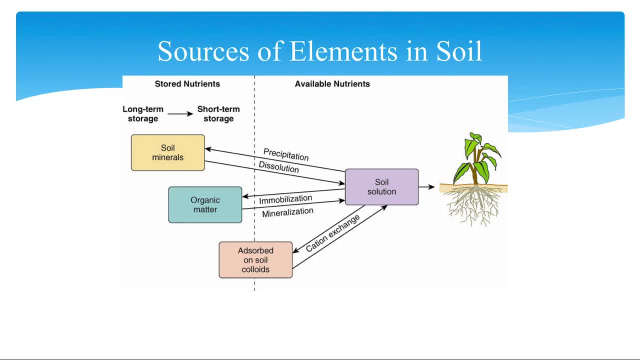 So these negative charges in the soil can hold on to positively charged ions. So this is getting into chemistry a little bit. So we have what's called cation exchange capacity. We have minerals that are part of the organic matter and minerals that are found actually. 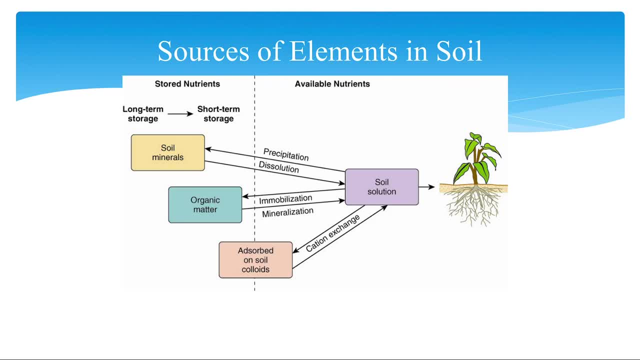 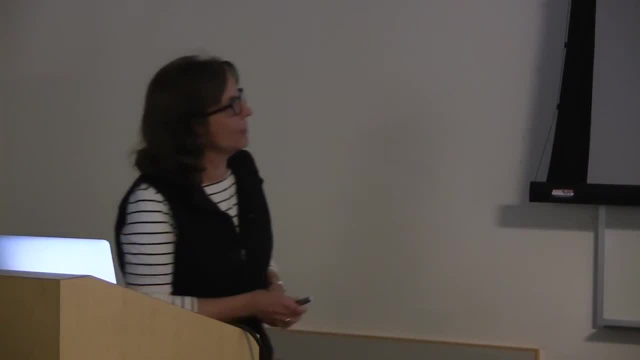 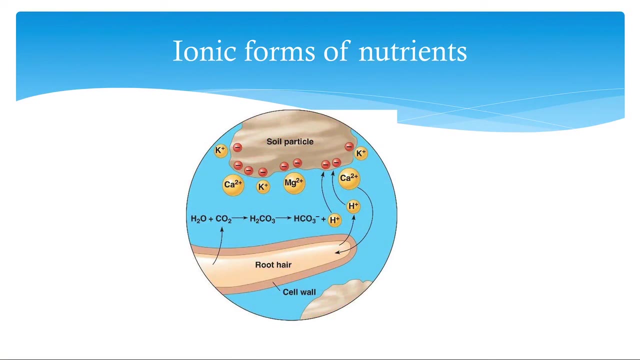 on some of these parent materials. They all get dissolved in solution and then they are taken up to the plant roots- And here's a little bit of a blow up of a root here- And it is bringing in calcium, which is a positively charged ion. 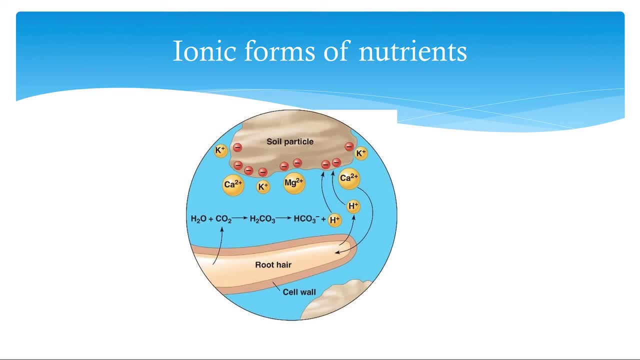 One- calcium with a double charge goes in, Hydrogen ion or two goes out And they can be held on the soil particle and just kind of waiting around until they're needed again. Magnesium, double charge: Again it's held on to the soil particle. 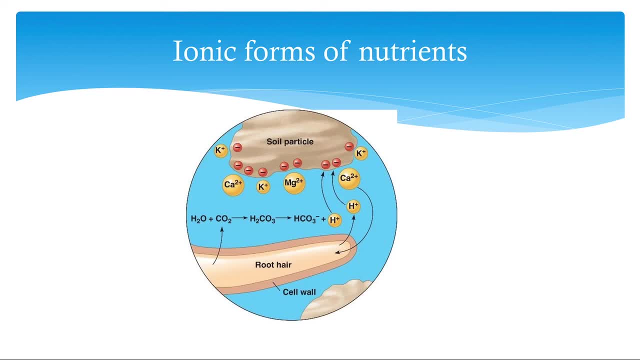 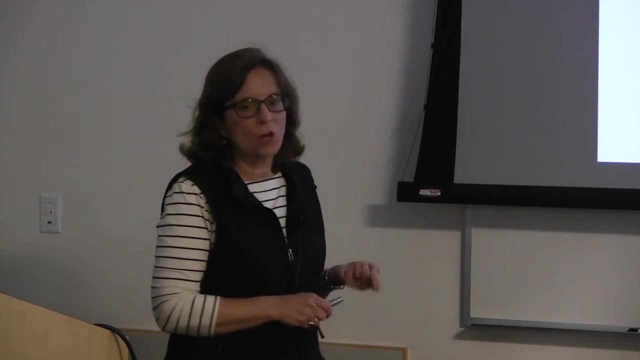 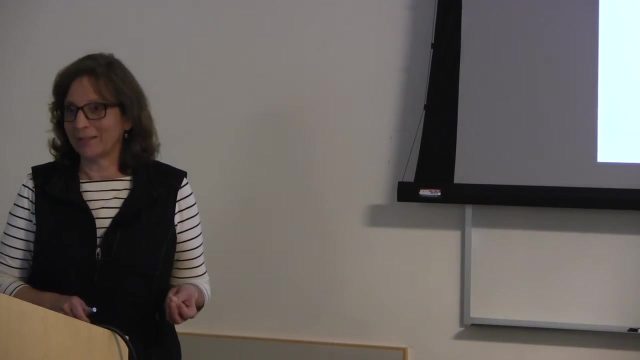 Potassium. there's another calcium, another potassium, So positively charged ions of these nutrients are held on to negative charges on the soil particles. Clay has a lot of negative charges, Organic matter has a lot of negative charges as well, And then they exchange them. 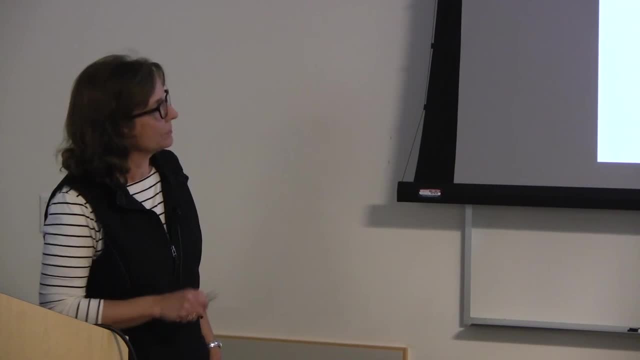 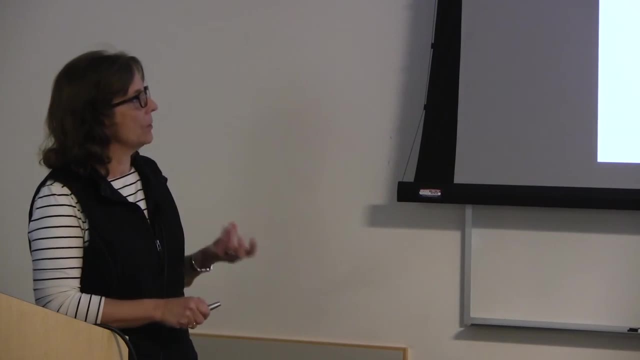 The root hair takes them in, The root hair gives them out And they can penetrate these cell walls. They're taken in in the soil solution, in the water Dissolved in that. So some comes in, some goes out, Guess what. The root doesn't care where it came from. If it came out of a bag of Scotts fertilizer, came out of your fancy chicken manure or cow or wherever. It just wants those nutrients, those ions go in and go out. So don't spend a lot of time in those sorts of things. 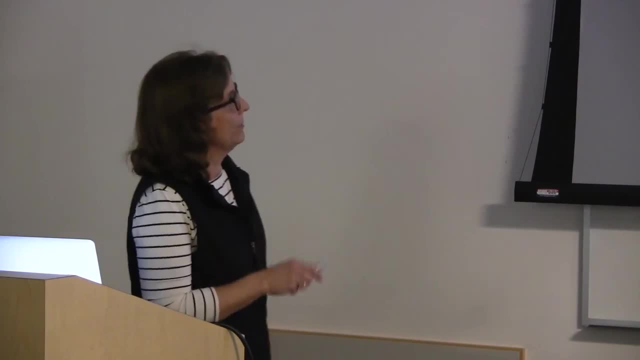 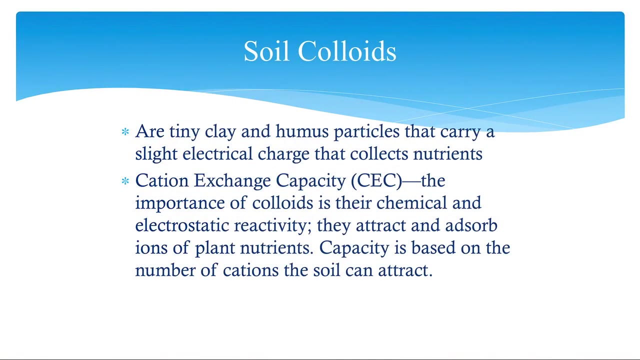 Don't worry about all your sources. Okay, I've got one minute here to kind of wrap up this a little bit, But the soil collides. here again are these tiny clay and humus particles. So if you've got a lot of that humus floating up in there, 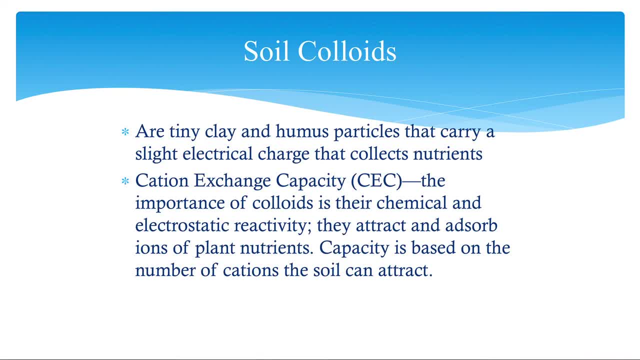 that's a good thing. They're going to be carrying an electric charge. That's why they float. That's why your clay stays suspended are these charges on it? And then they actually can hold on to these nutrients. So the more organic matter, the more clay. 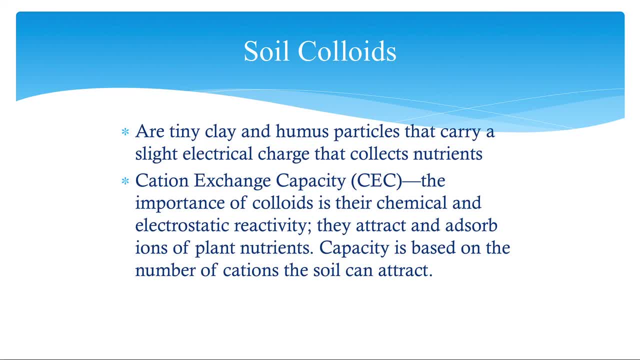 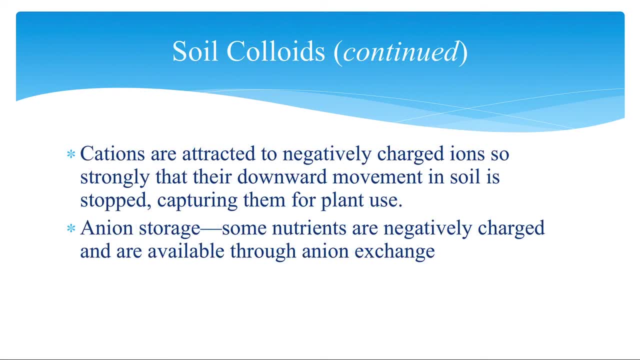 the more what we call cation exchange capacity of exchanging these cations of various nutrients in the soil. So they're positively charged, They're attracted to negative charges. Now some nutrients only come in the anion form or the negative form, So they're not always held in this situation. 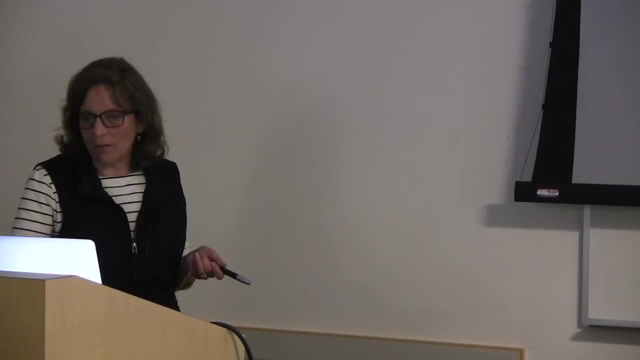 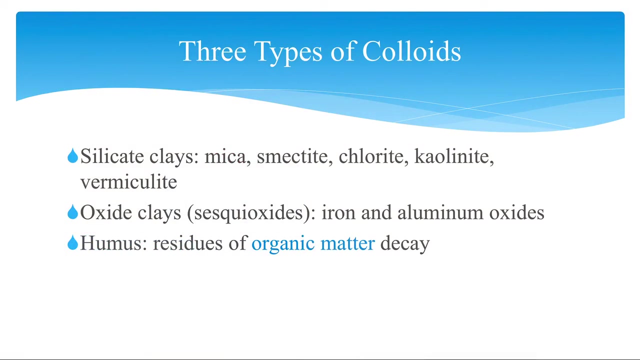 And they're the ones that tend to leach a lot. So different types of clays all have different properties. So whether you're coming from mica, smectite, kaolinite, vermiculite or oxide clays, you know. 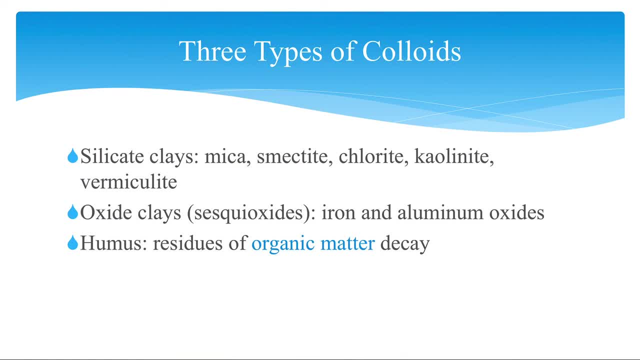 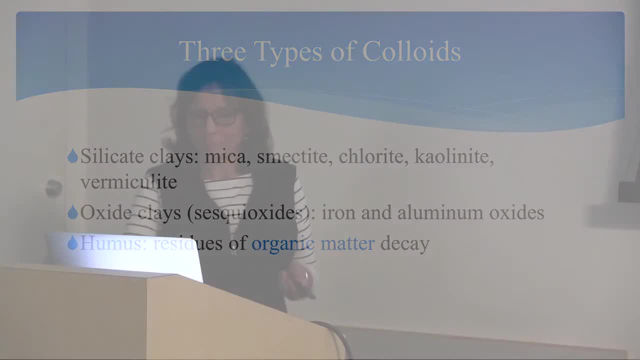 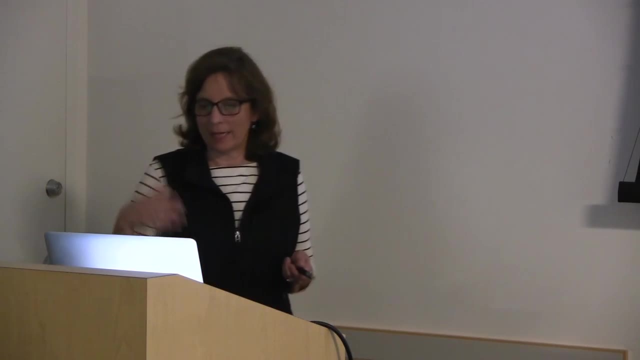 these are just all different types of clay, minerals Or organic matter. depending on that crystalline structure, you can store more or less amounts. So soil is the source of most nutrients, except nitrogen. Usually we have to add that, or it comes from organic matter.